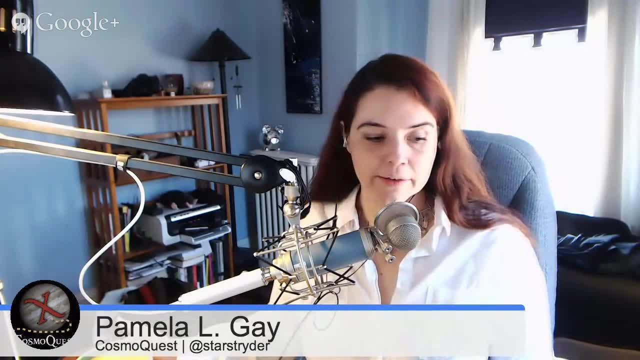 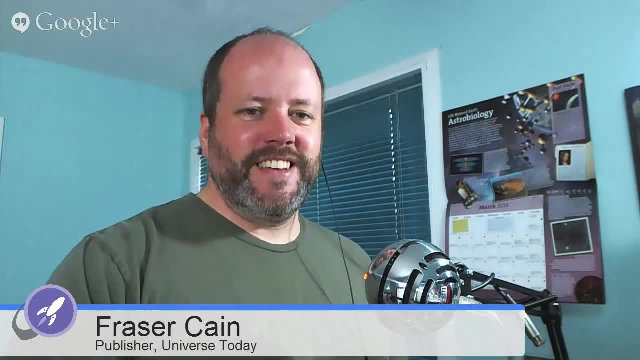 Yeah, I took my horse outside on Saturday and he looked at the ground and nosed the dead grass and asked to go back in the barn. This sucks, Yeah, All right. well, let's get rocking, Let's get into this episode. 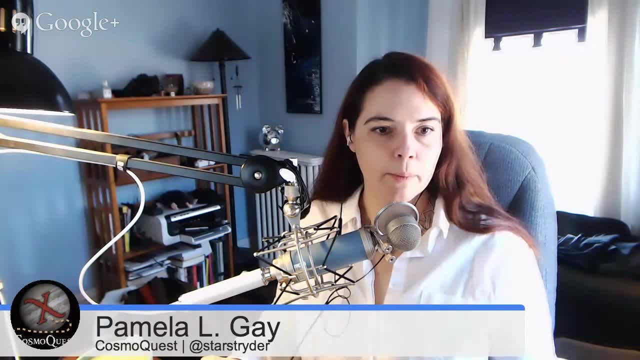 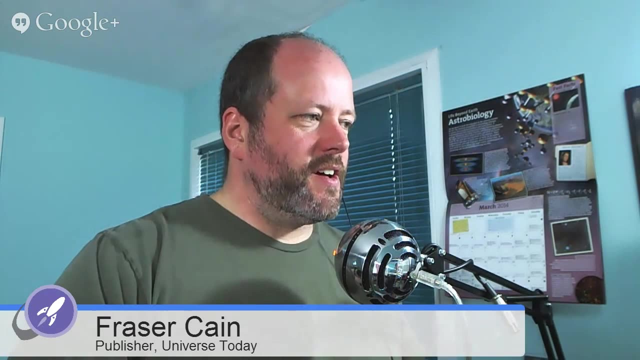 Okay, So are you ready to press record? I'm about to be. Yeah, I am Pressing record, Testing, testing. Okay, Hi, Preston, Everything's working. Hello Preston, Once again, we thank you for your service. 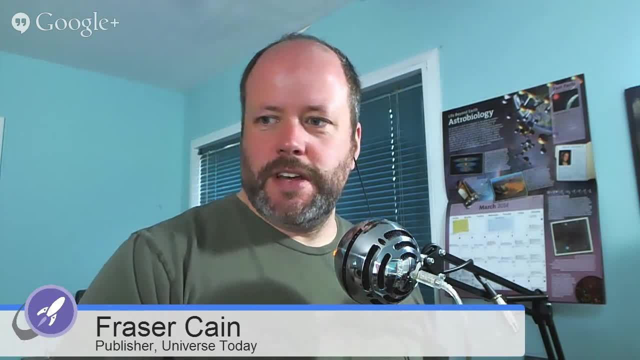 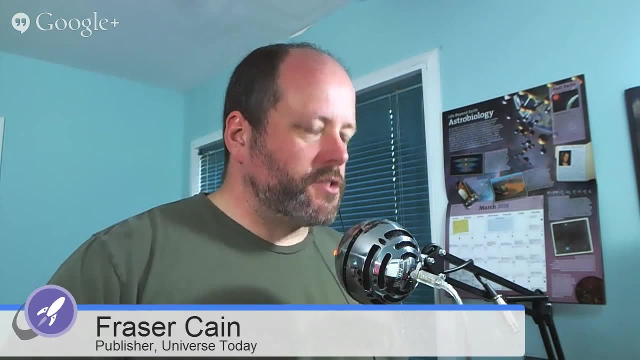 We're now about to bring you the latest episode of Astronomy Cast. Okay, Got my intro. Astronomy Cast, episode 337, photometry. Welcome to Astronomy Cast, our weekly facts-based journey through the cosmos. We'll help you understand not only what we know, but how we know what we know. 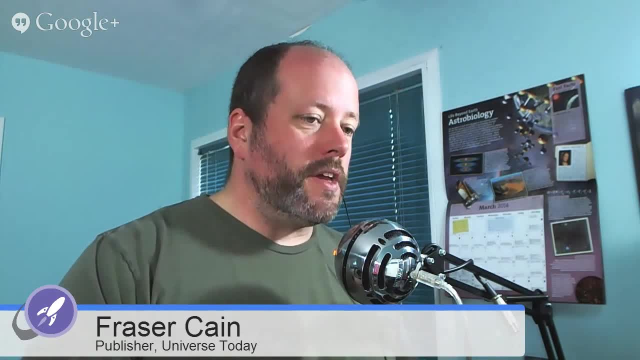 My name is Fraser Cain, I'm the publisher of Universe Today, and with me is Dr Pamela Gay, a professor at Southern Illinois University, Edwardsville, and the director of CosmoQuest. Hey, Pamela, how you doing. I'm doing much better this week and I have to apologize for last week. 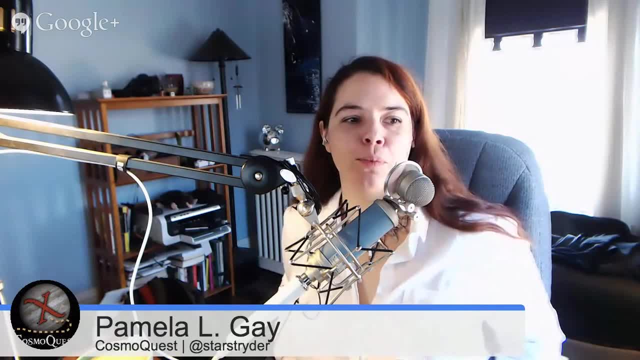 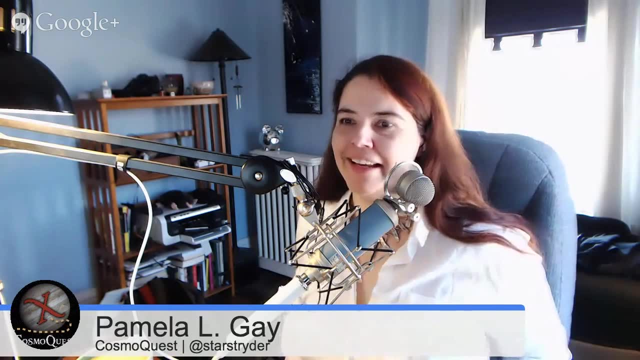 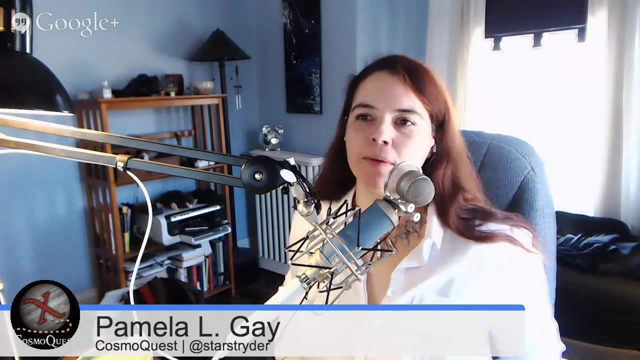 We recorded and I was really stubborn and determining not to admit how really damn sick I was. and The next day I got diagnosis of pneumonia and scolding and Yeah. so if last week's episode, the episode on units, was not the best-ever episode we've ever produced, 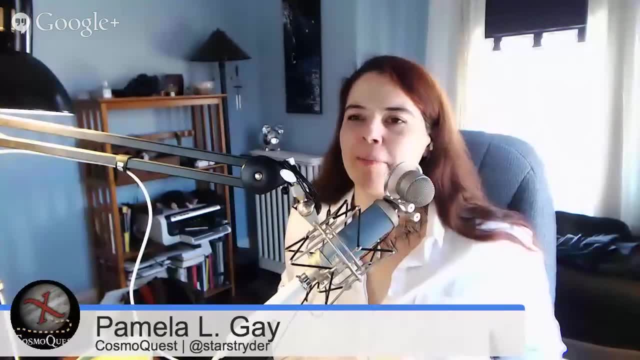 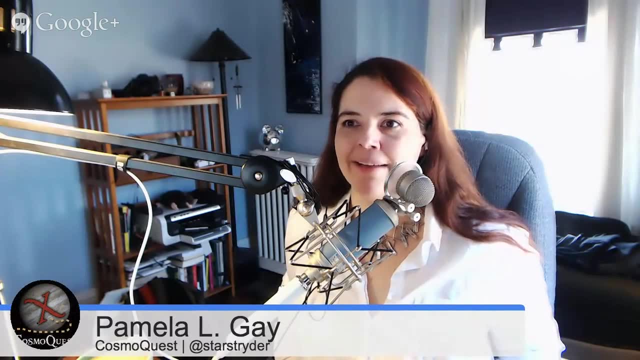 For once, we can blame you. It's totally my fault, Totally my fault. Dayquil, Nyquil were not enough to get the neurons firing at full capacity. I'm better now. Good, Not 100%, Yeah, you do. 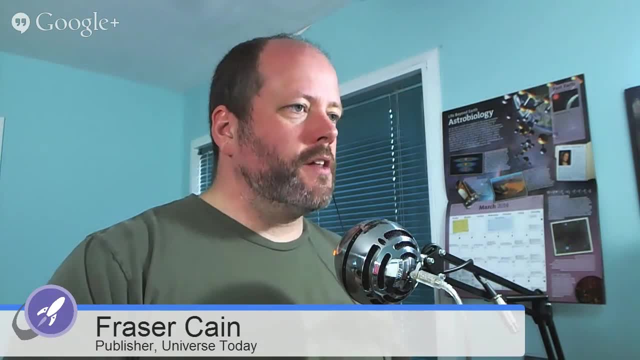 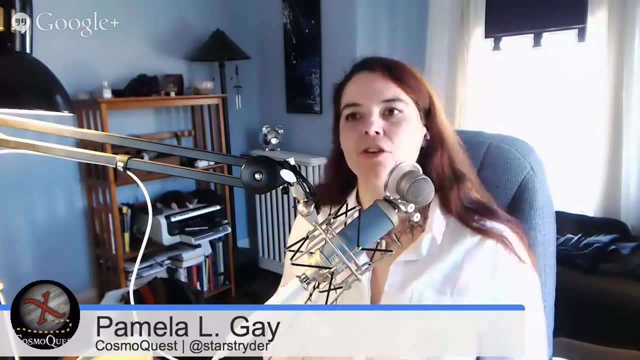 You look like you're well into your recovery. so, Yes, Yes, I'm at the getting the energy backstage instead of getting the oxygen backstage. All right, let's get on with the show. So there's a lot you can learn by just staring at an object, watching how it changes in brightness. 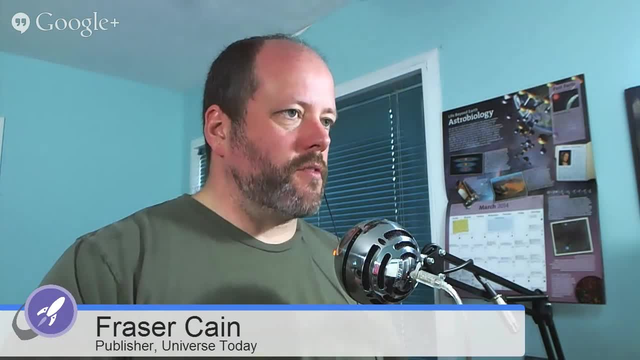 This is the technique of photometry and it has helped astronomers discover variable stars, extrasolar planets, minor planets, supernovae and much more, And this episode is going to come straight from your head because you are a variable star astronomer. 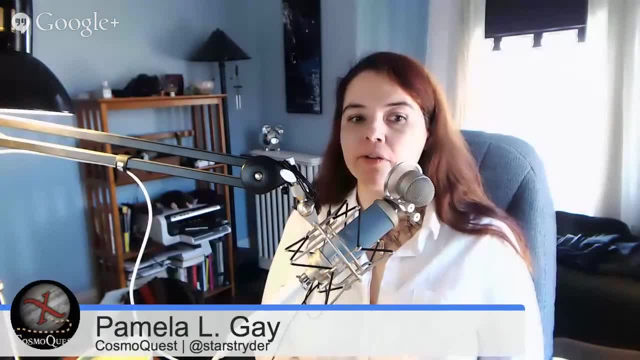 This is Well, and it's not just variable stars, You can also do photometry on galaxies. And most of the research that I've done and all of the research I've done that hasn't made me hate my computer has been based on photometry. 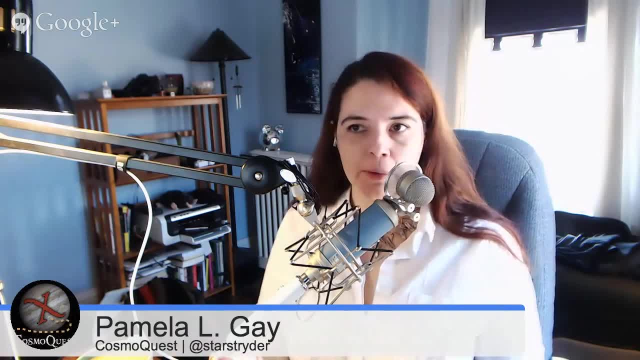 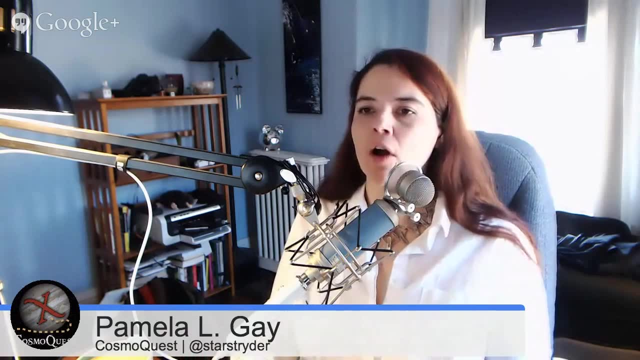 So when I was in graduate school I studied variable stars in the Ursa Minor dwarf storoidal galaxy. I studied galaxy clusters at what we would now call low redshift, but back then we called moderate to high redshift. So I've done a lot of research on that. 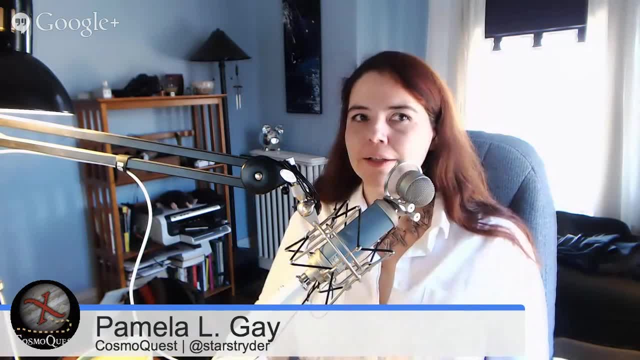 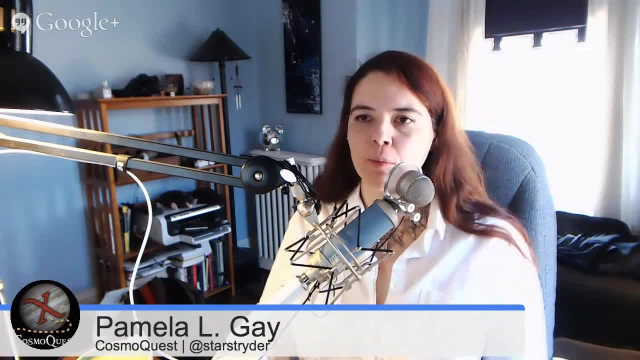 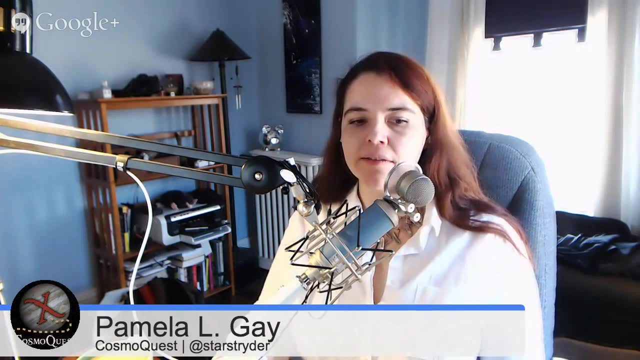 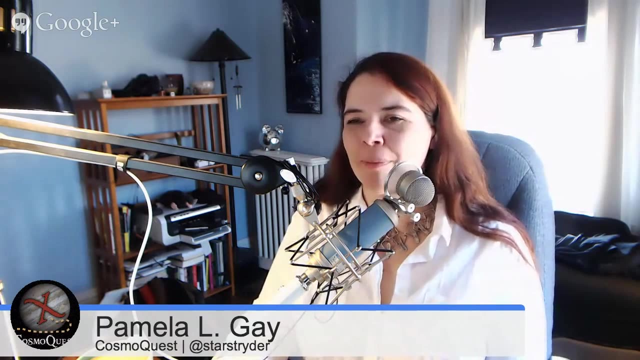 And you just kind of treat them like stars when you study them with CCDs. And so most of the work I've done has been: let's take pretty pictures of things, except ignore the prettiness and get at just the science. And even as an undergrad, using much earlier technology, it was all about let's just see. 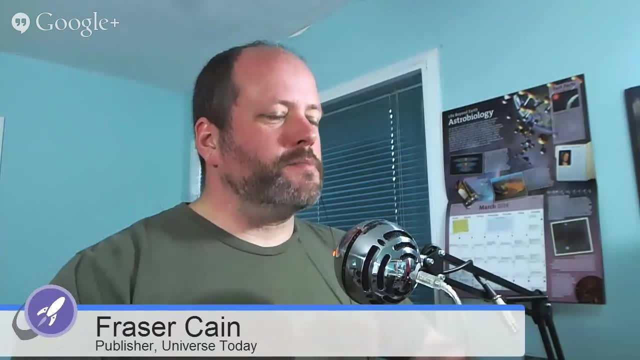 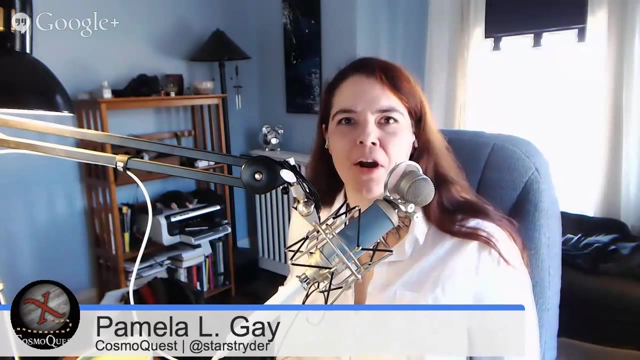 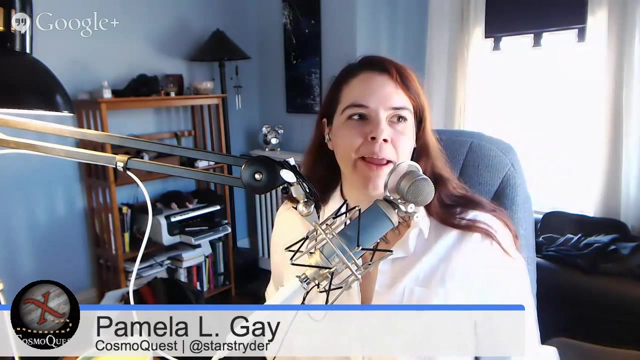 that light. So give me then I want to hear some stories. Okay, So what was like your research and how did photometry kind of play into it? So what is the title of one of your research papers? Oh man, the Blaschko effect in RR. Lari, I've done work on HLEO. I've man my, unfortunately. 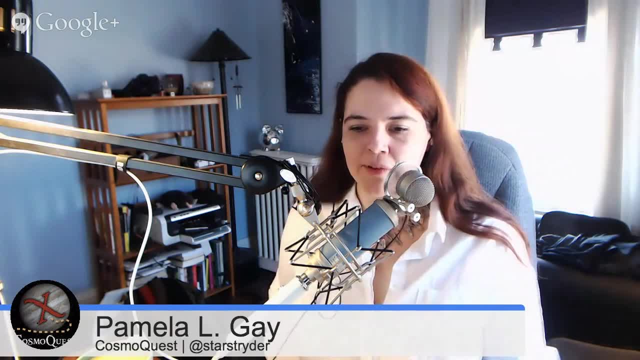 master's thesis. research got totally sniped by the Hubble Space Telescope. but there's some posters out there on using the variables. There's some posters that say you know, you can't really see the star from a star in the Milky Way. 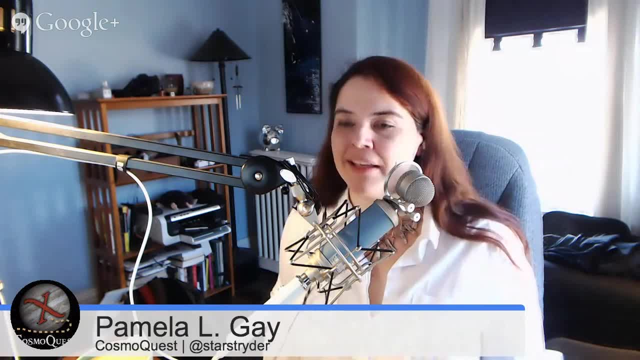 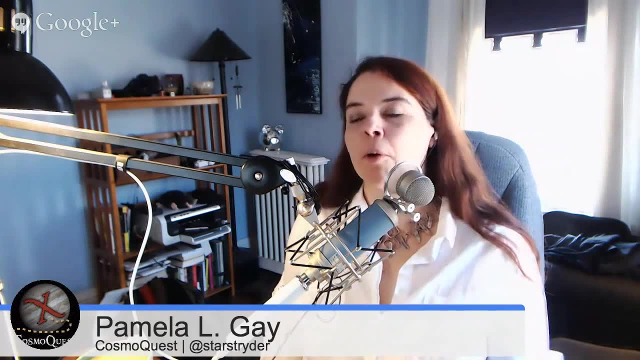 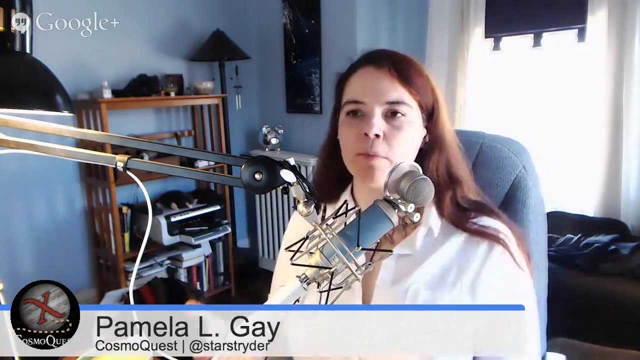 You have to be able to see the stars in the Earth's minor dwarf's roidal galaxy to understand the stellar population distribution. That may be one of those things where my poster led to one of my greatest moments of sadness. in my research career I was at an American Astronomical Society meeting and one of the awesome things about 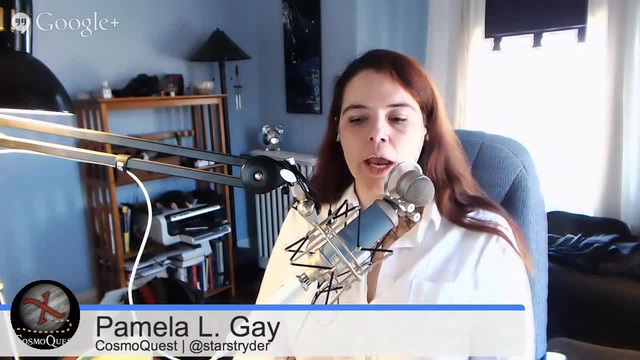 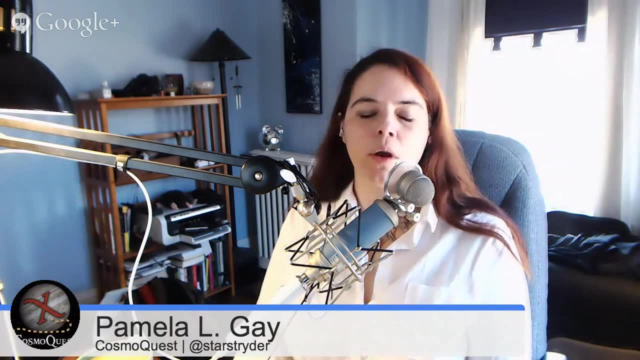 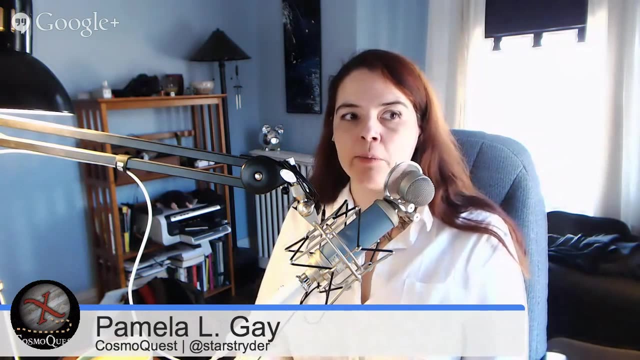 photometry is, if you have a reasonably good telescope and you are careful in what you're doing, what you do, you can make up for the telescope being small by just observing long enough, And I observed these faint 20th magnitude variable stars in Ursa Minor using photometry. 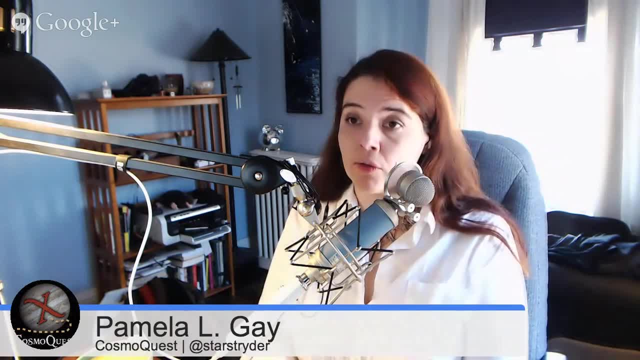 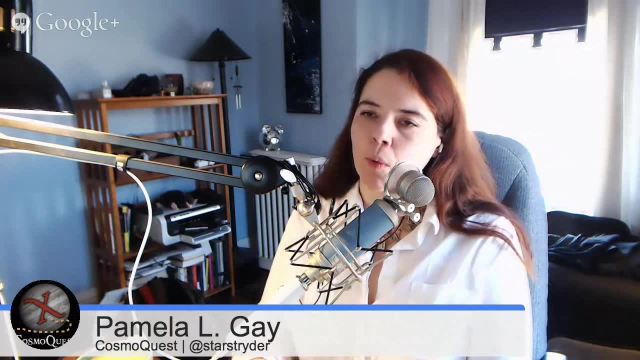 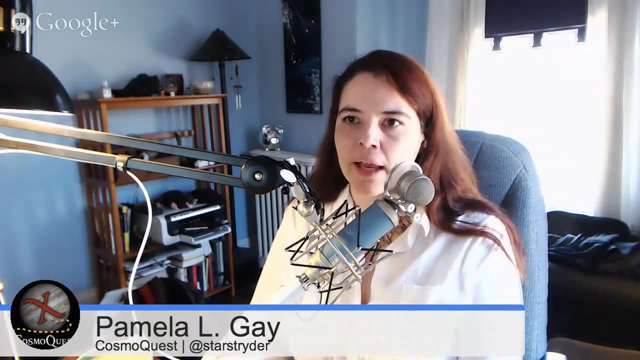 to measure how their light varied over time And with our Olaris. the period of the stars related to metallicity, to type of star, to a whole variety of different things, And then the brightness of the star is related to distance, and all of them have basically the same luminosity. 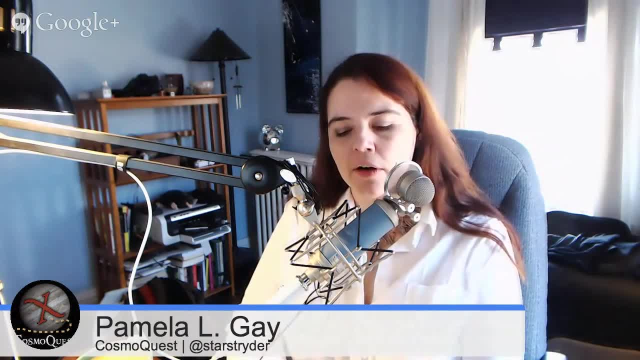 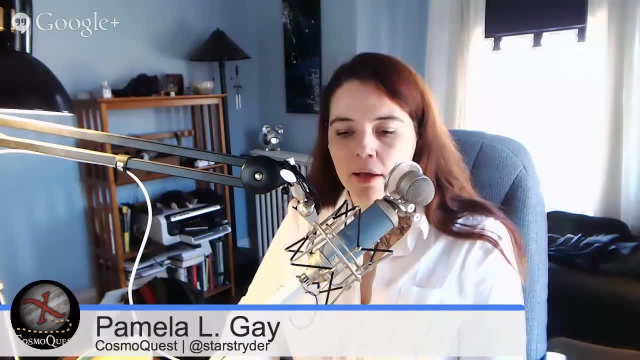 So you can pull apart all these different, how many stars have this type of period, how many stars have this kind of period? and look at all of this and realize, huh, all of these, even though they're so faint I can't get a good spectrum of them are probably made. 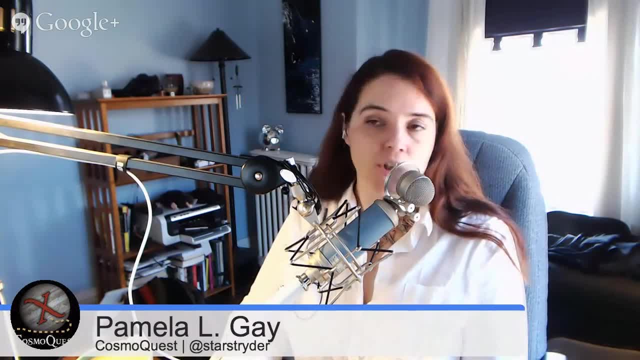 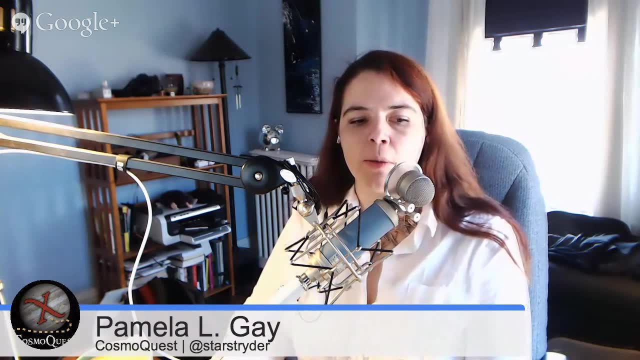 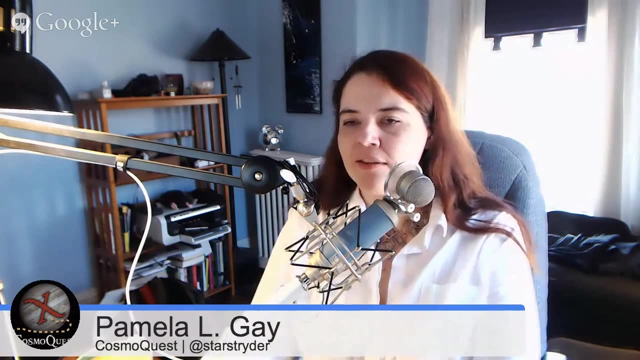 of the same stuff. All of these are basically the same age and that's just the RLRs. As you keep going looking at stellar populations, when you start to find other kinds of variable stars, each kind is a test particle saying, hey, there's stuff this age and this metallicity. 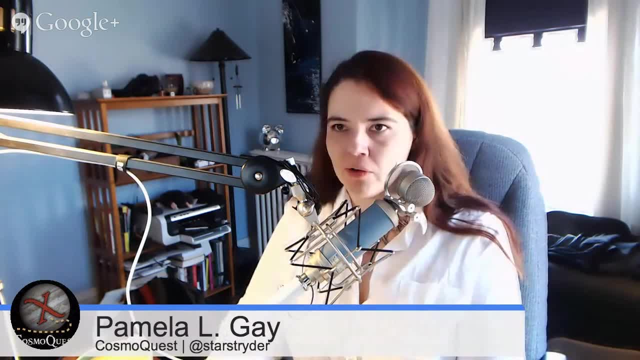 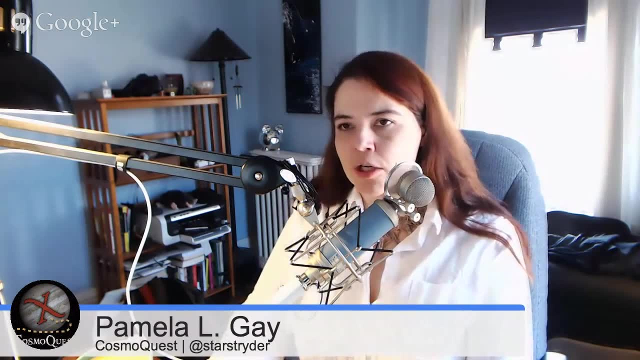 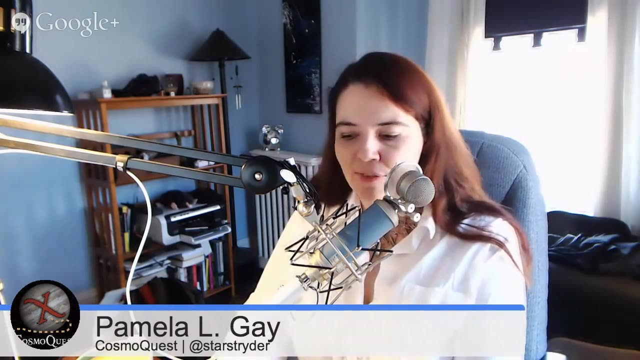 here, because if there's more or less metals wouldn't pulsate, If it was older or younger wouldn't pulsate. And when I looked at Ursa Minor and put together all of the information I could learn from the variable stars, I was able to pull out the details that this little tiny faint system. 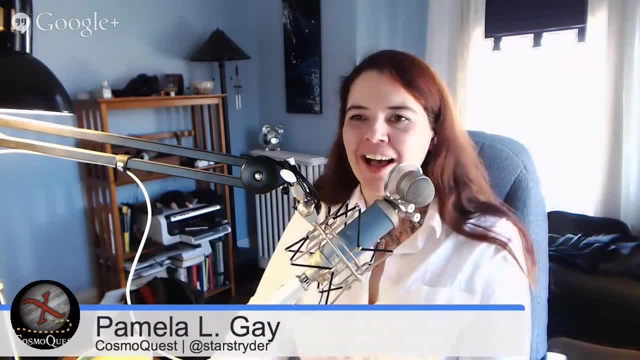 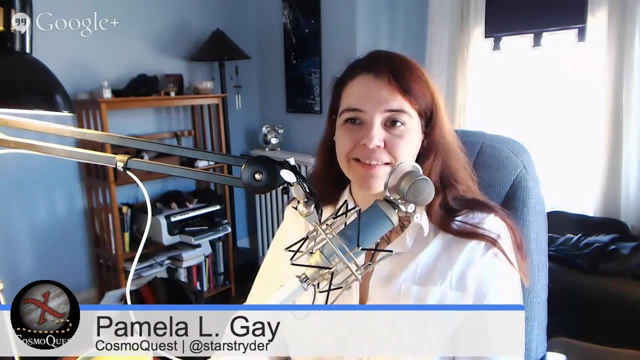 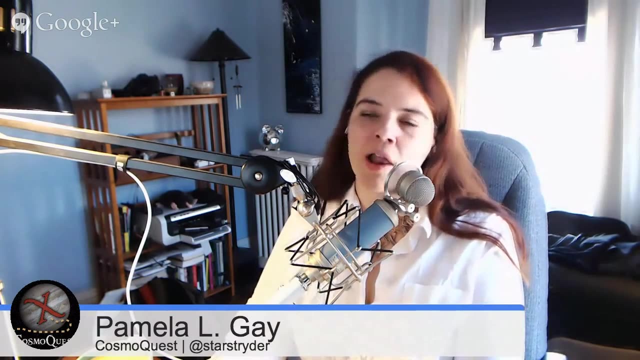 that I observed with a 30-inch telescope. all the stars had come out of a single epoch of star formation, which for a galaxy is pretty cool, But it's such a small galaxy that it was basically one of these great situations where this little tiny galaxy used up all. 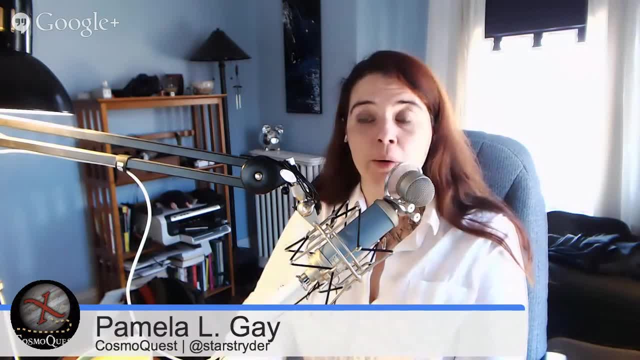 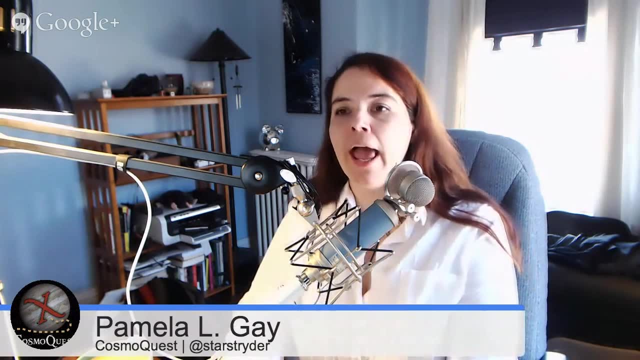 of its material for star formation in a single go. And I was stupidly proud of my results, hanging my poster up, getting ready to write up the research paper for publication, And right next to me, Ken Miguel's hanging up his poster on the Ursa Minor dwarf galaxy. 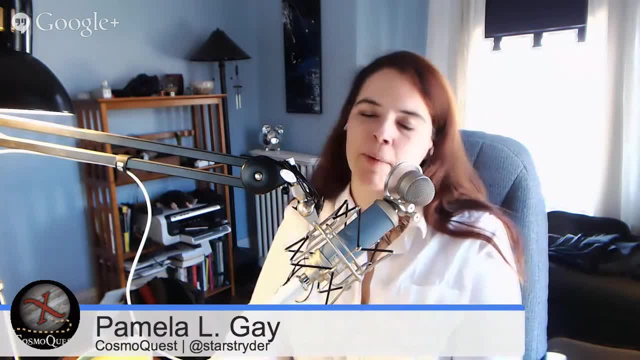 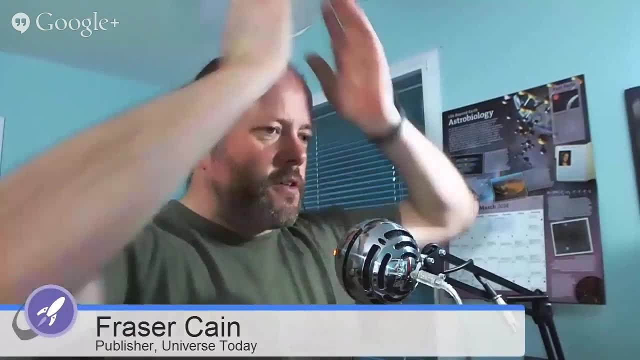 showing the exact same results using an HR diagram with the Hubble Space Telescope and much better quality of everything. Wouldn't you just high-five each other, though, and that's just like confirmation for both? Yeah, I think that's a great way to put it. I think that's a great way to put it. I think. 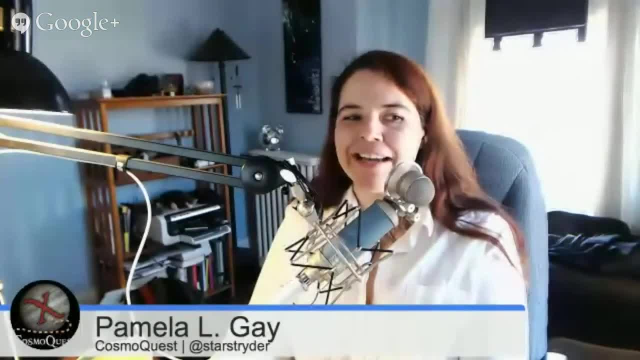 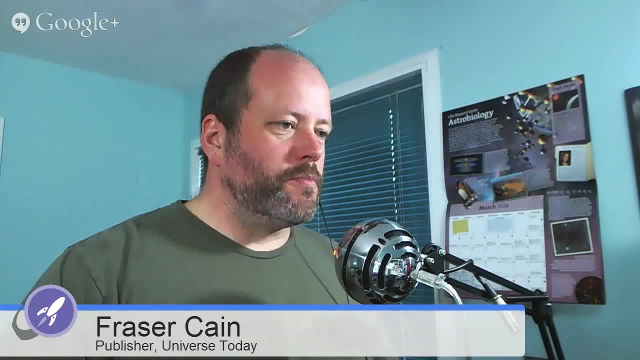 this? No, Did he not even let you participate in the paper? Did you not be a co-author? Well, I had nothing to do with his results. Well, I know, but you had your results and they're the same as his results. that'd make. 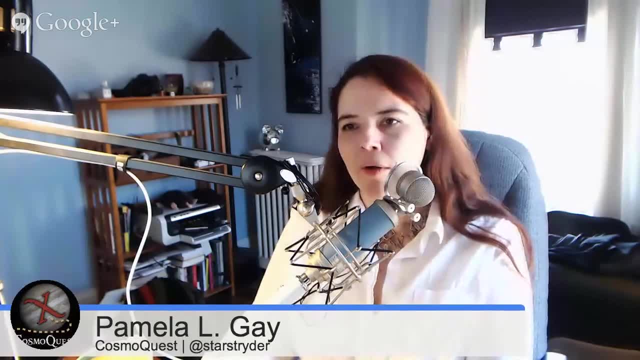 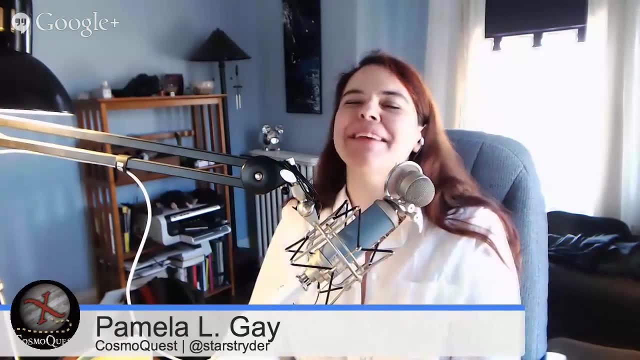 them look better. Yeah, but my poster was already going up in the proceedings. You should have just shuffled your papers together and then just handed it in. It was just one of those icepicks. two years of my life and like a hundred nights at the telescope getting my results and 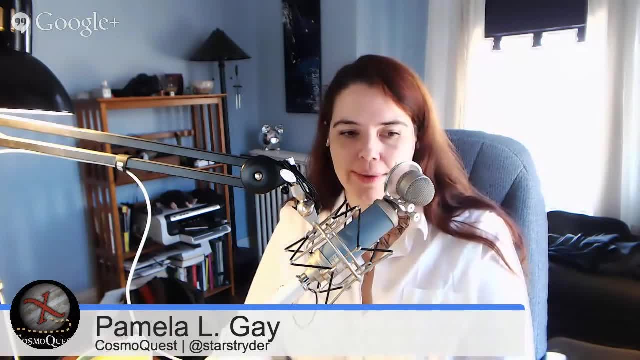 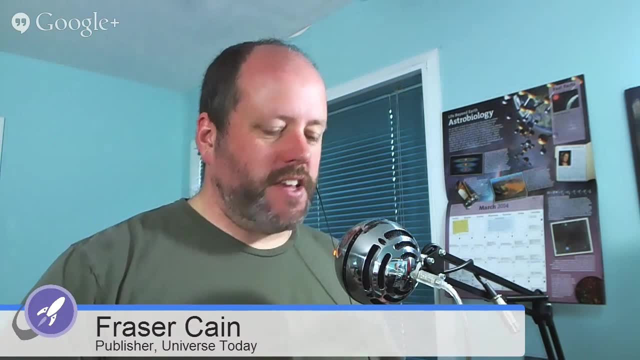 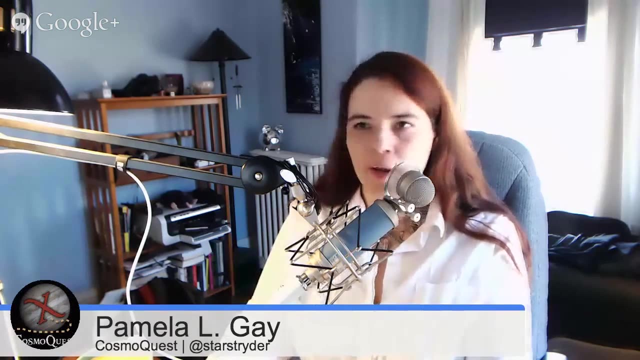 it could also be accomplished with Hubble very quickly. yes, of course it could. much better than was all right. so photometry: it is detecting the changes in brightness from an object, be it a star, be it a galaxy, a galaxy accretion disc around a black hole, exactly um so. so what is like? what do? 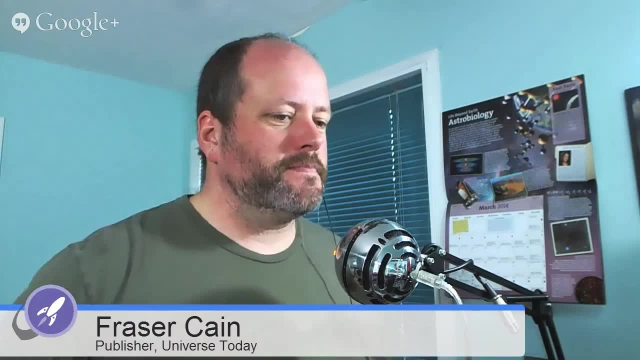 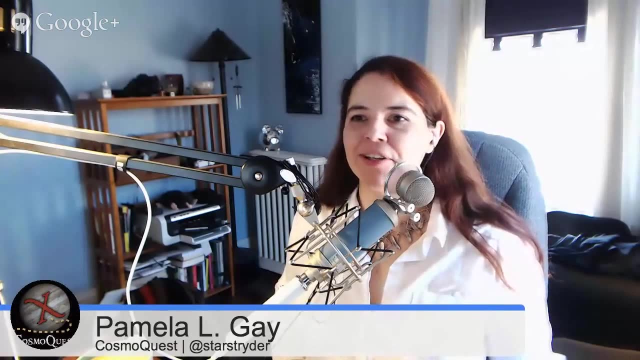 you. what is the gear? what is a photometry thing? if I can hold a photometer, photometer, photomultiplier, tube, photometer, yeah, what would this thing look like? um, they come in a variety of different forms: the old school ones that still get used. if you're trying to do high speed work is just a simple. 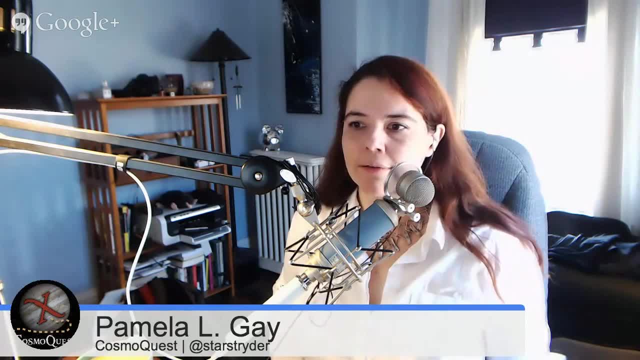 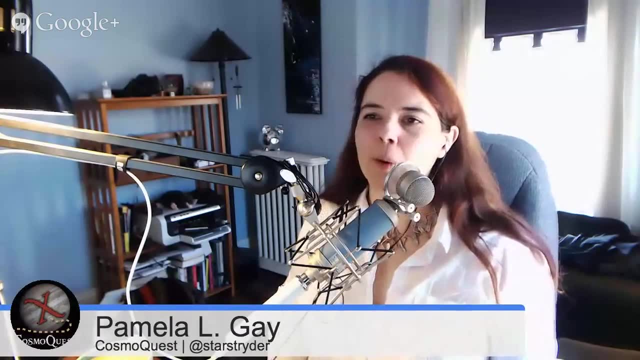 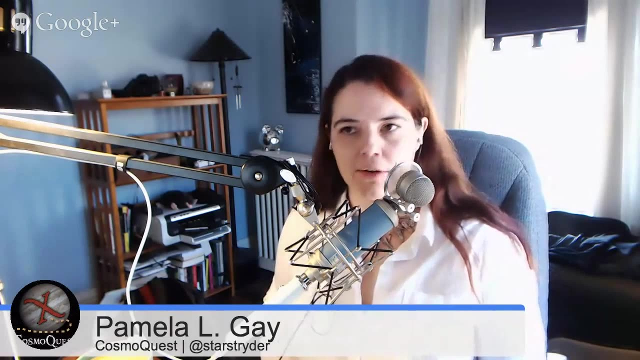 photomultiplier tube. it literally looks like a tube, kind of lame that way. um, light goes in one end, okay, okay, light goes one end and it goes light, no light, and it very, very precisely counts the number of photons coming in. you can stick a filter in front of it so that you know what colors the photons coming in are. 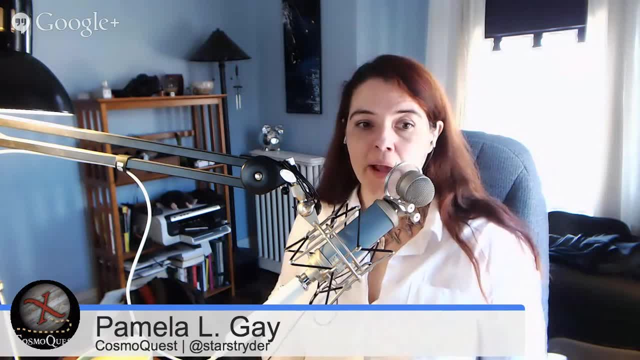 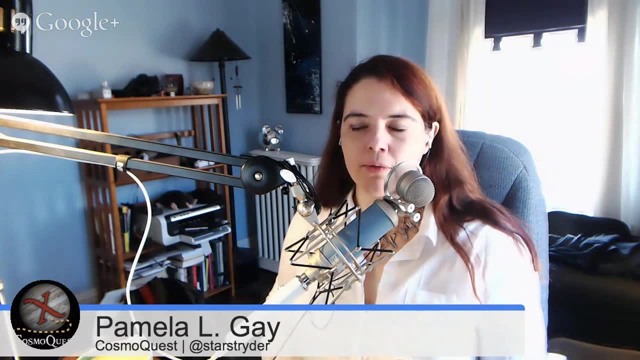 and what is glorious about these is there's really not a whole lot of data reduction involved. you point your photo photomultiplier tube at the star galaxy, whatever it is that you're measuring. you then point it at the star galaxy and you're like: oh my god, I don't know what to do with this. 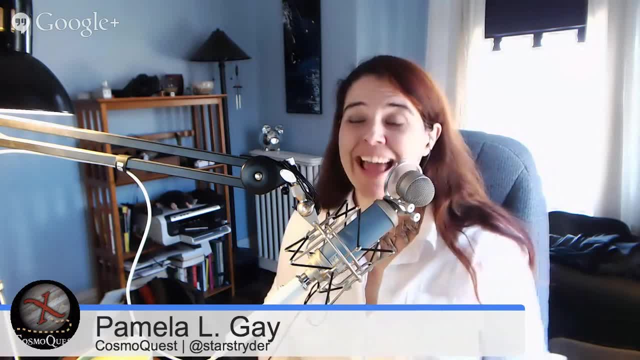 so it's very difficult to figure out how much light is coming in at this point and you can start to take a lot of data from the stars, right, and then you can go back to the stars and you can start to look at the sky. subtract the value of the sky from the value of the objects you looked at. you have your. 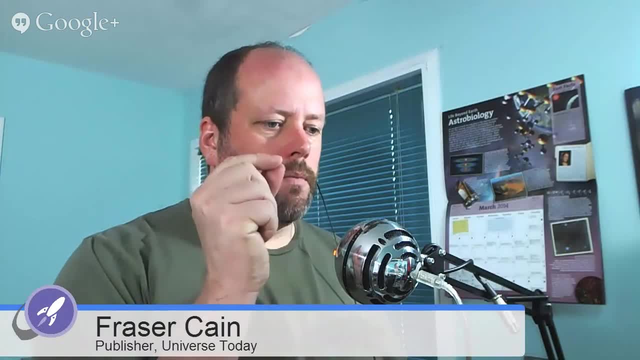 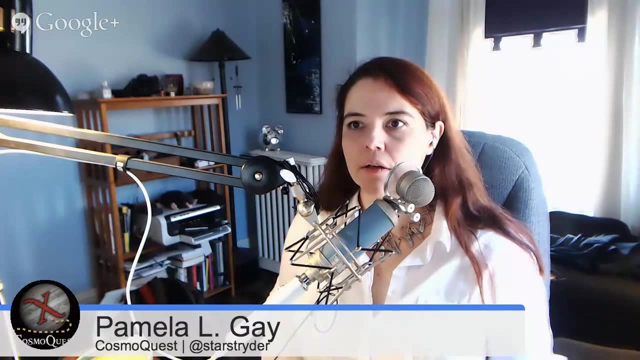 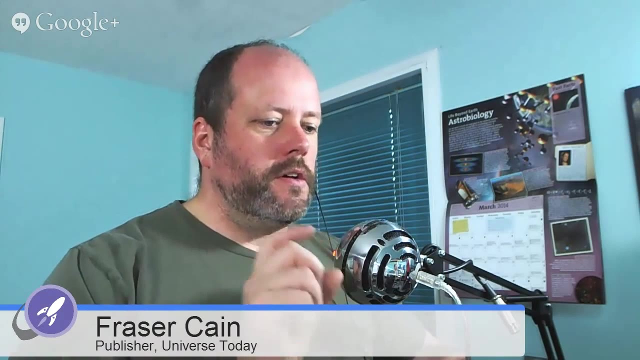 data and do you and like, do you say like you can count, like the number of photons, like how, how precise can you get with this amount of of? um? they claim 95 percent quantum efficiency. wow, yeah, so. so in other words, your, your error bars are going to be now like, if it's within the five percent, then you're. 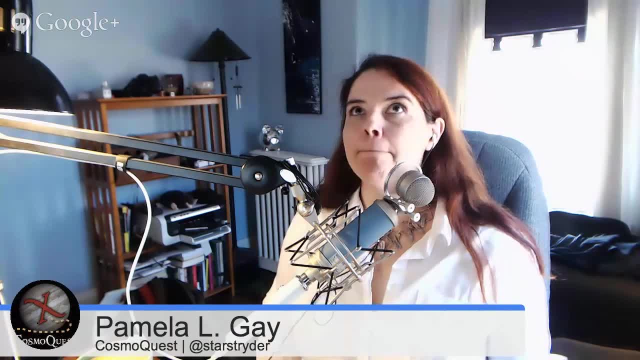 probably going to say it's error. but if it's like 10- 50, then you feel the bigger issue comes from the atmosphere. um, so so you, you're going to have to kind of look at it and see what's going on. you're going to have to figure out what's going on. you're going to have to figure out what's going on. you're. 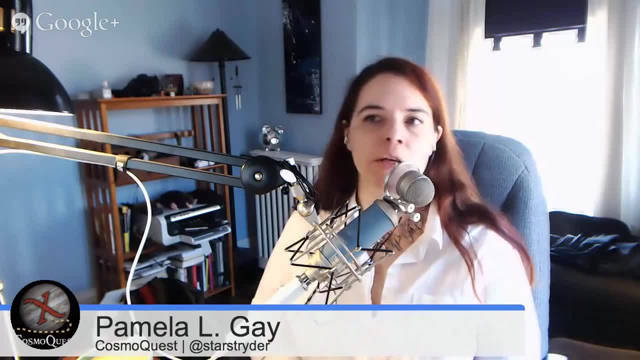 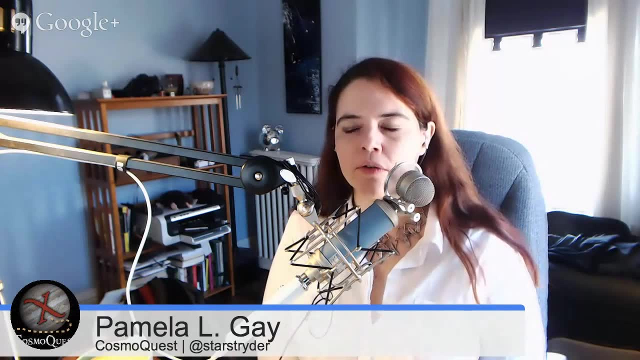 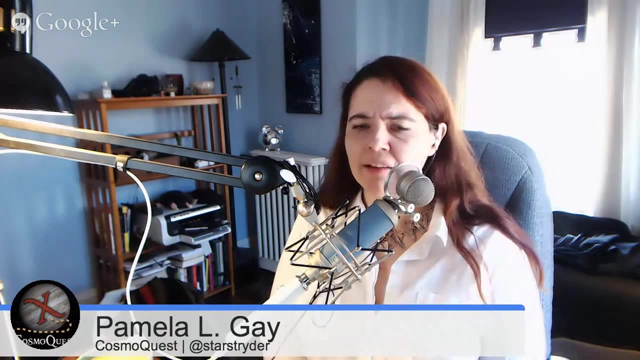 You do have to correct for sky glow. You have to worry about changes in transmission of the sky. As your object wheels from straight overhead towards the horizon, the atmosphere is going to start knocking out more blue light. But at the end of the day, the detectors are really good and this is why, with the even 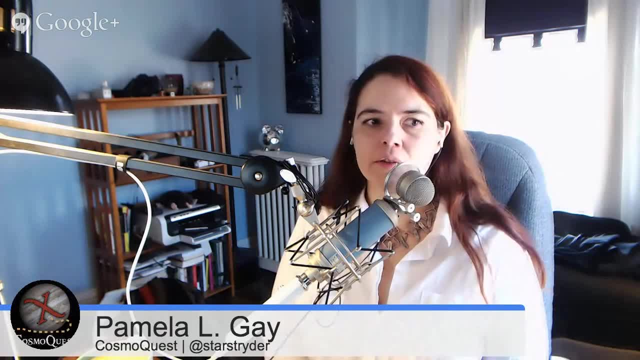 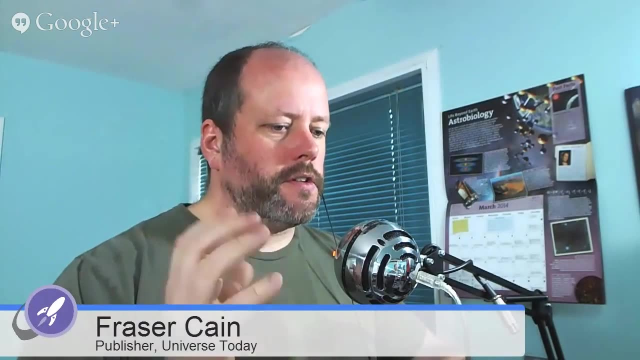 not as good CCD cameras. we can spot planets going in front of other stars. It's a photometric process. Kepler used photometry to discover planets. What will you get as a result? You're going to have the photomultiplier. you're going to have this tube in front of 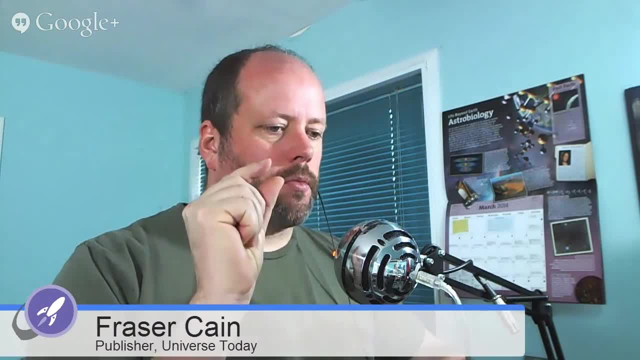 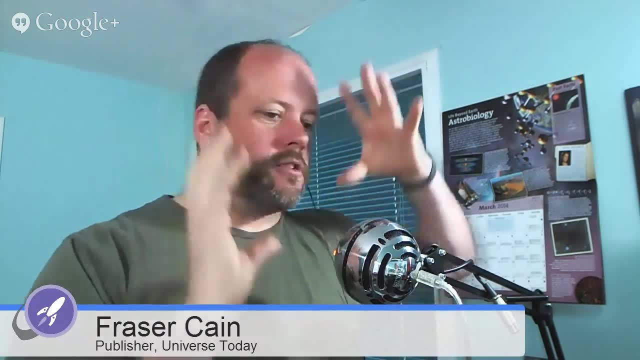 the telescope, It's only going to be able to see the photons from a very small portion of the sky. I've seen ones that are more elaborate, where they're gathering multiple stars all at the same time, or multiple galaxies. Right, so that's the CCD. 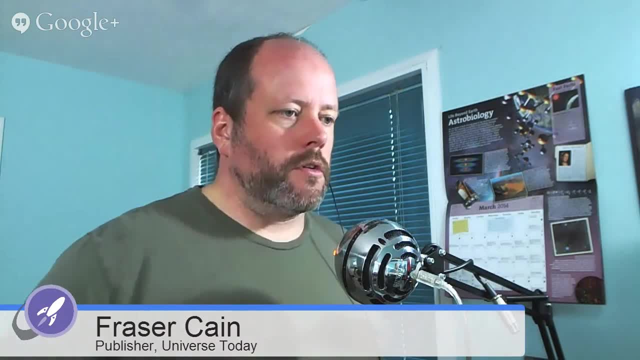 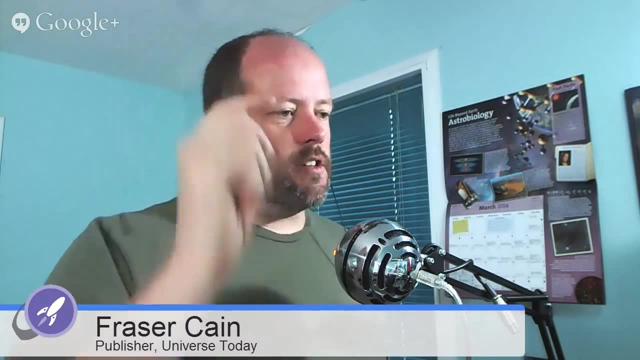 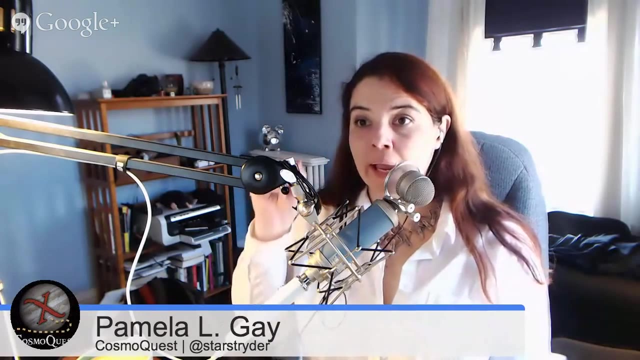 Right, but mostly you're aiming for one little chunk of your sky, right? You know what I mean. like, the size of the sky that you can see is pretty small. So when you're doing photometry, what you're interested in is the light from a single object. 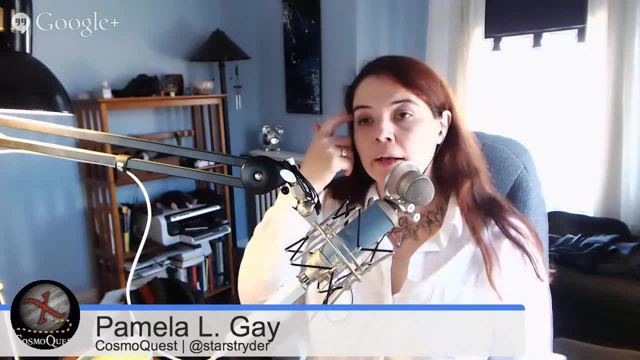 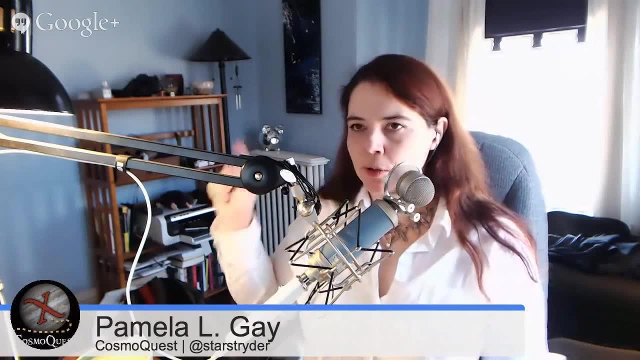 or a single region of light from an object. And if I take a big picture of the sky and I look at the distribution of the light pixel to pixel to pixel, it will be essentially a central pixel that gets a lot of light Right. 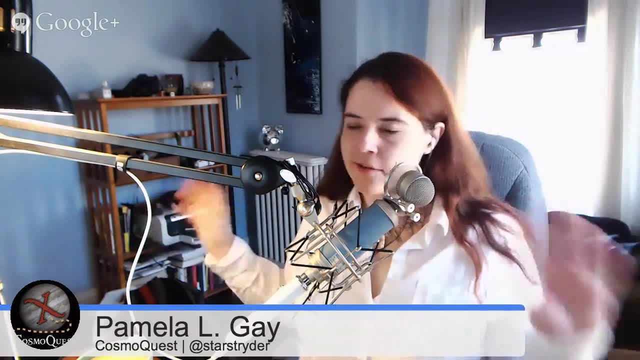 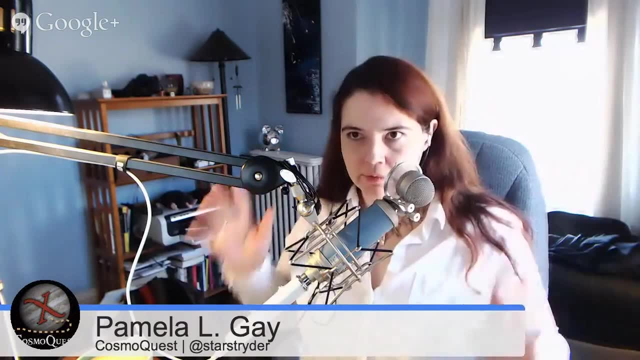 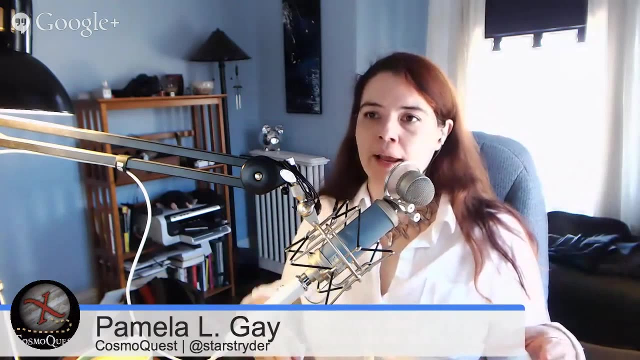 Right, And then the light tapers out towards the edges. The distribution of how the light tapers off depends on the sky, depends on the detector, but it tapers off in a nice neat curve And there's what's called a full width, half maximum to this curve. 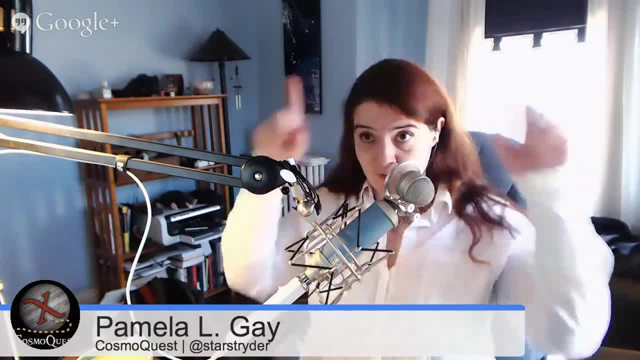 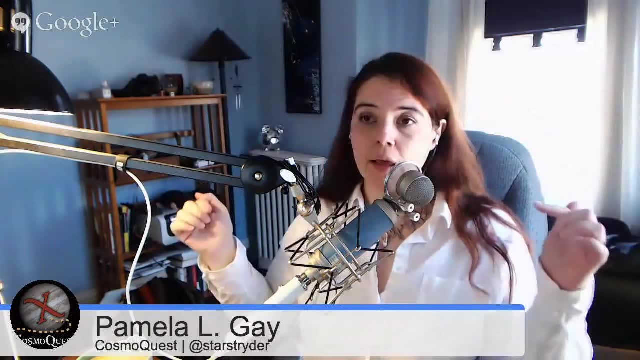 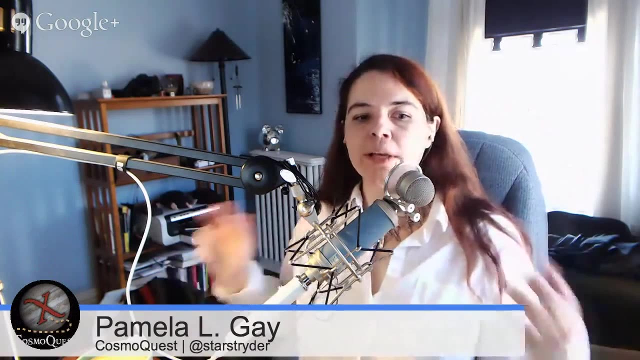 And so that's the width of the falloff curve where the light at that point is half of the maximum light coming in. So when we're doing photometry we try and collect everything that's within three to six times what that full width, half max is. 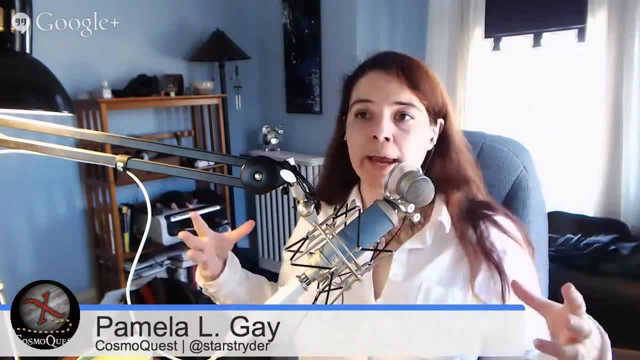 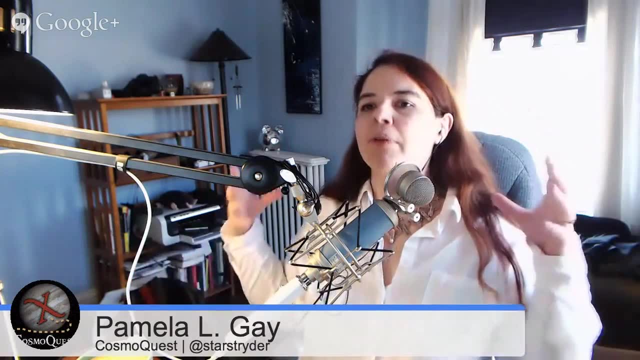 And that's what we consider the useful portion of the light coming in from the star. Now, if you keep going, our atmosphere blurs that light out for a long time, But that's the core light that allows us to get the bulk of the science done without getting 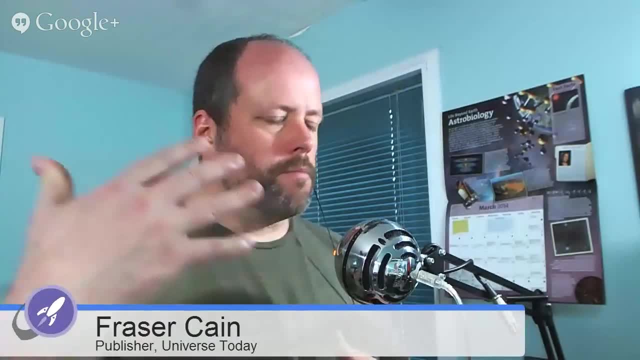 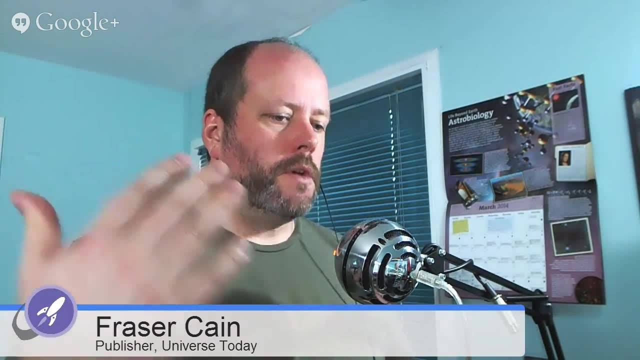 a lot of noise from the sky in. Now you said that you can put filters in front. So, for example, if I'm only looking for, If I'm looking for the blue end of the spectrum or the red end of the spectrum, if there's 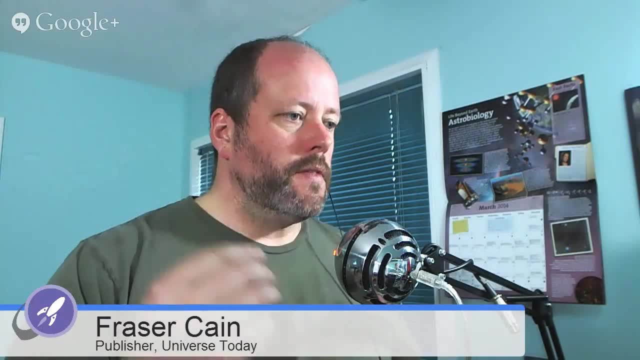 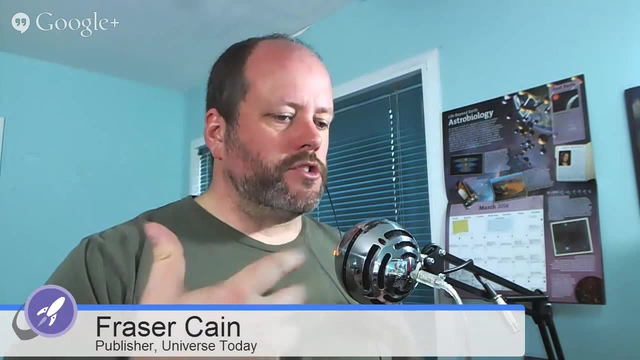 enough light coming from the star, I can start to segment that stuff out and see. So could you have a situation where the overall light of the star seems to be the same, but there's changes in brightness from some of the photons, from some of the types of photons? 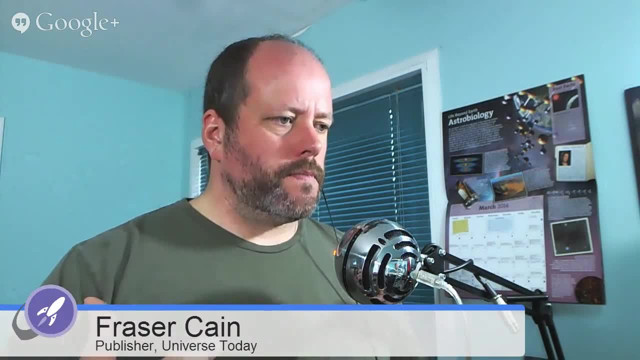 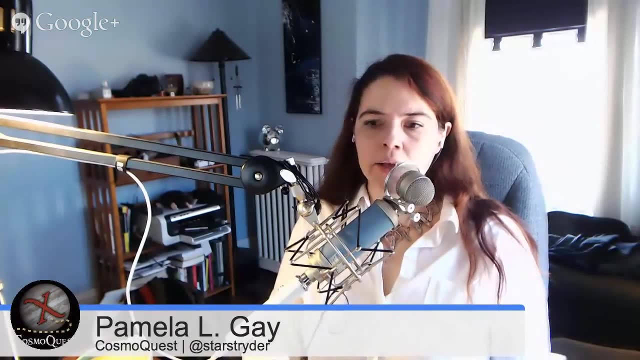 Like the heat. I guess if it's heating up, That changes the entire curve because it's black body radiation. So this is one of the awesome things about doing photometry. Yeah, So what you're doing is when you're doing spectroscopy, when you're dividing the light, 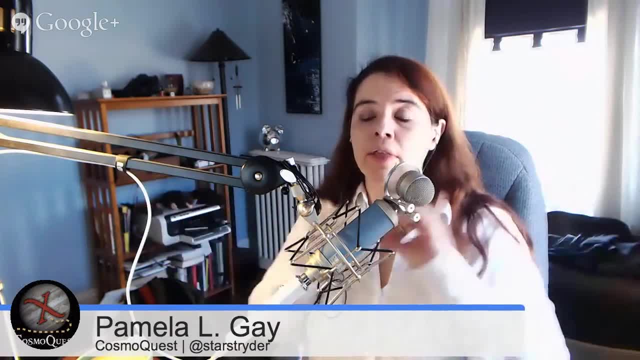 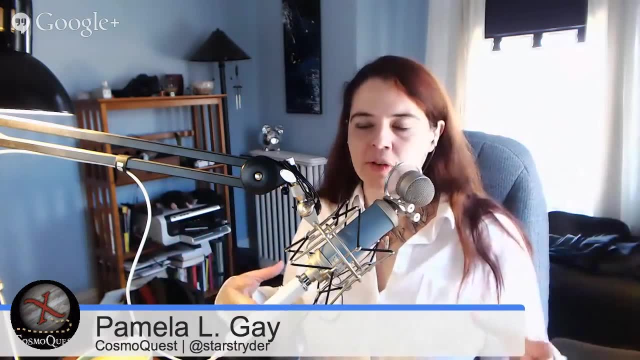 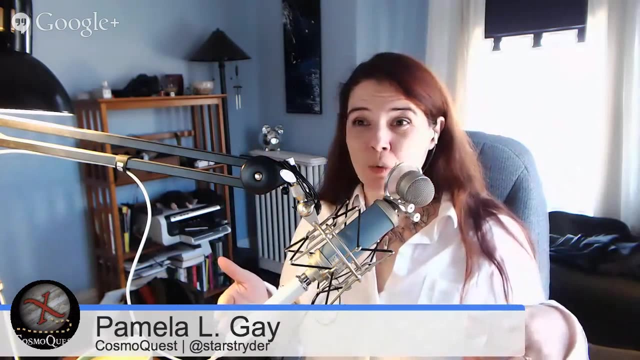 of a star galaxy, a source out into that full rainbow to measure how many atoms of this, how many atoms of that, what molecules are there, what redshift is it at? you have to spread that light out a whole lot, So you're starting to get less than one angstrom of light per pixel, and that's like 10 to. 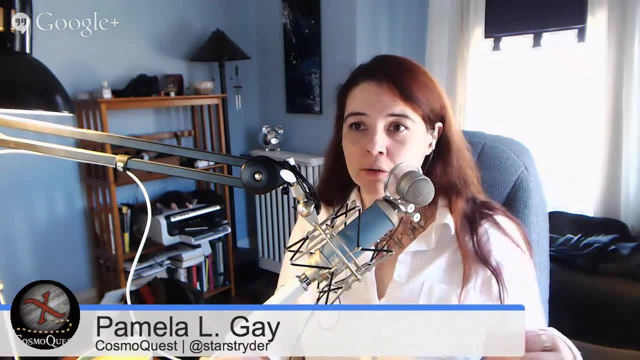 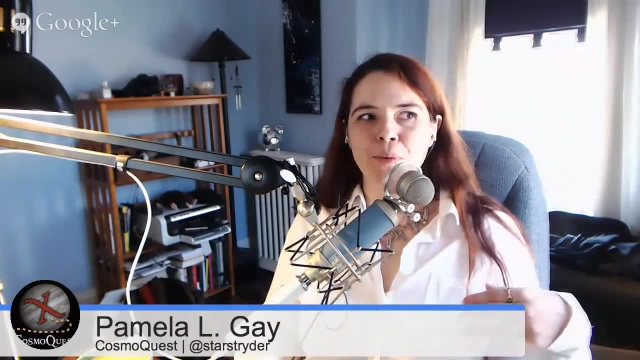 the 10th of a meter, 10 to the minus 10th of a meter, tiny fraction of the light into one small bit. Well, with photometry you're looking at sometimes a couple hundred angstroms, a couple thousand. 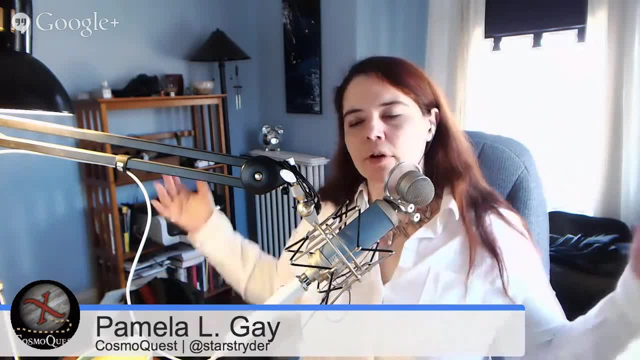 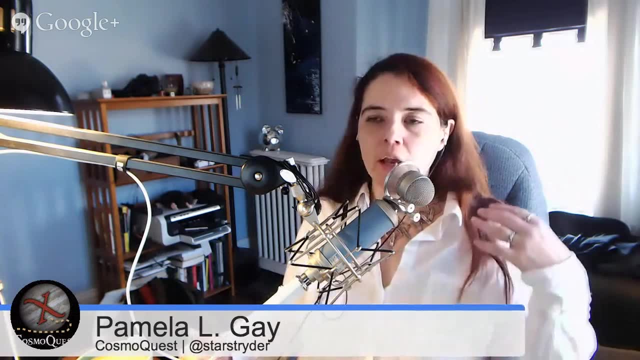 angstroms, depending on what you're trying to accomplish, And so you're getting a whole lot of colors of light in. But because the shape of a black body curve is very distinctive, that curve of light that describes the temperature of an object. 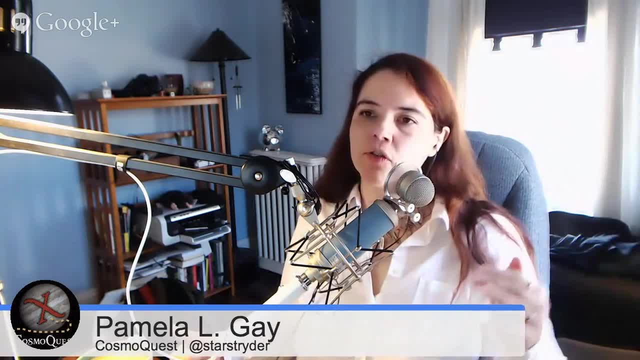 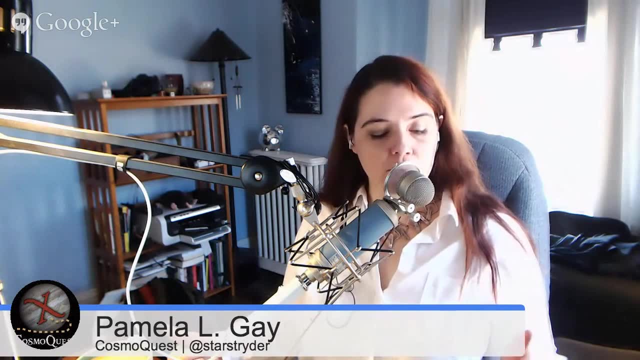 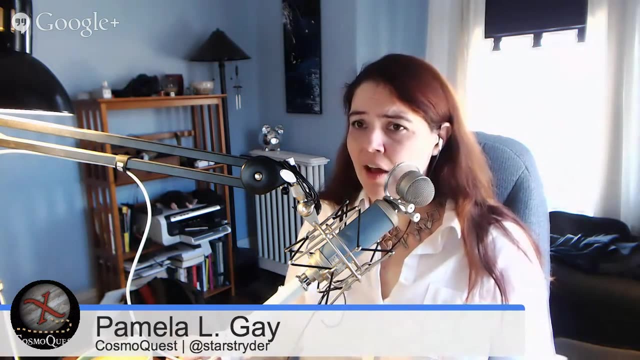 The peak of the object. Yeah, The peak of the light shifts towards bluer and bluer colors. the hotter an object is, That shape is very distinctive And if you sample an object's light at three different places, you can fairly precisely get at the object's temperature, because only one curve is going to fit to those three lines. 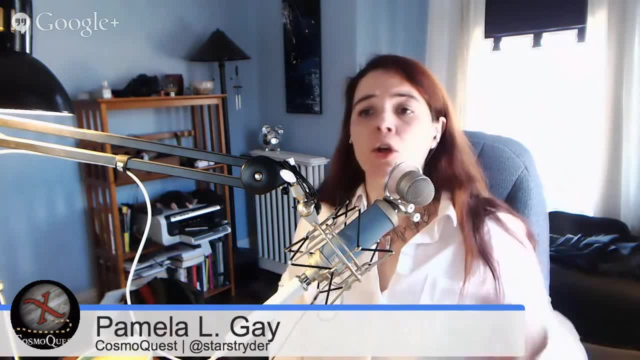 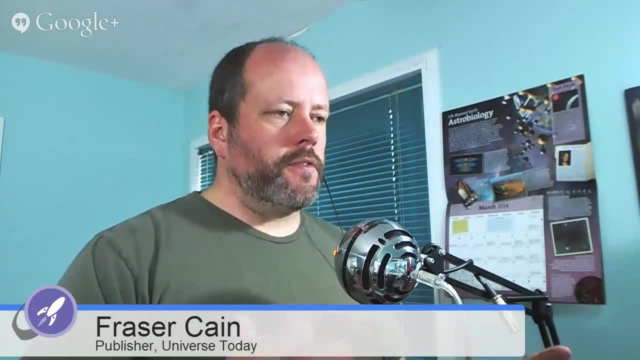 And if you have extra information you can sometimes even get away with just two colors of light if you have to. Right- And I guess I mean with spectroscopy, as you mentioned- You know the difficulty is getting that light spread apart. 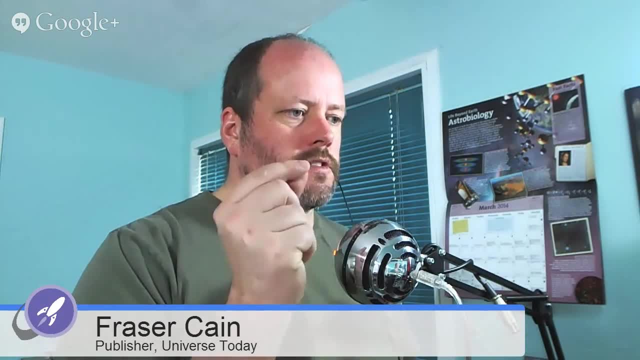 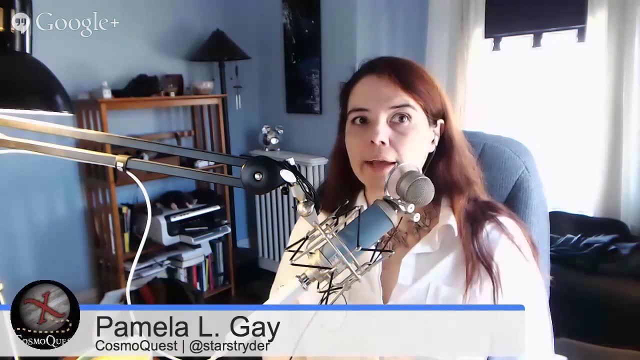 I guess with photometry, the real challenge is to measure those slight changes in brightness. That's how you find the planets, That's how you find. you know that's tough, Well, and you're not always looking for the changes in brightness. 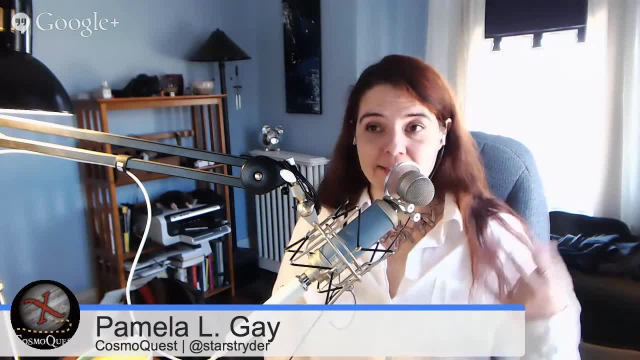 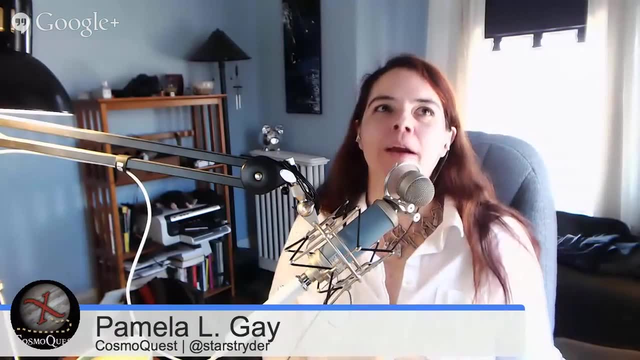 Sometimes you're just looking for stuff And that sounds lame but Super lame. So this is one of those rare shows where we hit nail on with my research. Yeah, Yeah, Yeah, Yeah, Yeah, Yeah, It's group research. 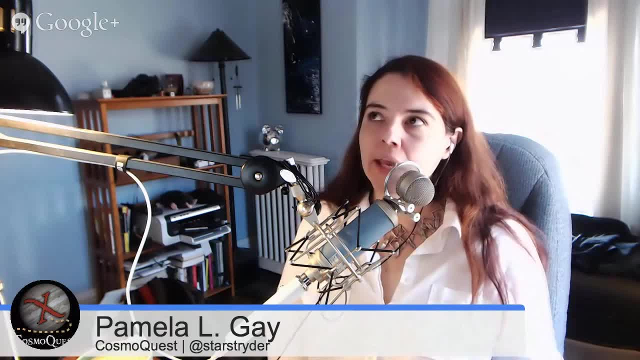 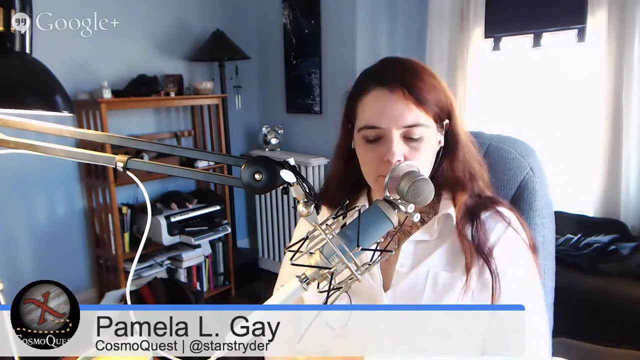 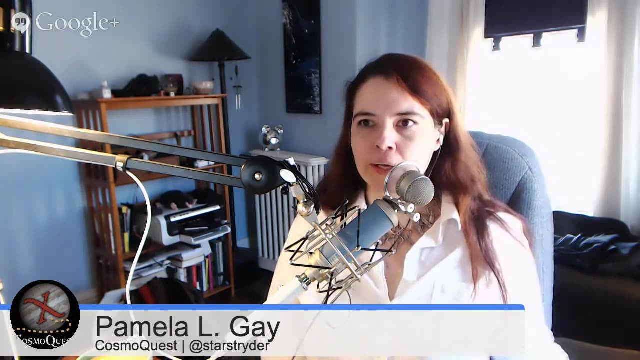 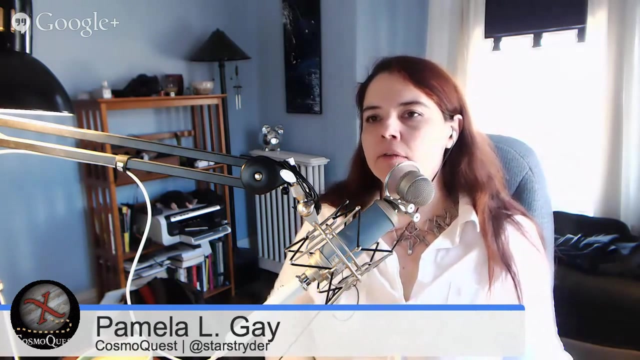 And when you're looking for galaxy clusters, you're taking images of sections of the sky and then going through and basically counting the density of objects across your image and what blurriness are they? Blurriness isn't quite the right word, but what spread does the full width, half max have? 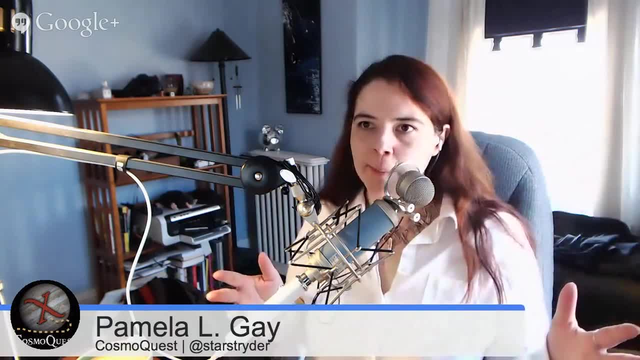 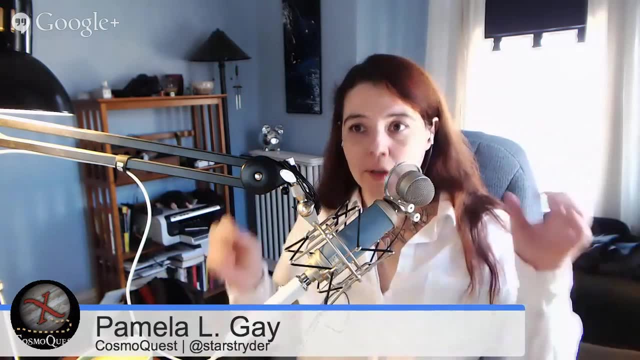 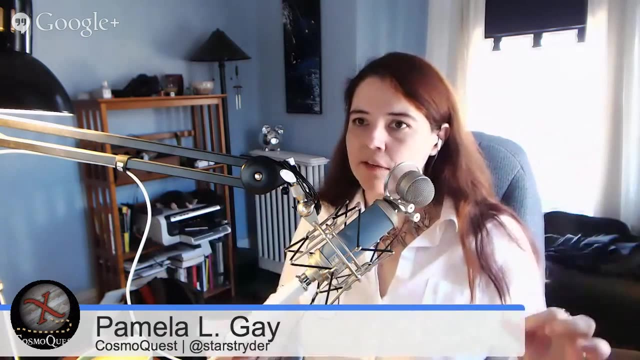 This slide was so hard to get around with. I have a little…. projections: idealistic, doesn't actually exist, but we're going to pretend for the points of this episode. telescope: When you look at stars all across your entire field of view, all of the stars will have the exact same point spread function. When you look 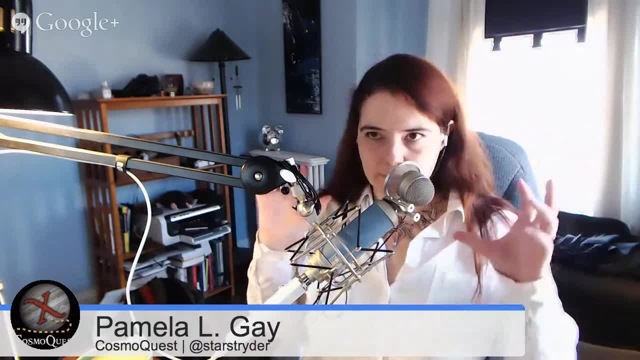 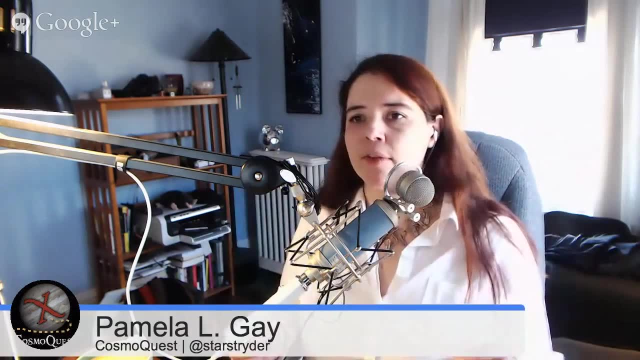 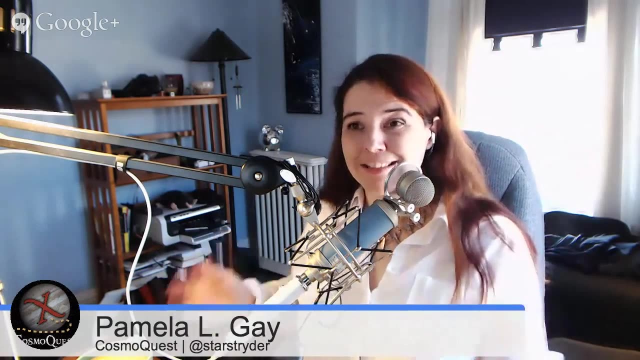 at how their light forms, that hopefully circular distribution that fades from the center towards the edge. all of them will have the same full width, half max. they'll all have the exact same shape. You can even, at a certain point, go huh, they're all slightly teardrop shaped. 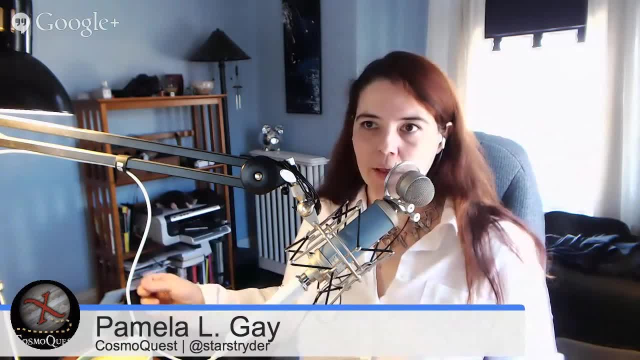 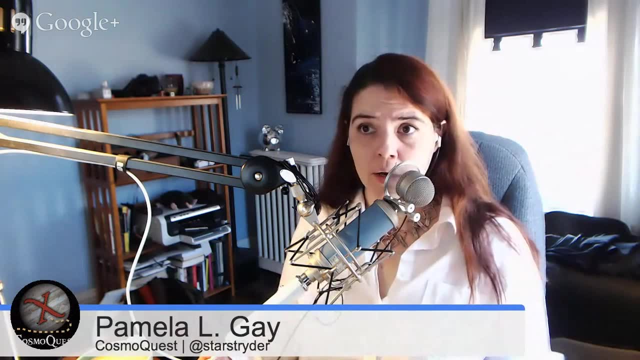 but all stars look the same. Now, a galaxy, even if it's far away, it's not a single point of light. the way a star is, It's point spread, function is going to be larger. it's going to be not necessarily the same shape and by looking for clusters of things that have 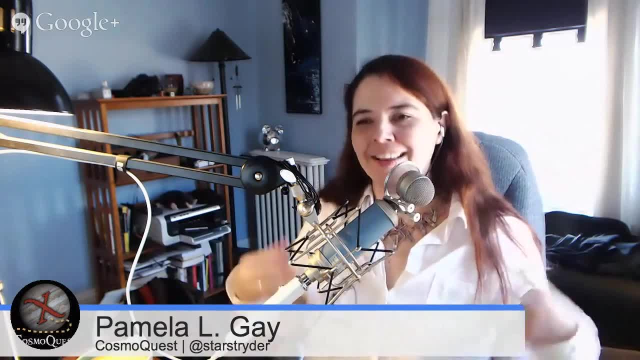 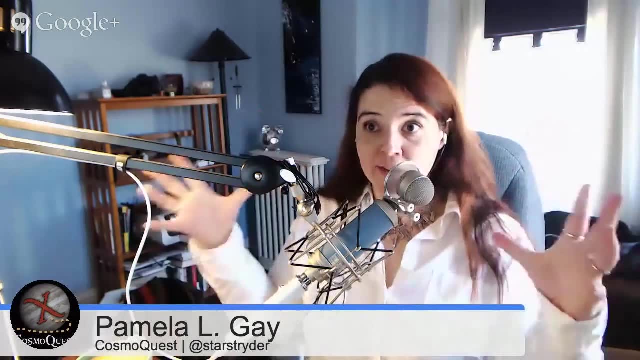 not the exact same shape. you can even, at a certain point, go: huh, they're all slightly teardrop shaped. You can even, at a certain point, go: huh, they're all slightly teardrop shaped. By looking at things with a not star point spread function, you can say this: cluster: 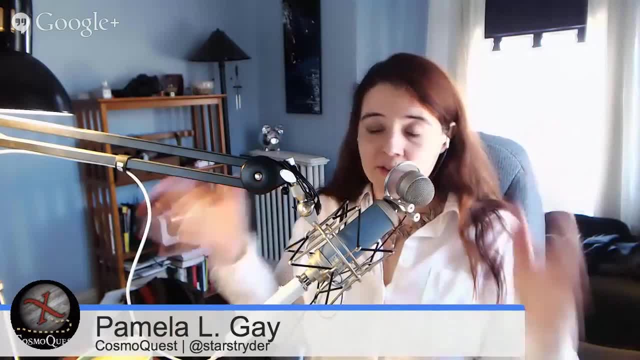 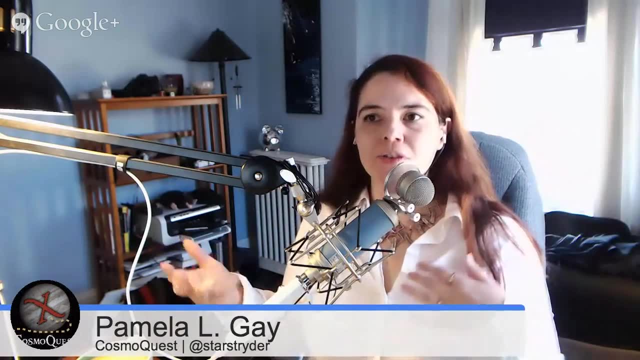 of things that I tried to do. photometry on this is actually a galaxy set, and then you can start looking at them and going: does the profile of colors match the profile of a bunch of galaxies that are located at the same distance? You can start to put all of 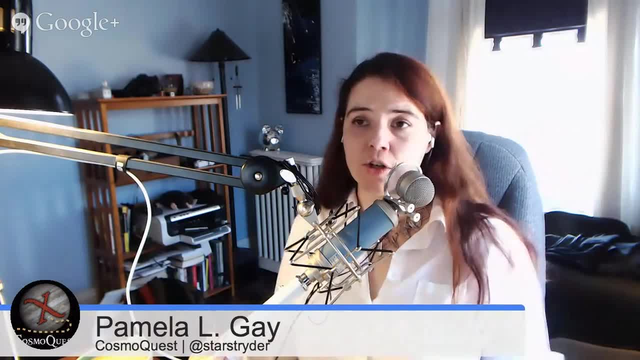 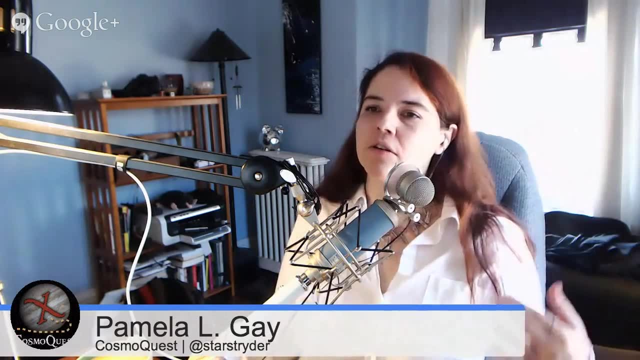 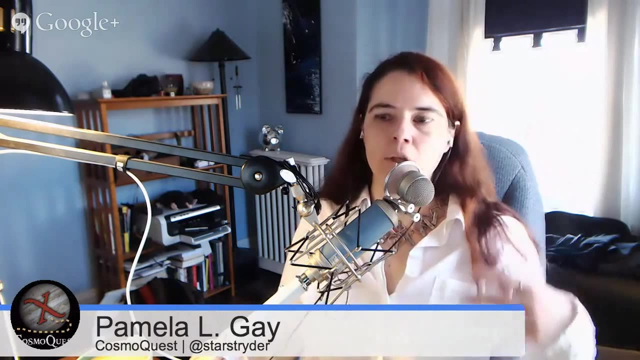 these pieces together to map out The structure of our galaxy. by looking at the density of stars, by mapping out the density of galaxies, you can start to get at where are the clusters, where's the large scale structure? and in this case, yeah, some of that stuff's varying in light. You have black. 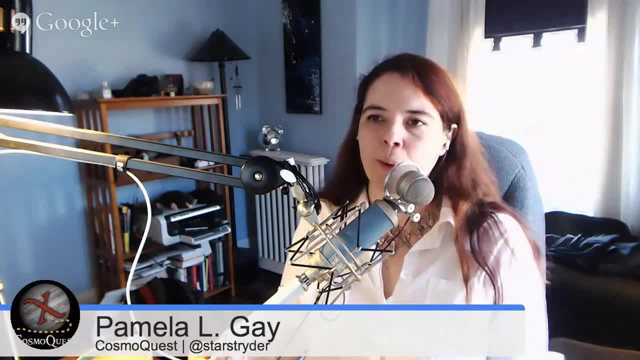 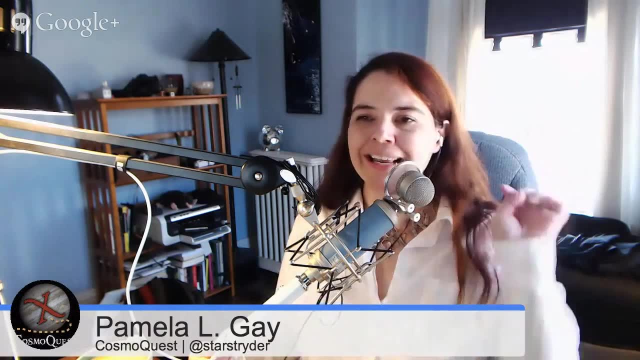 holes that get accretion disks that vary around them. but if I'm looking for a galaxy cluster off the bat, I don't care about those variations, I just care that point. spread function is not a star, And so can you do things like that. 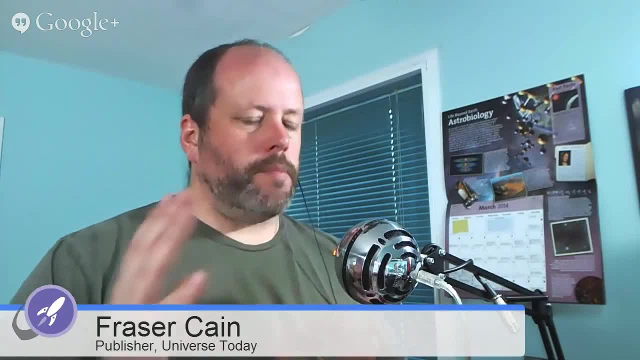 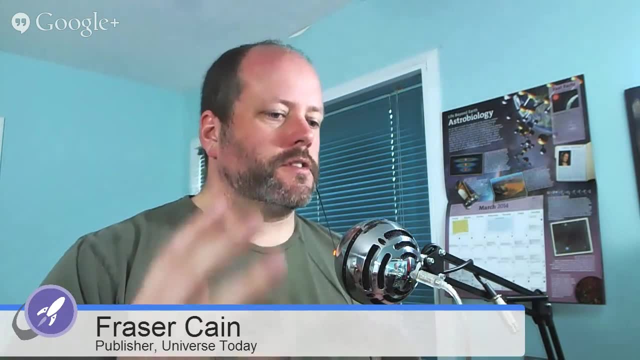 I can imagine when you take, just look at a picture of the galaxy, of whatever, of Andromeda, and you just see the structure and you see the star clusters and the central core and it all looks pretty. But I guess, if you're doing photometry and you're just carefully, 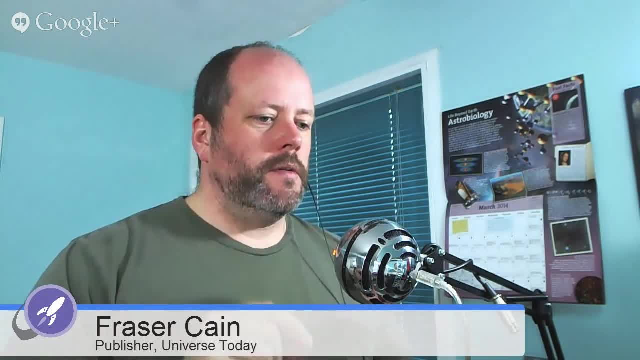 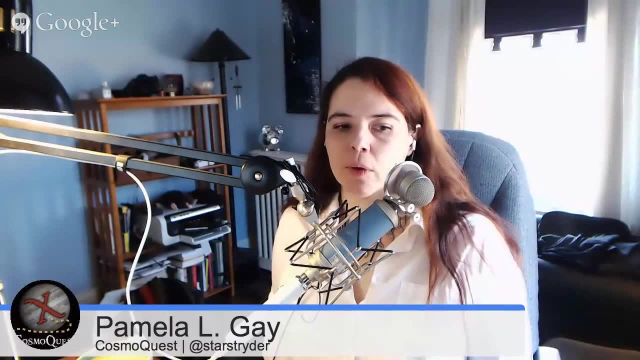 going across the galaxy bit by bit by bit, you're going to get these changes in brightness. that's going to tell you things about what's going on in there, And you start to use a different technique when you're doing that In general, when you 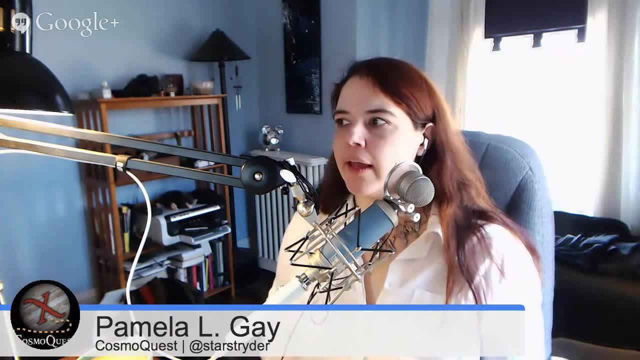 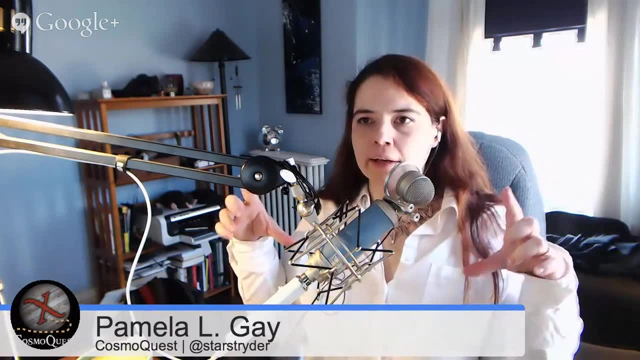 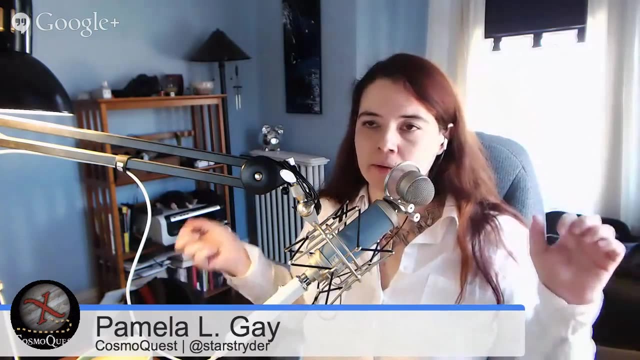 talk about photometry you talk about. You talk about something that we say you can put an aperture around. You can draw a circle around the object you're interested in and you count all the photons inside of that. You then draw a donut around that aperture, measure the sky, the nebula, the whatever. 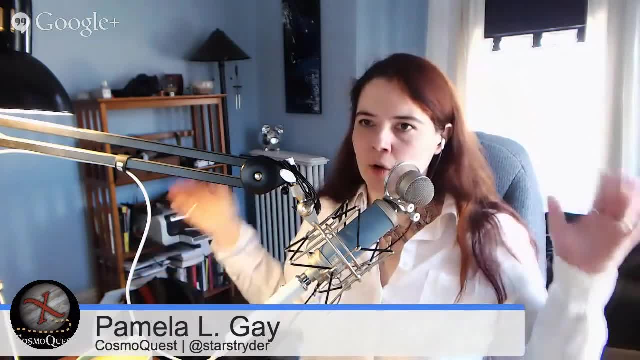 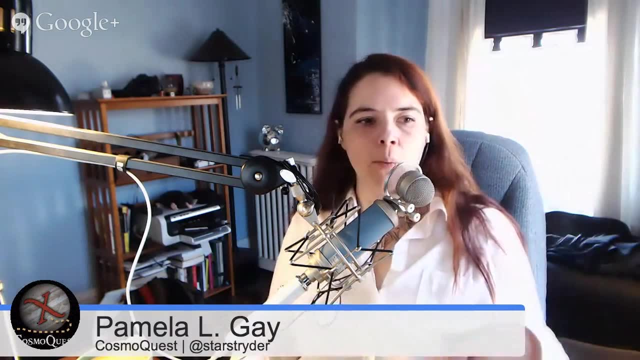 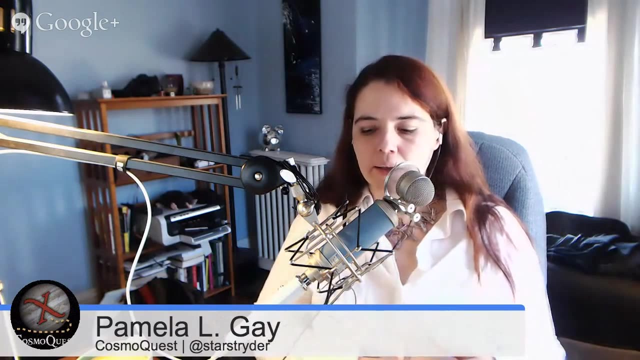 that it's embedded in subtract the average value of that donut and that tells you about what's inside of your aperture When you start looking at measuring the brightness of the brightness of distributed objects, of things that actually take up space across the sky. 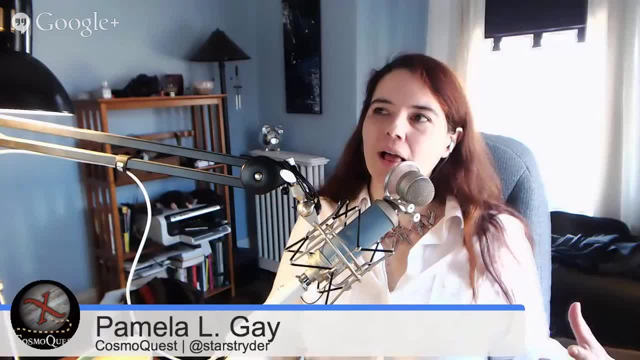 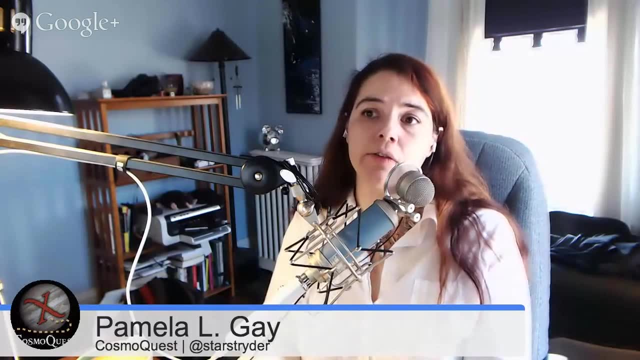 you start looking Like the sun or like Jupiter, like would that? Well, there you're even getting into completely more different science. So we start talking about, with galaxies, what's called surface brightness, where you start, instead of talking about what is the total brightness of the object, you start talking. 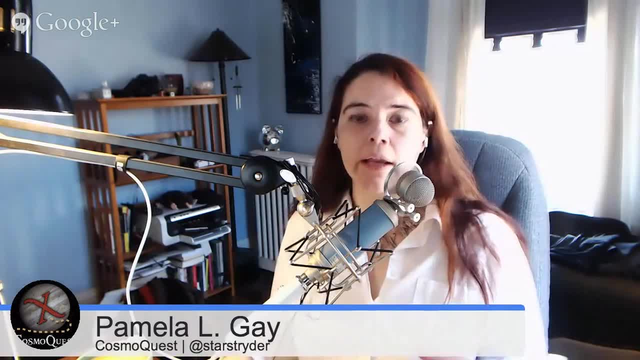 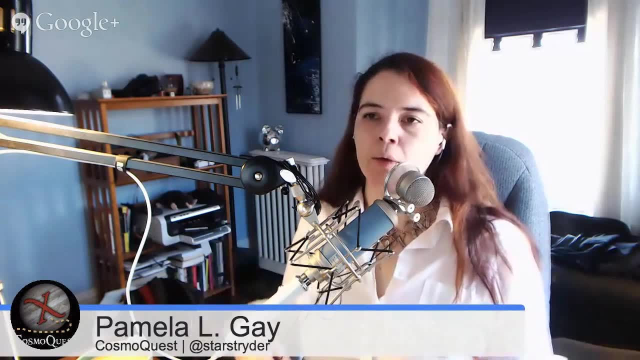 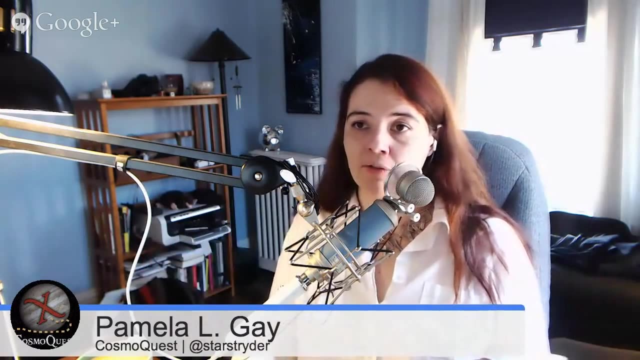 about what is the brightness per arc second on the sky. You start talking about What is the. Then you turn this around with math. and what is the luminosity per unit of volume or unit of area, because you can't actually get it? volume, unit of area on the sky of what you're. 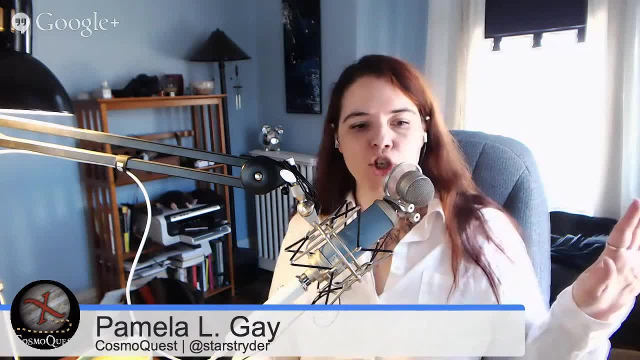 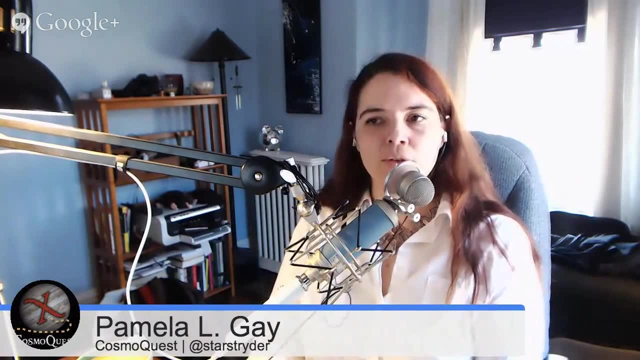 looking at- And in this case you're looking at a changing box, car average. draw a box, move the box around, see how much light is inside the box. It's a different type of technique, but the detectors that you use for 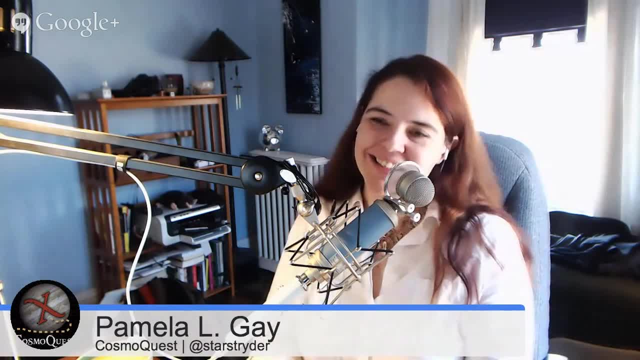 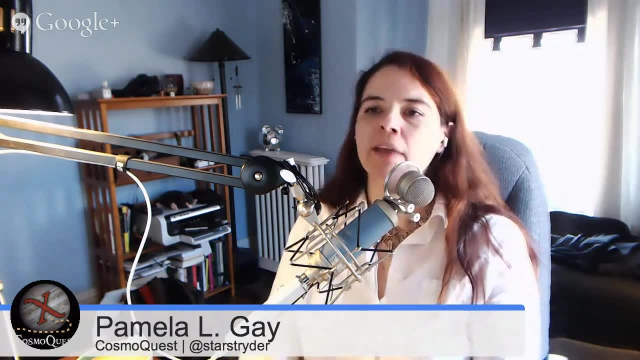 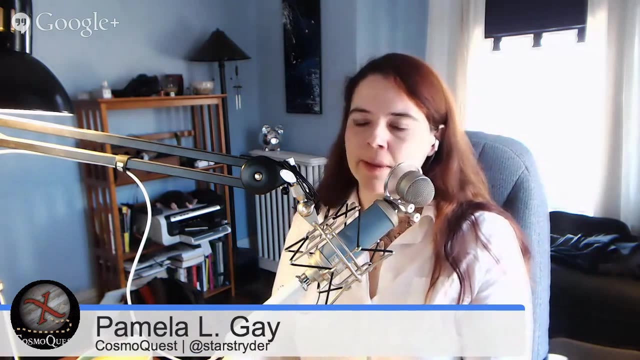 For doing photometry on a whole bunch of little tiny things, a CCD you can also use to do surface photometry instead of aperture photometry and start getting at that surface brightness profiling. start looking for dust lanes, star forming regions. how does nebulosity vary? 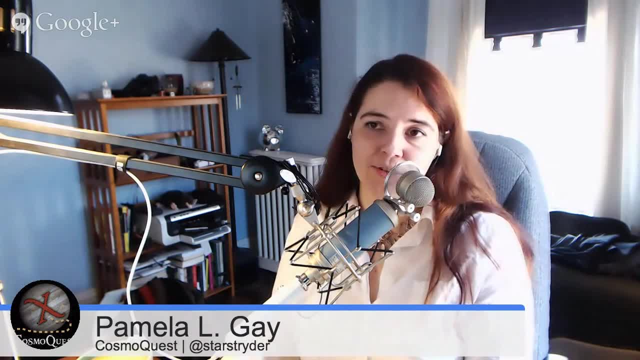 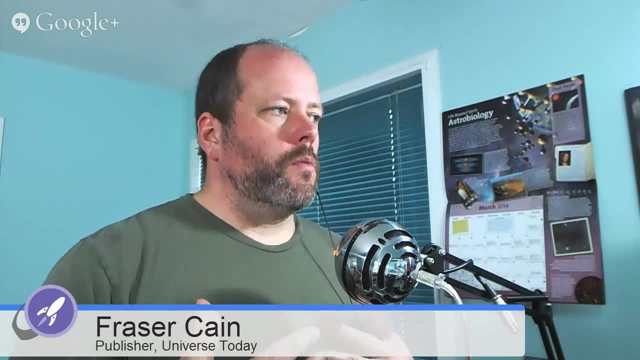 It all comes down to how much light and what color. That's astronomy. So I want to talk about some of the kinds of research that we'd be wanting to do. I mean, you've talked a bit about it, Yeah, At the highlights, but what are some of the different kinds of observations? the kinds? 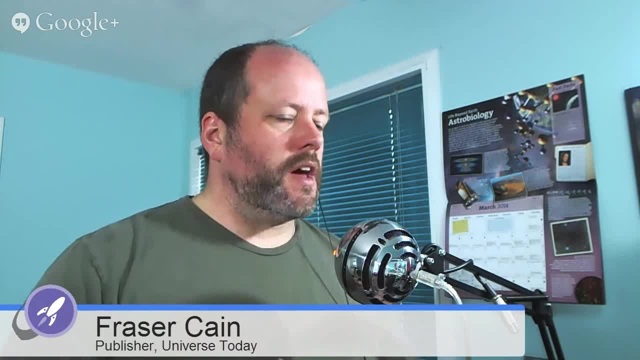 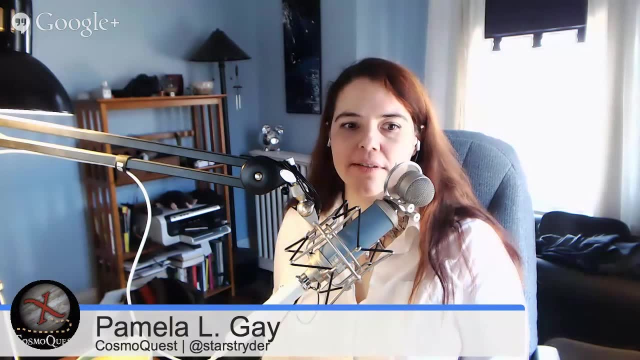 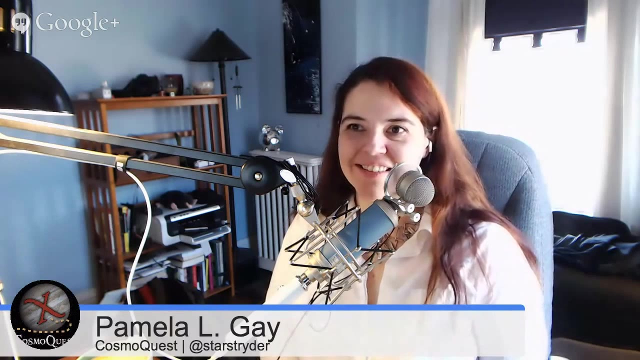 of answers we're looking for. and then what would our setup kind of be like? Like, for example, finding extrasolar planets, right? Well, what's kind of awesome is the setup is the same and the technique is the same for all of the science cases. So your setup is: you need a device chargeable. 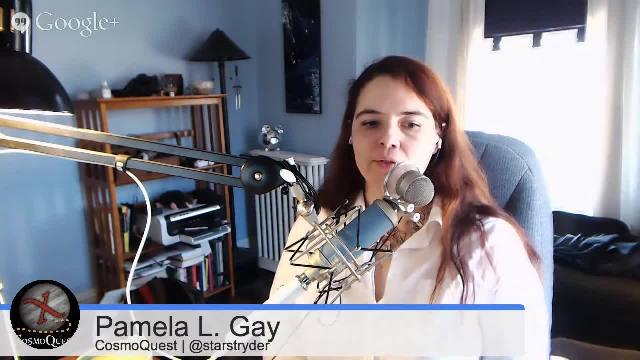 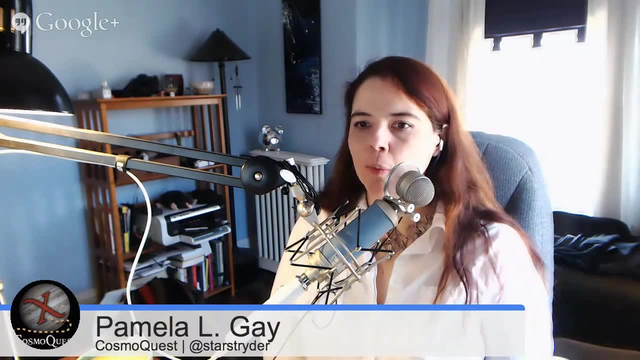 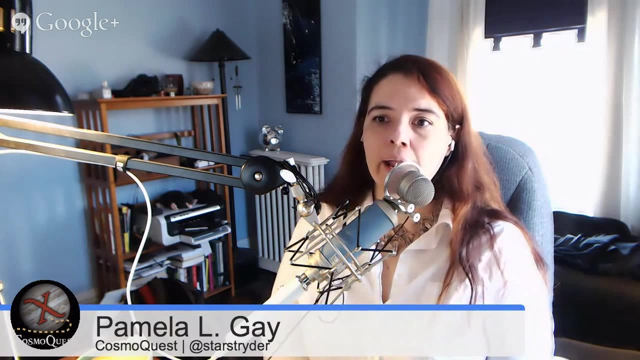 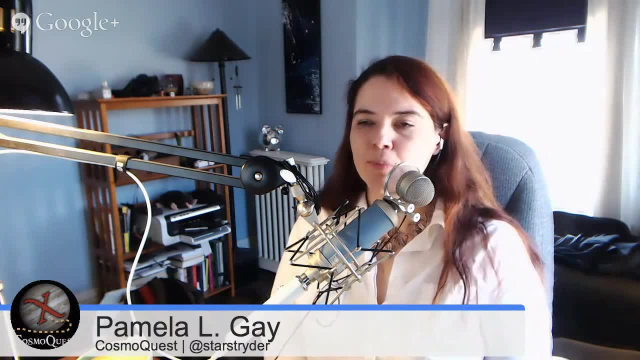 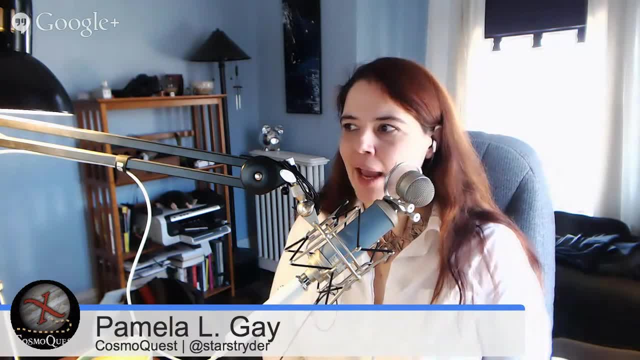 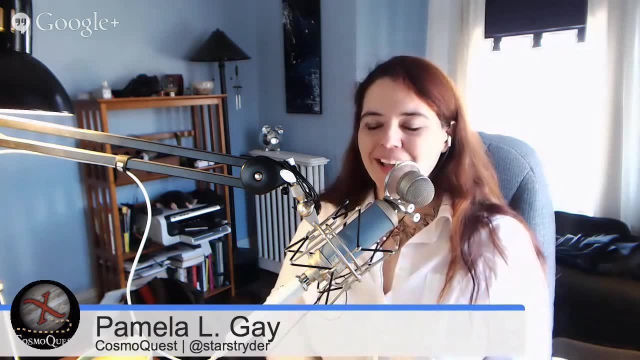 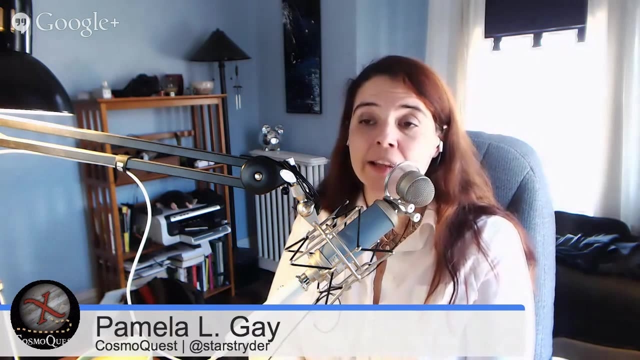 What you do pretty much runs the gambling. I'll start at the Sun and move my way out. People who do solar photometry. depending on exactly how they're set up, they can actually start to measure astrosismology, heliostismology. they can look for tremors, pulsations mode. 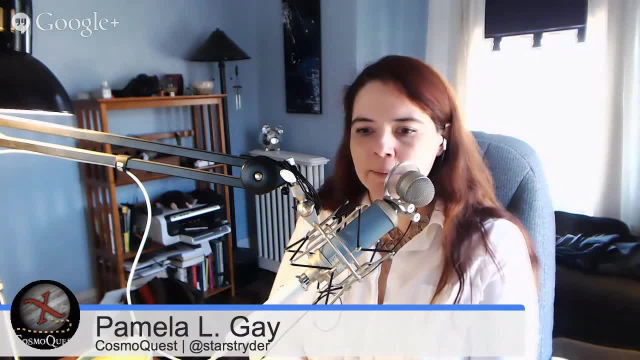 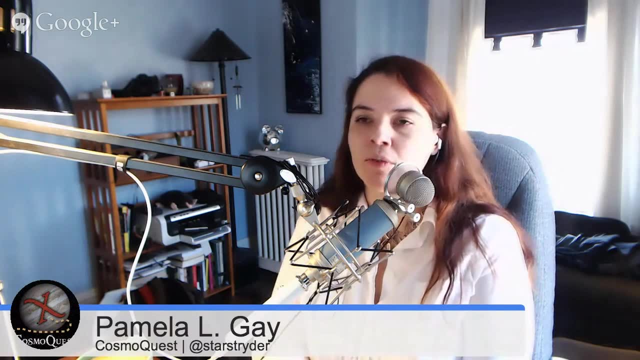 set up in the surface of our sun, moving outwards as we start to look at asteroids, near-Earth objects, small chunks of stone moving through the solar system when they pass in front of stars. if we observe them from multiple points on the surface of the Earth, the timing 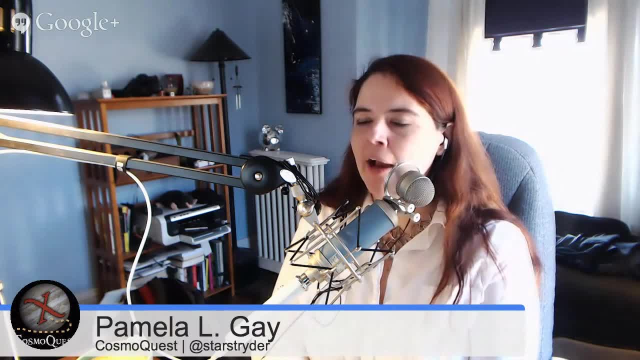 of how they block out the light from that background star will start to tell us the shape and more information on the position of that rock moving through the solar system. If we simply look at the reflected light coming off of an asteroid, we can start to get at. 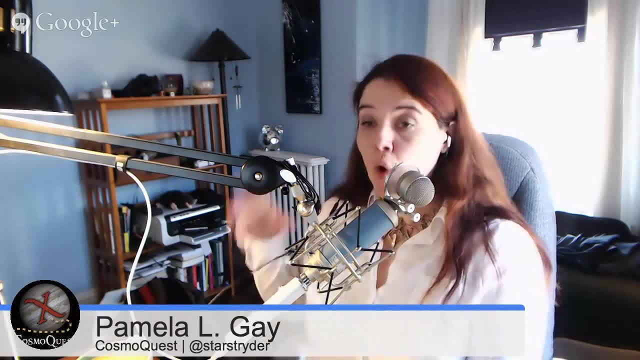 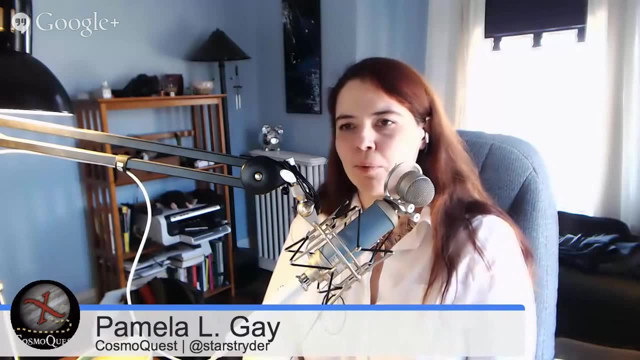 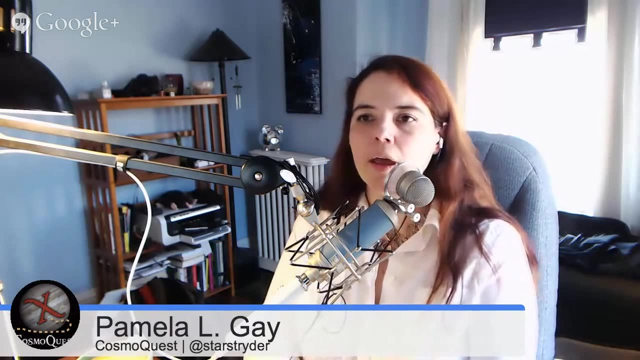 changes in its shape as more of it is facing, less of it is facing As we move out. you can take pretty pictures. You start doing surface photometry of planets. That's different. That's pretty pictures. Use a box, Measure what's in the box. 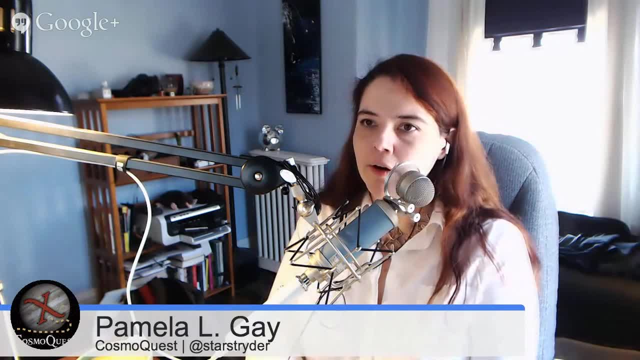 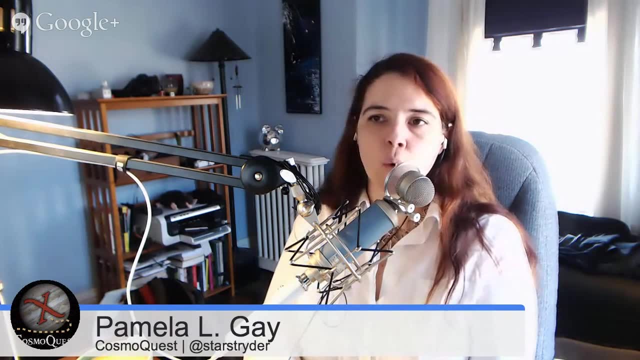 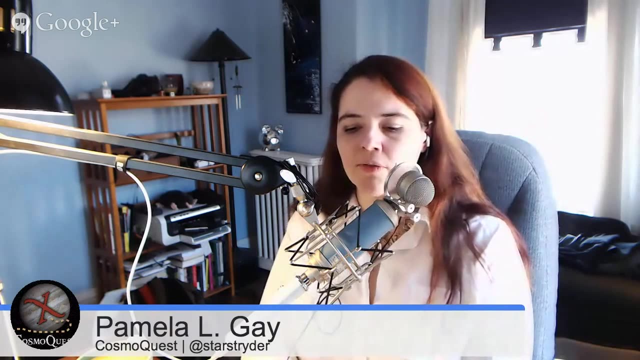 But then as we move out and continue to move further, when you start looking at stars, you can look for flares, You can look for pulsation modes. that means this is this type of star that has this sort of. they're actually what are called harmonic oscillations. 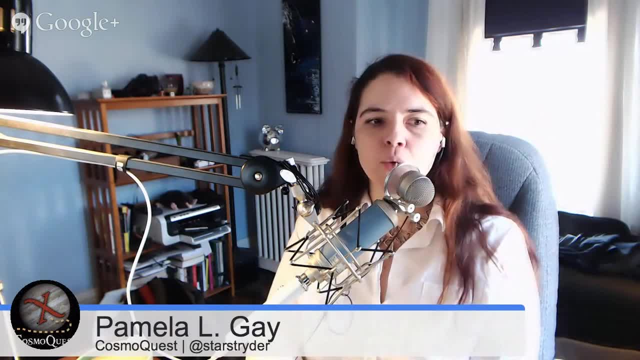 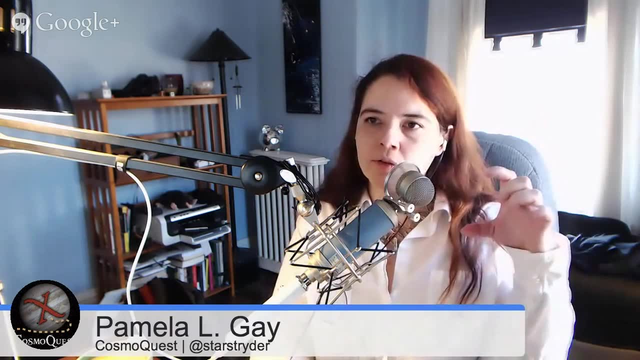 These are just like when you blow into a bottle and it vibrates at a set noise. You blow harder, it blows at a different set noise And there's no vibration. There's no noise in between those two you can get. Well, stars pulsate the same way. 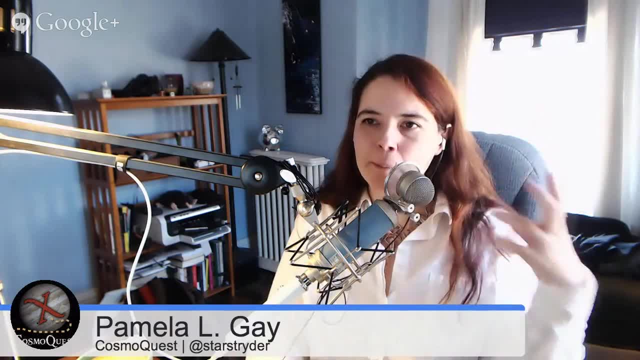 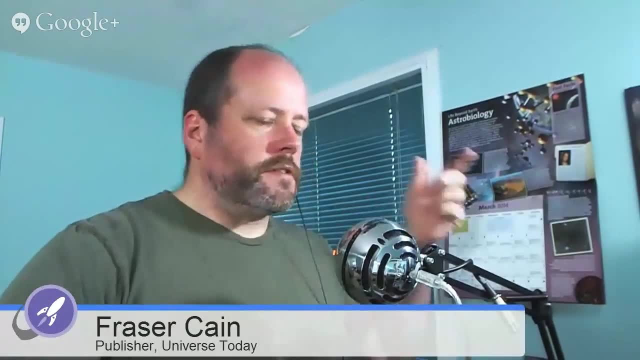 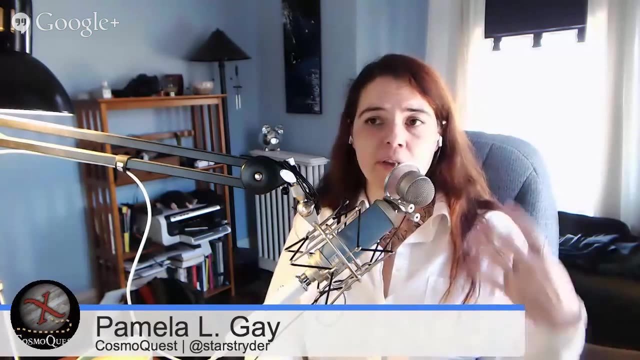 They have allowed frequencies, And what pulsation modes you get depends on the composition, the age, the size of the star, So you can measure the pulsation and then that tells you some of those other variables that you're interested in, And over very long periods of time. and this was the first research I actually started. doing. you can look at some of these stars and look for changes in their pulsation And as you measure these changes in periods- and this was one of my first papers that I did- as you look for these changes in periods you can actually start to get at the density. 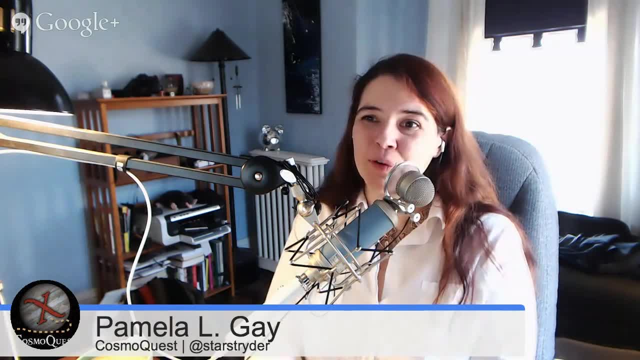 changes that are going on inside these stars, And we've been studying variable stars for so long that there's now measurable changes. Wow, That's really cool, Yeah, And so that tells you other things about even more refinements on what's going on. 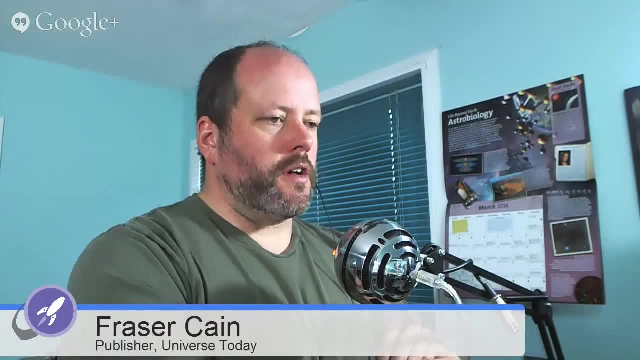 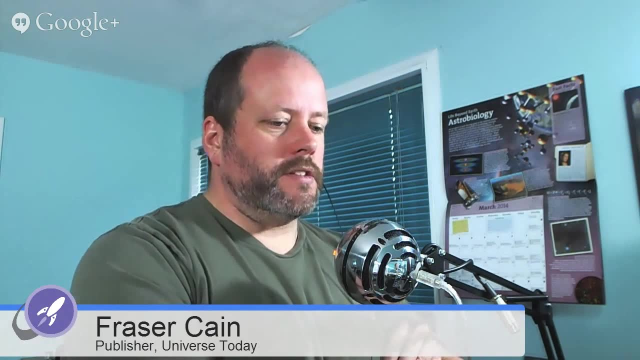 Stellar evolution modes? Yeah, Star models. What's going on with the star? Yeah, Exactly. I mean you think about all of these events. I mean I know, like what would be the absolute holy grail would be to see, for example, a. 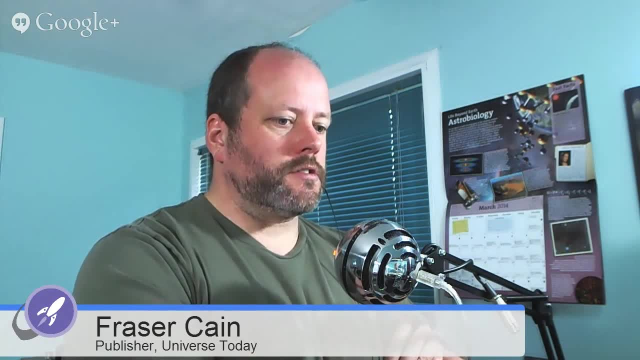 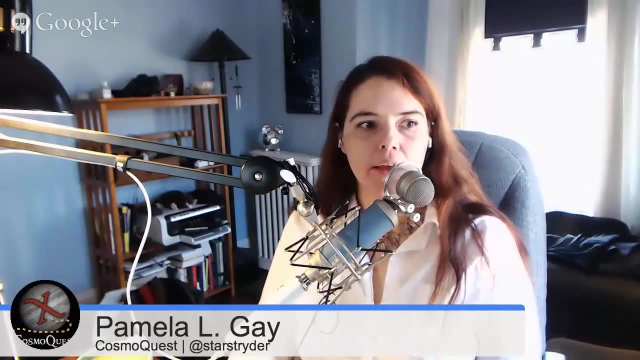 supernova precursor and to be able to watch changes in brightness weeks before it actually detonates. I mean that would just be the greatest thing ever. right To see a supernova precursor right before it goes. That's all cool, But what I think is just as cool is: 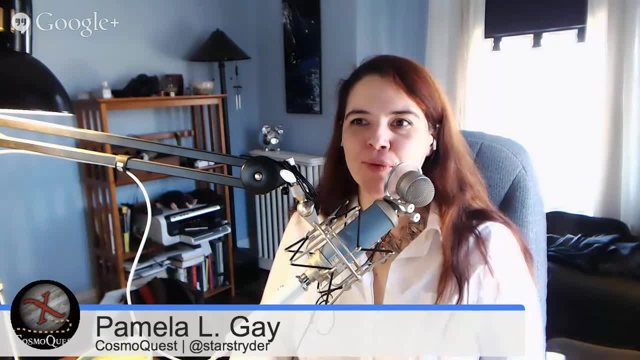 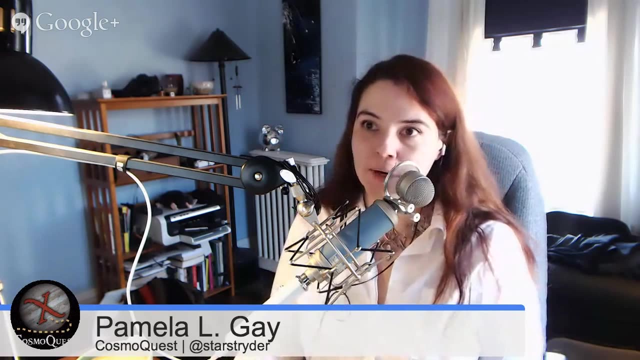 What about those moments right before a star goes from main sequence to spending a couple thousand years becoming a red giant? That death to a main sequence star is the next thing our planet's going to have the joy and death of experiencing, And so there's so many other stages out there. 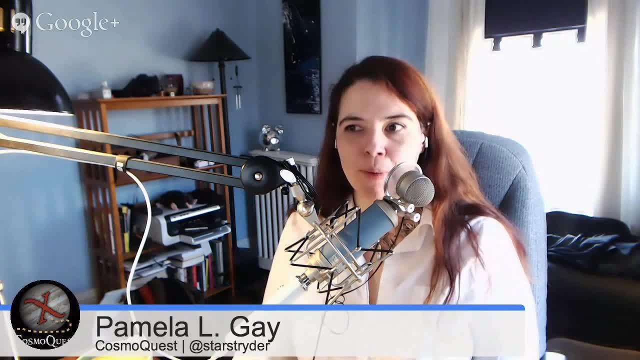 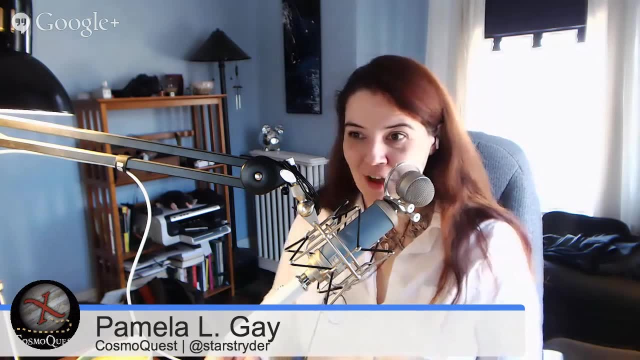 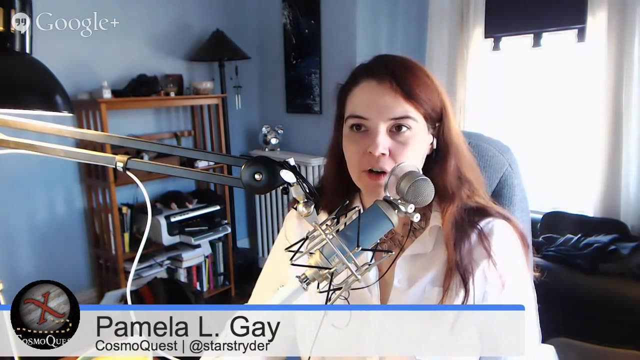 And what's kind of awesome with variable stars is? we've been able to now and thenmy favorite one is variable stars And my dog has decided I'm not giving her the leftover Chinese. Sorry, Preston, for the dog noises in the background As we watch all these different stars over time. with more and more surveys we're going. 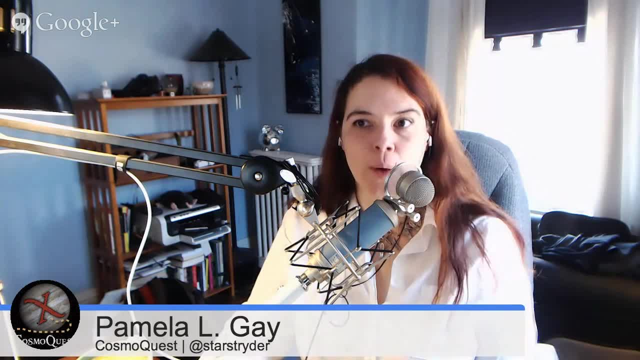 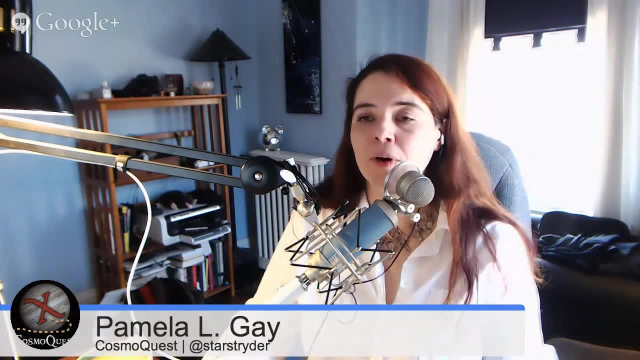 to start catching stars, going from main sequence to red giant branch, moving on and off the horizontal branch, And we see variable stars change modes periodically, showing us their steps through the evolution. Yeah, Yeah, And it's a lot of revolutionary trails, Yeah. 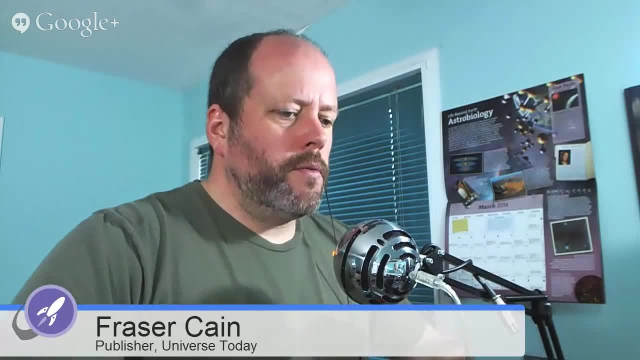 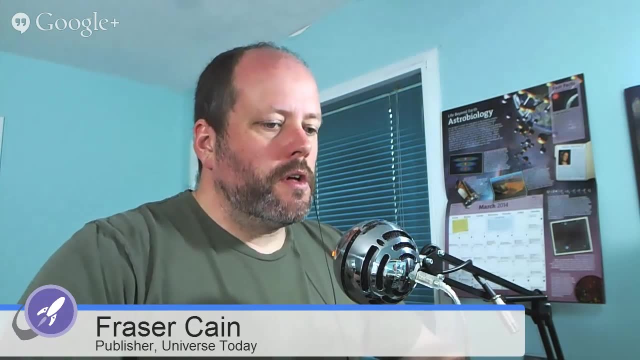 I wonder if Gaiais Gaia going to be able to help out with this at all, Like it's going to be doing really precise measurements of the positions of the stars, But I wonder, And very precise photometry Part of it is getting- 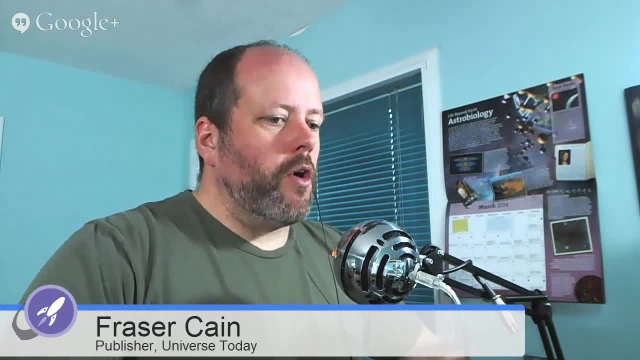 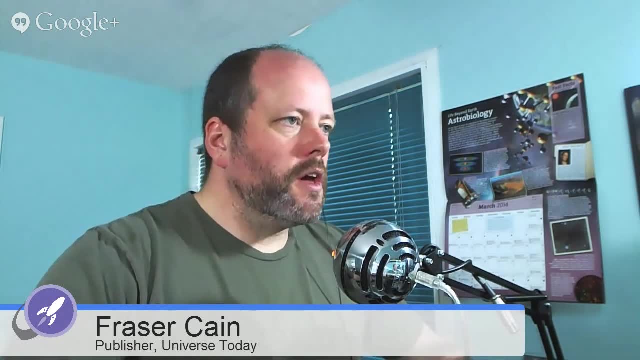 Yeah, I wonder if it's going to start to pick up some of theseyou know, if you look at 1% of all the stars in the entire galaxy and watch for changes in brightness and you've got some of these events that you're looking for, chances are you'll catch some of these. 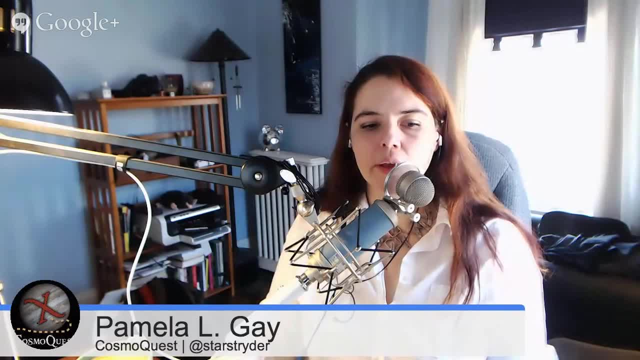 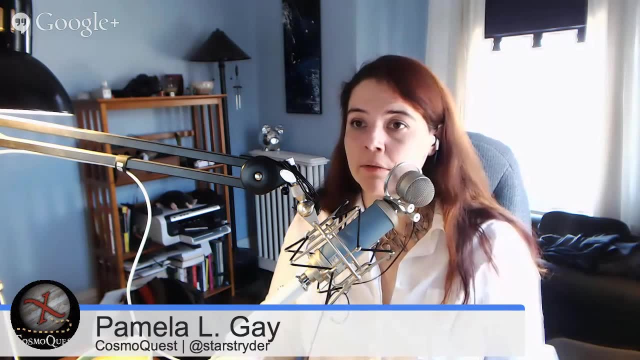 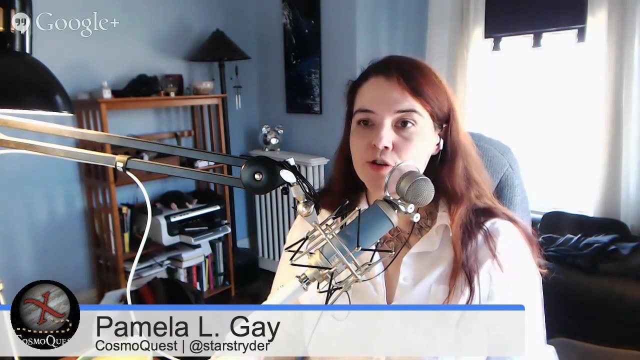 Well, There are two things that you need to worry about. One is getting precise enough data, And with Kepler, we had the most precise data that has ever been accumulated, And people who do variable star work basically have a treasure trove that it's going to take. us a long time to sort out. Now, unfortunately, stars that Kepler realized were variable stars didn't get observed for the whole duration of the mission because those weren't prime targets for finding planets. But there's still some really amazing stuff in there, So getting the amazing data is part of it. 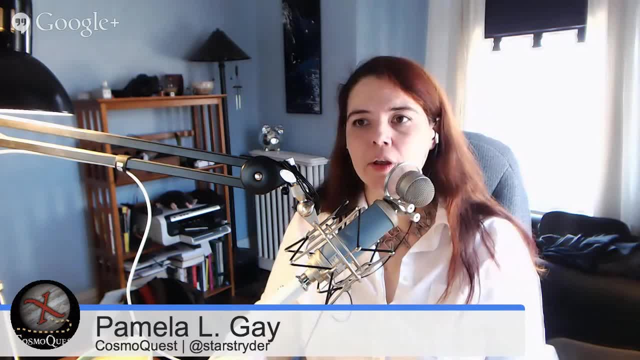 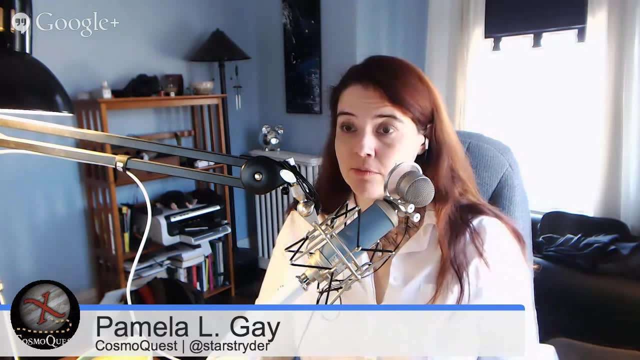 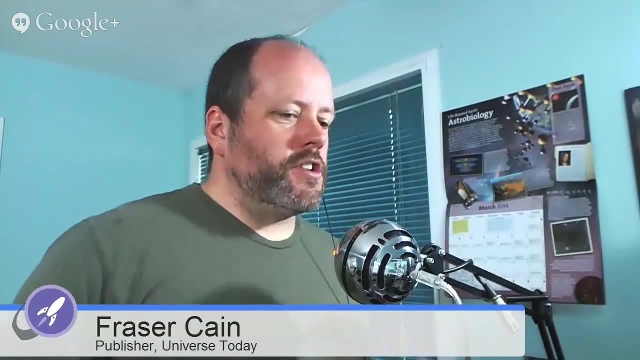 Part of it is getting data long enough. Variable stars are changing periods over a hundred plus years, And we have a hundred plus years of data from the ground but not from the sky. So is Kepler like justlike, in addition to all of the work it's done in helping to? 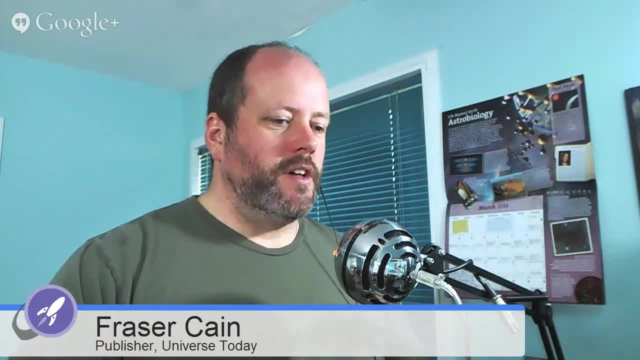 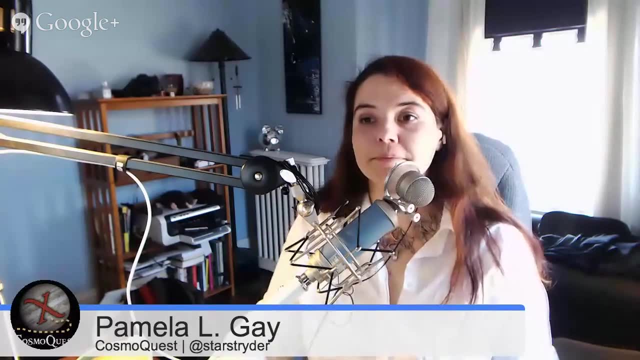 find all these planets? Is it just dumped out mountains and mountains of data? Yeah, There's all these kinds of garbage data for Kepler, which is like, oh yeah, the variable star. astronomers are just like digging through the trash. All of this like, oh, you know what? it's a variable star that no one's ever heard of. 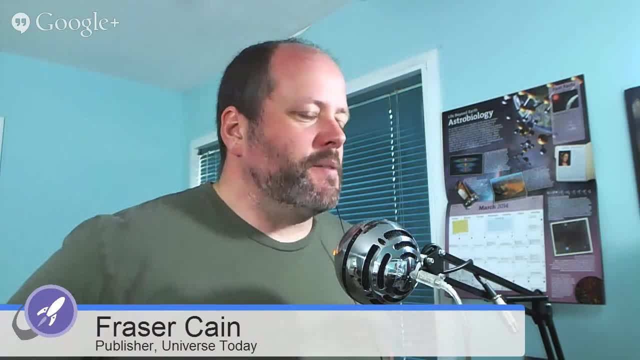 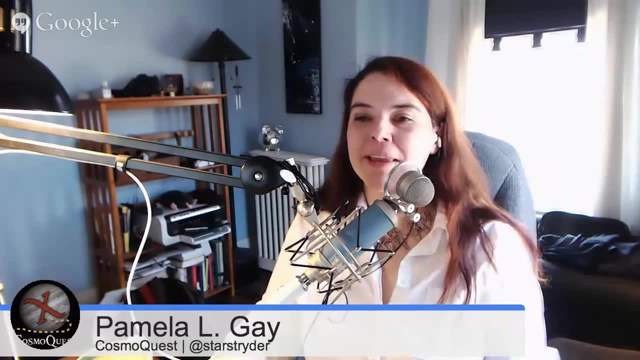 but it's not interesting to us, so you guys can have it if you want. Yeah, I can just imagine how much of a treasure trove that is for the variable star astronomers, because you have to look at so many objects. What gets me is a lot of people are like: yeah, we don't care about variable stars. 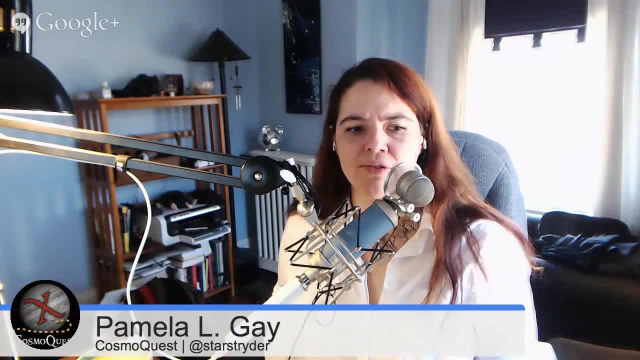 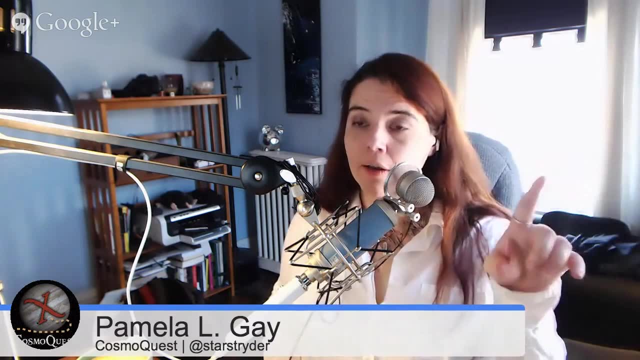 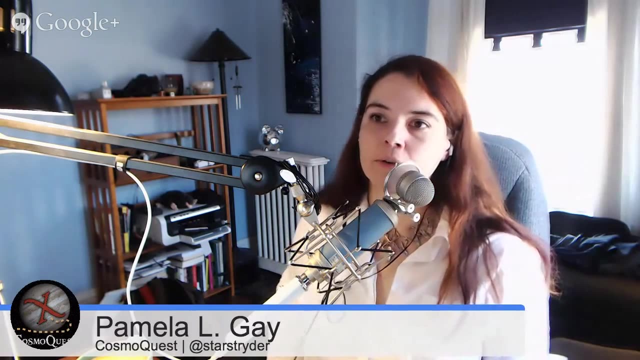 But variable stars are what start to put the fine constraints on our stellar evolution. They're like: no, you didn't explain me. I'm doing this thing over here And so, while a lot of people who admittedly need money and grad students and stuff will, 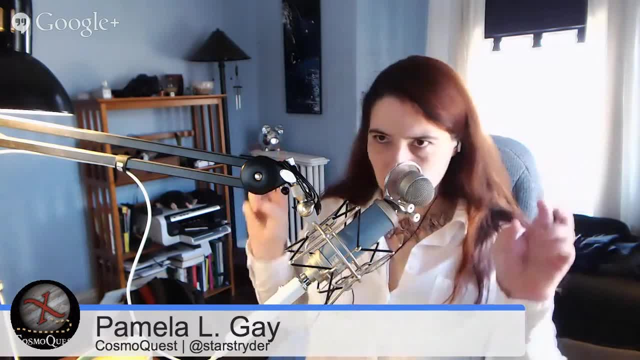 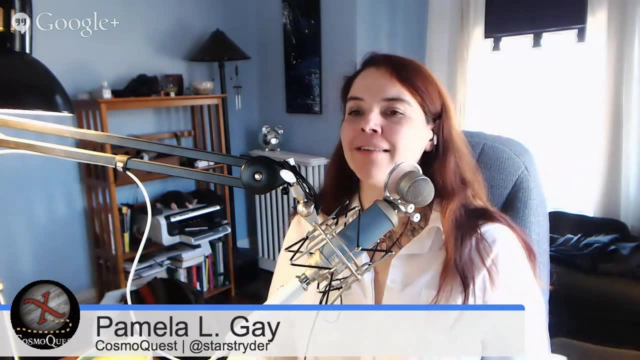 just ignore the variable star data because they're deemed a solved problem because we know the basics. there's a whole lot of data that it's not as desperately sought after. Okay, so you were moving out. You got to variable stars. Yes, I got to stars. 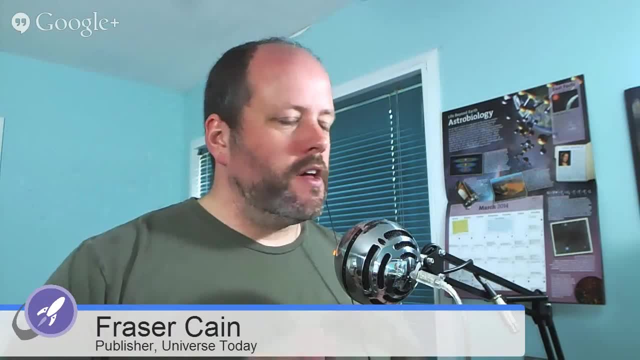 You're finding planets. I keep saying planets. I don't know why you keep avoiding planets. No, I just hadn't got there yet. You've done it again. You're not interested in planets at all, are you? No, I hadn't got there yet. 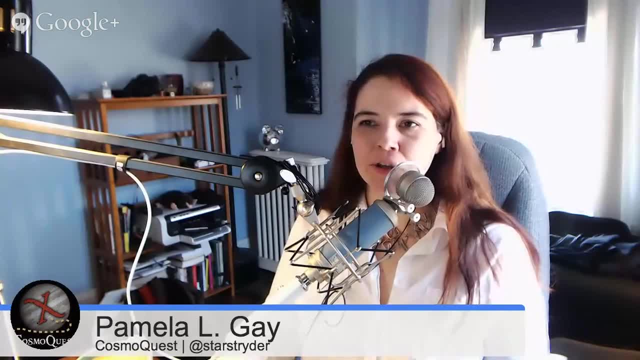 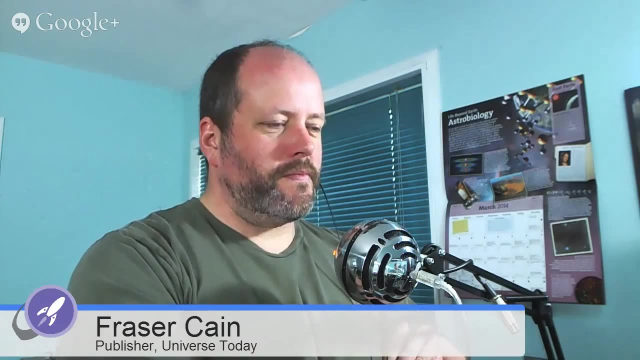 Okay, Pulsars. So pulsars, you can notice them in radio photometry. basically, It's not all about the optical light, It's all about the stable, precise setup. Yes, you can find planets, You can find binary stars. 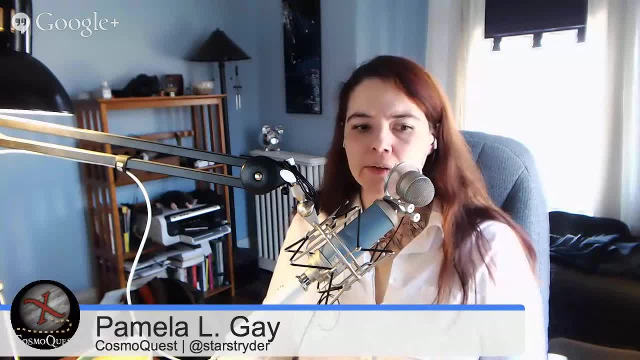 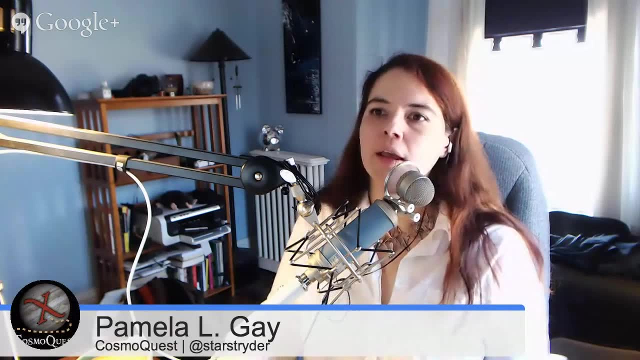 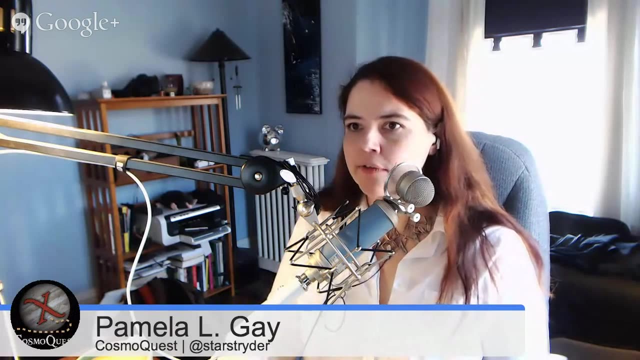 Thank you, And then you can start looking at really neat physics. So there's systems with small, compact stars, white dwarfs, neutron stars- sitting next to a companion star that they're cannibalistically sucking material off of, And those accretion disks of material that build up around them will vary in brightness. 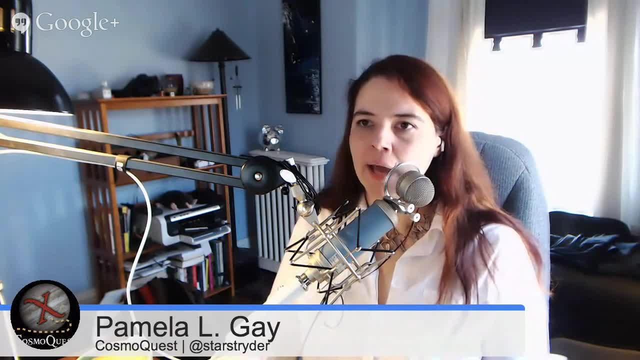 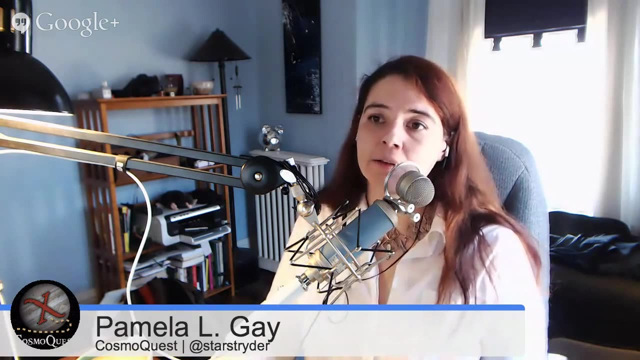 And so, as we watch, those vary in brightness and periodically undergo radical explosions and things like that- Okay, That's photometry. Same physics applies to the accretion disks around black holes and galaxies, So we end up with active galaxies that flicker and you can actually map out the cores of. 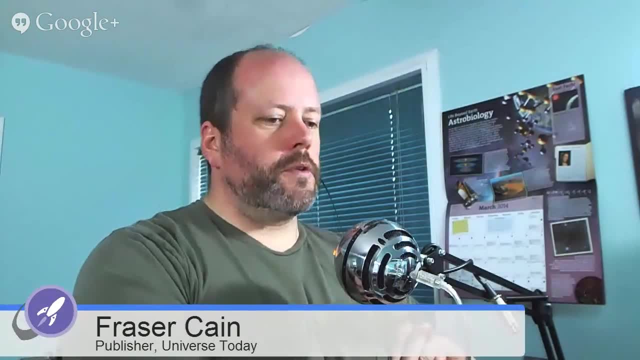 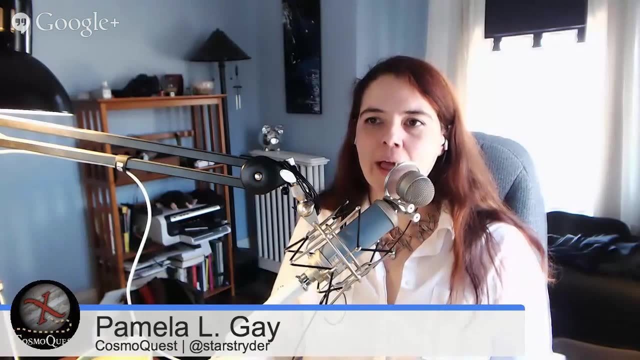 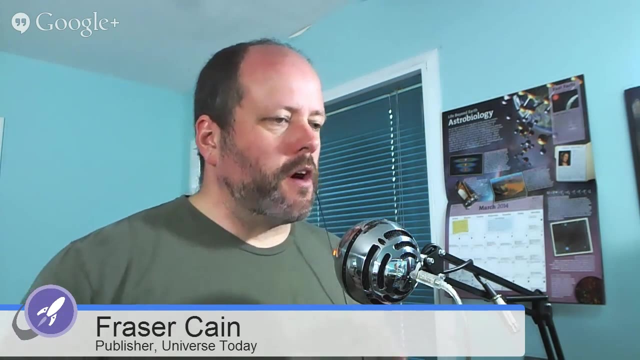 the galaxies using photometry. Light curves of supernova. Light curves of supernovae- Yeah, it's a whole lot of physics going on. Is there any sort of value? even beyond that, Is anything done with the cosmic microwave background radiation? 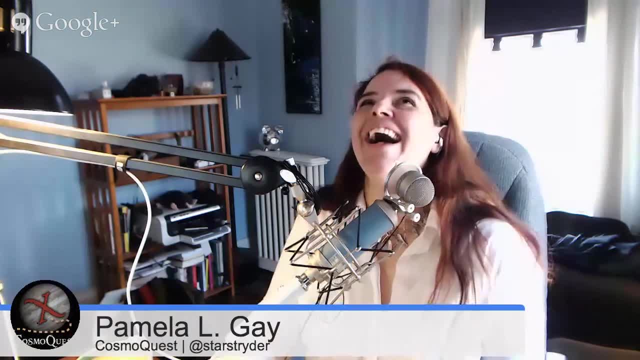 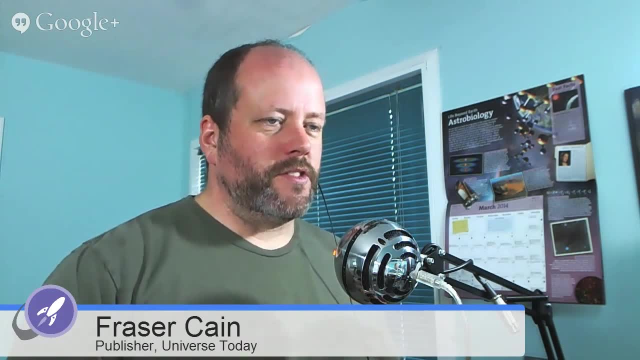 Because we know that it's used for everything There. I don't think you call it photometry anymore. Okay, All right, But there's no point gazing at one spot in the cosmic microwave background and just watching for any changes. Yeah, no. 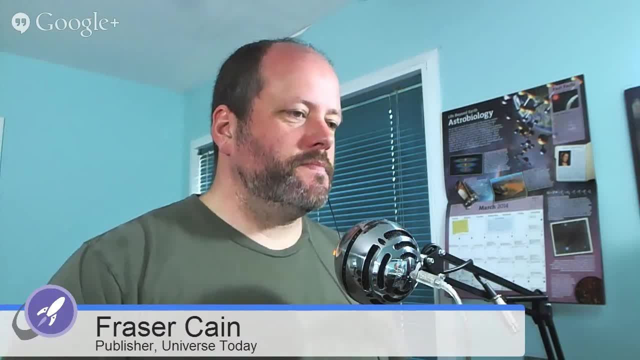 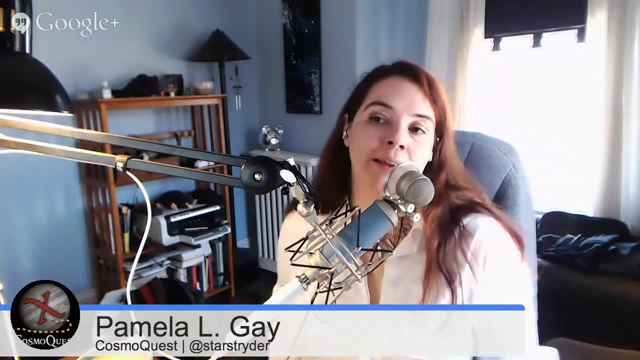 That's it. We've reached the limits With James Webb Space Telescope. Yeah, With James Webb Space Telescope, we'll be able to start doing photometry on the first time. Yeah, We'll be able to do photometry on the first stars and galaxies forming in the early universe. 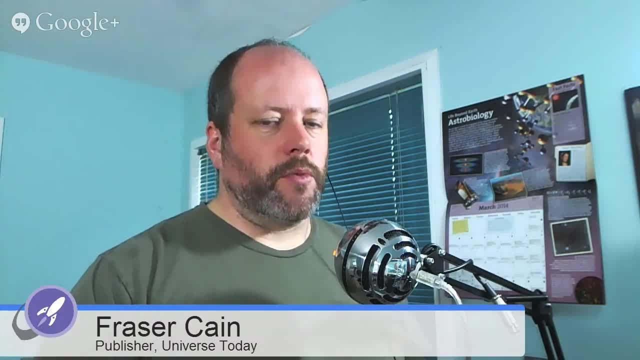 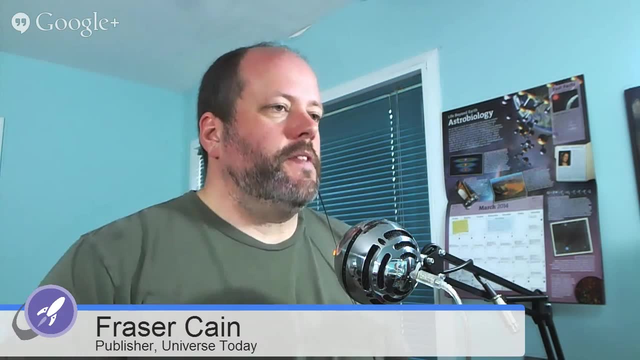 That is going to be mind-bending. Yes, Yeah, That telescope. when it comes online, it is going to change everything. We just went through the big NASA 2015 budget and I know everything you love was destroyed. There's going to be no salaries left. 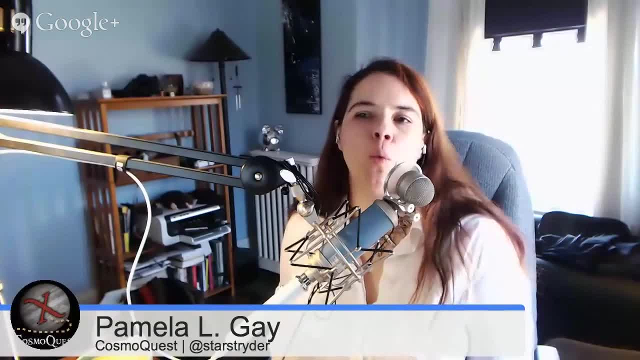 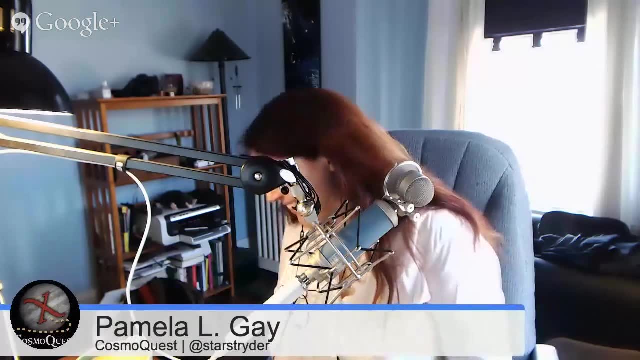 We're going to have the most amazing telescopes out there and no one working in astronomy. Now I don't know if you've heard- I have volunteered the resources of Canada to help take over some of the maintenance of some of those projects. like I don't know, Cassini. 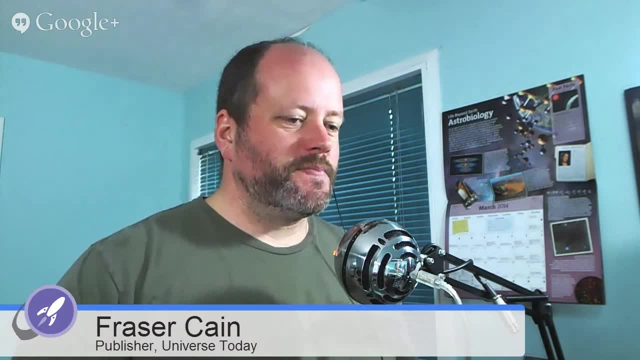 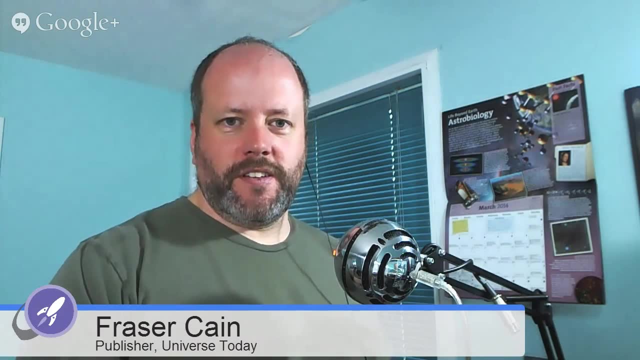 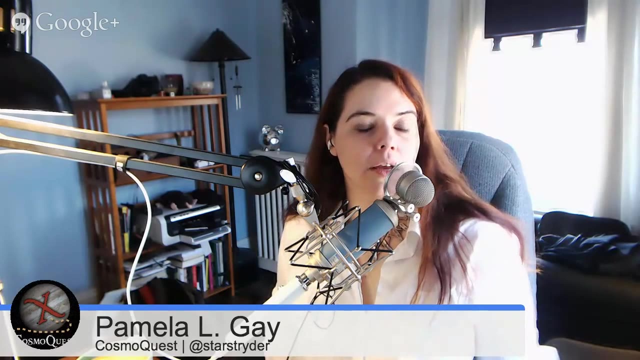 SOFIA. Anyway, well, thank you very much, Pamela. My pleasure. I had way too much caffeine, Not enough caffeine Saving- Yeah, Okay. Do you have time for questions or are you running to the airport? Yeah, Yeah. 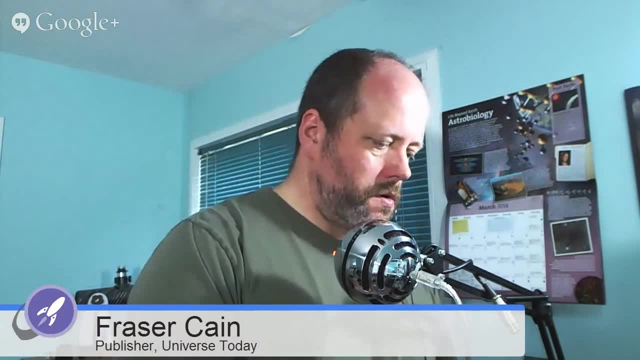 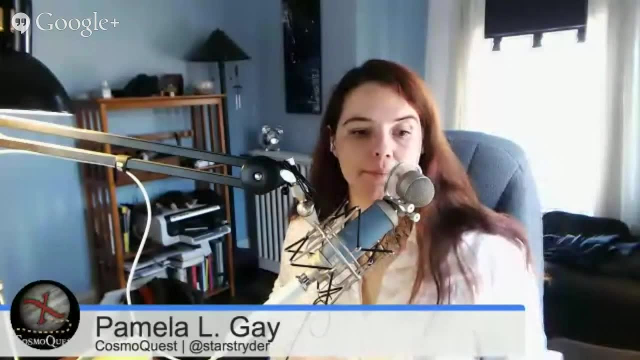 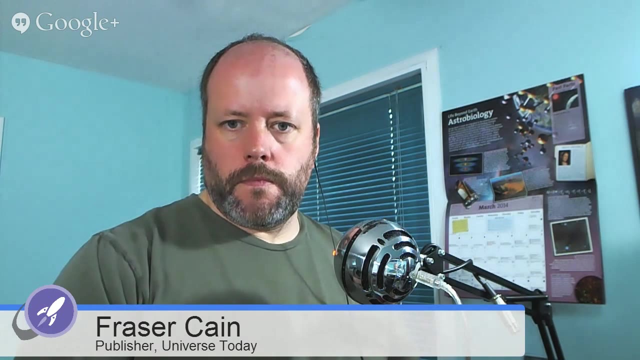 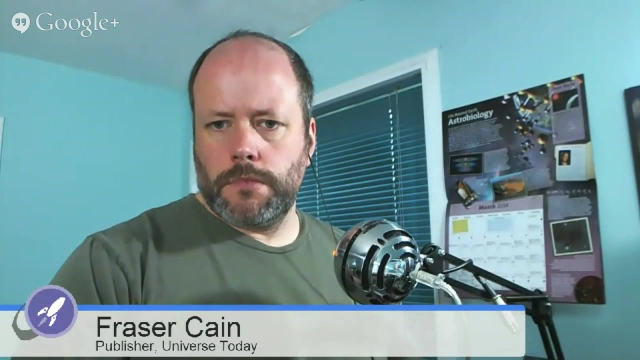 Yeah, Yeah, Yeah, Yeah, Yeah, Let's go for. what is it now? 1240,? let's go for. yeah, we'll go for 10 minutes. Okay, Just save. Okay, Everything is nice and safe. 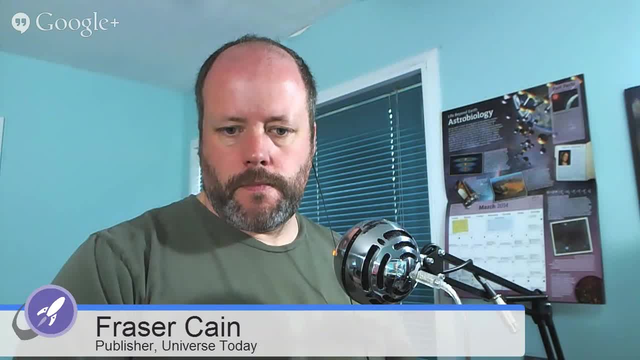 And uploading. John Yeager wants to know: how did you become so smart, Pamela? The questions you are seeking are so incredible. I really love the way you're explaining this. Pamela, how did you become so smart? I don't have a single athletic bone in my body, so books were the only option. 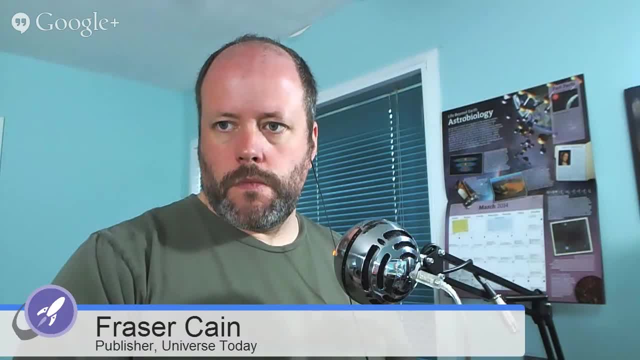 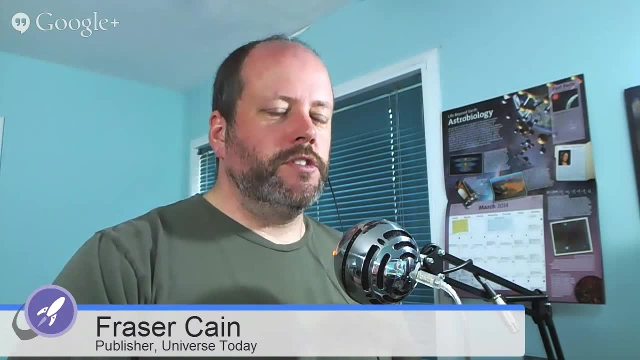 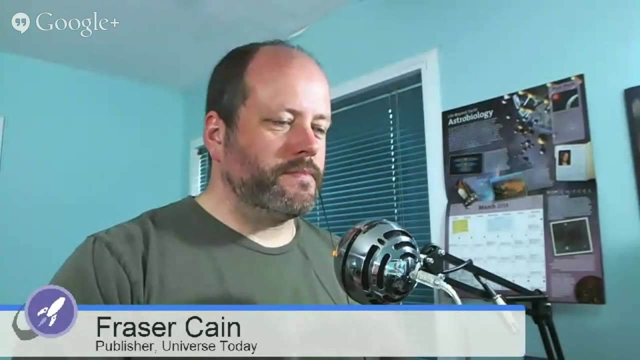 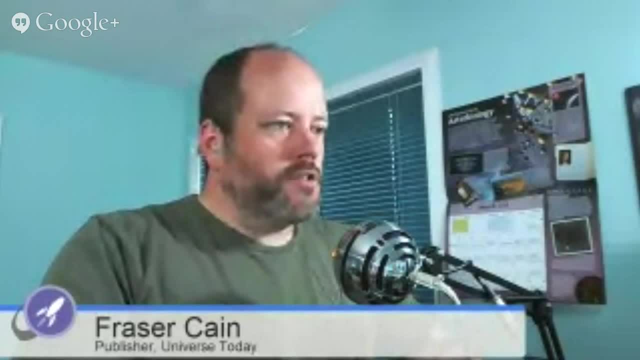 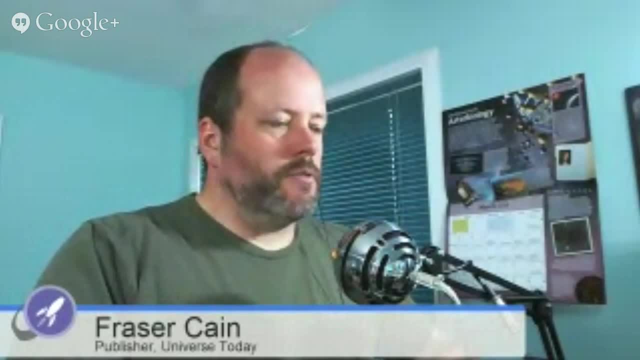 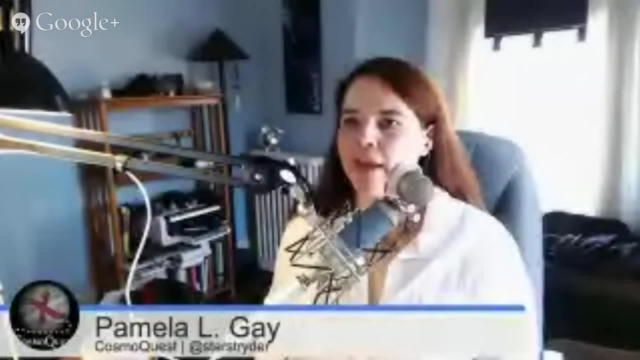 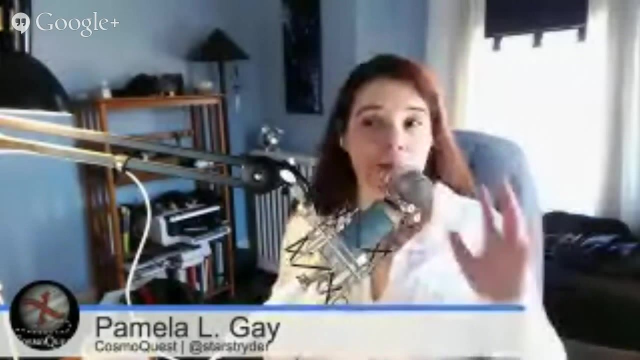 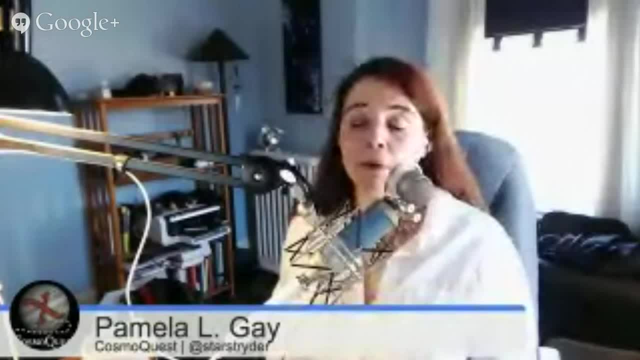 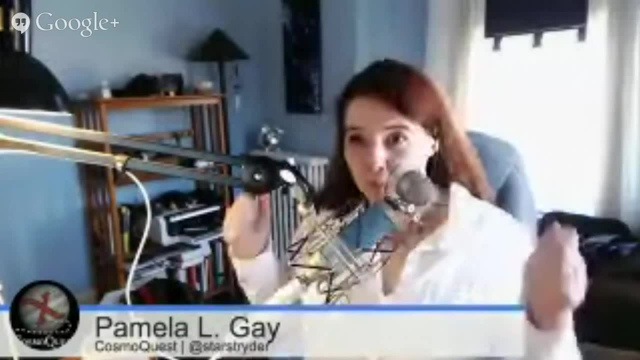 Yeah, Yeah, Yeah, Yeah. summer to raise money for the library and at least when I was growing up, the last day of the sale it was a buck for one of those brown paper grocery bags of books. Wow, Yeah, And so heaven. 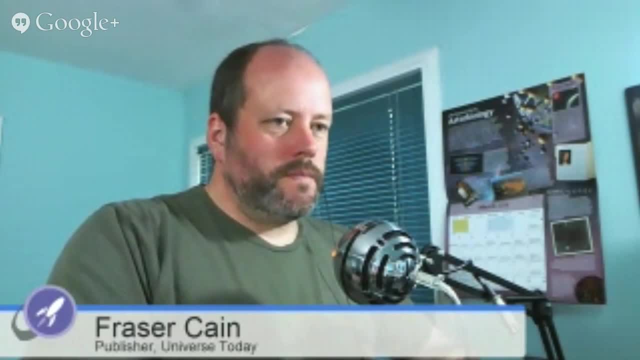 Well, not anymore, because I hate atoms, So I don't like to own anything physical anymore. Yeah, Okay. Anish says: how does a black hole seem to slow time down, Just like you got one minute? Whose perspective. 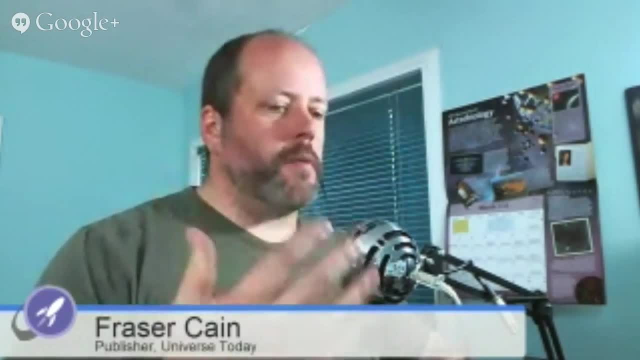 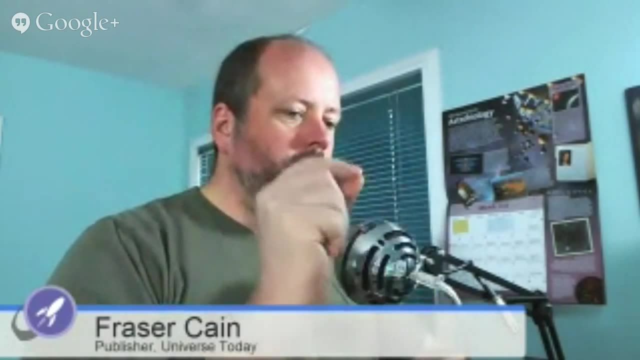 I guess from I guess you know the saying goes, or the thought experiment goes, that if you're watching your poor friend fall into the event horizon of a black hole, from your perspective their time slows down to the point that they are sort of. 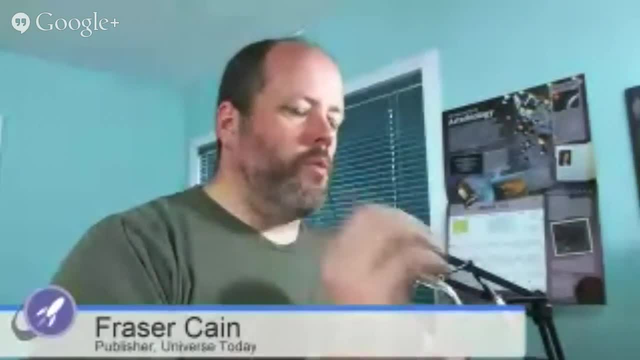 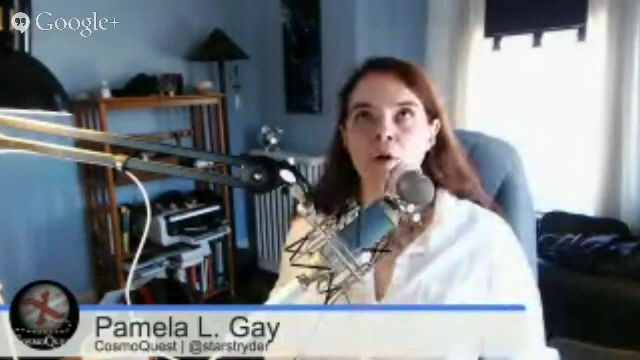 trapped on the surface of the black hole and then they're redshifted away and they just fade away, But you don't actually watch their horrible, painful death. The issue is that they're moving so fast that, in order for them to perceive the speed of light, at the same speed that you perceive it. their clock has to slow down And, pretty much from your perspective, stop, And so you don't actually see them die. What you see is them just get redshifted away as they fade away. 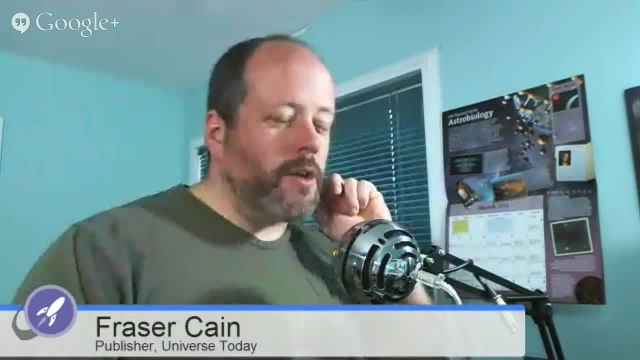 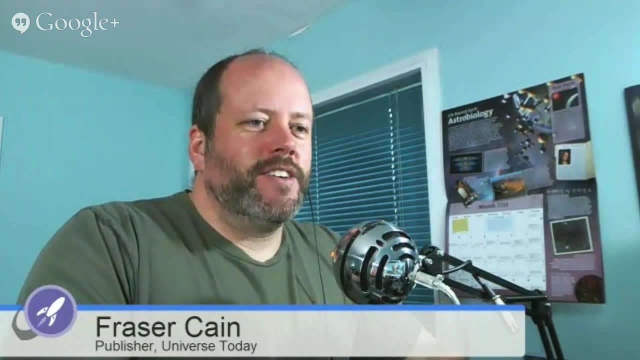 until the photons become radio And you're listening on the radio as they die. That's morbid, Isn't that wonderful? Yeah, No, I should give that to Sigler. He can turn that into a book. Our Strohsa says: 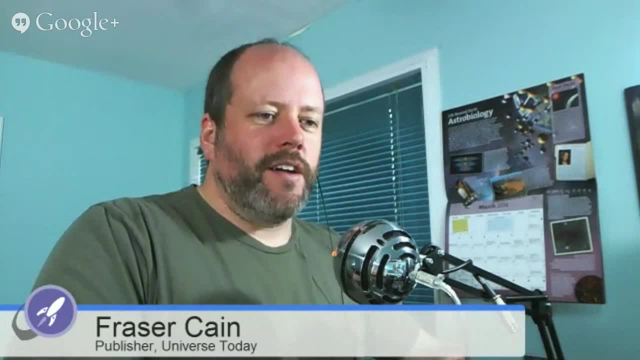 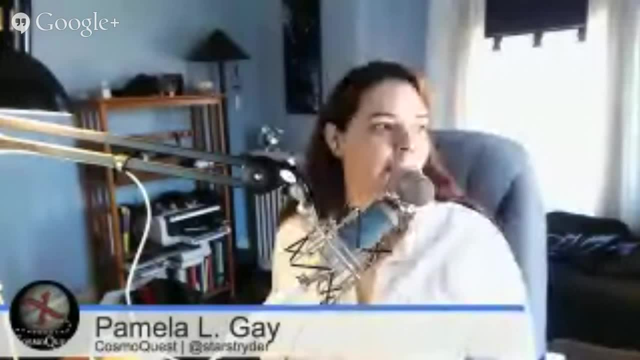 I do turn in every week for the discussions on plumbing. So yeah, I think that's what we do. Between your burst pipes and my leaky ceiling, we've had more water inside than we needed. Don't buy a house There, Alright. 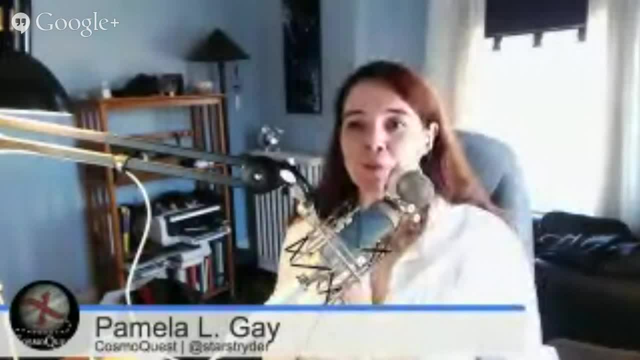 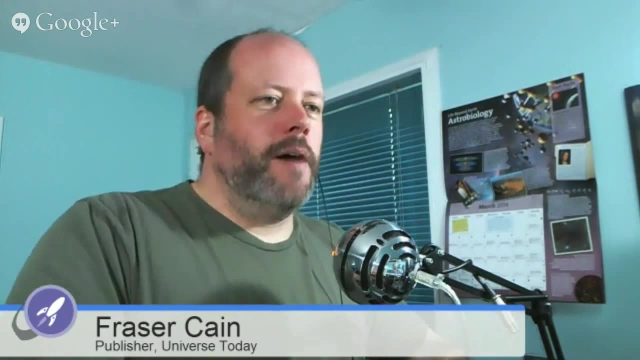 Don't buy a house Rent. The only advice I've ever received from Elon Musk was actually that, Yeah, I'm sure, What about rockets? Just don't buy a house. Okay, Yeah, actually Russell Bateman who gave us. 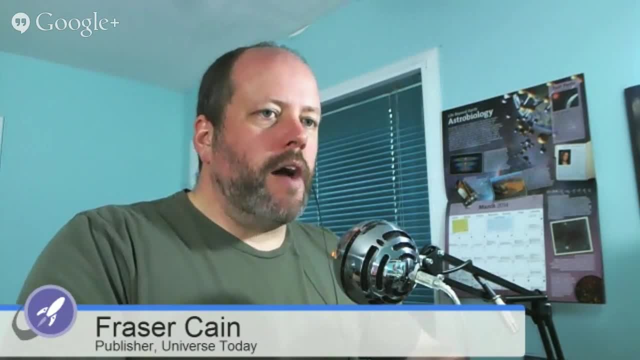 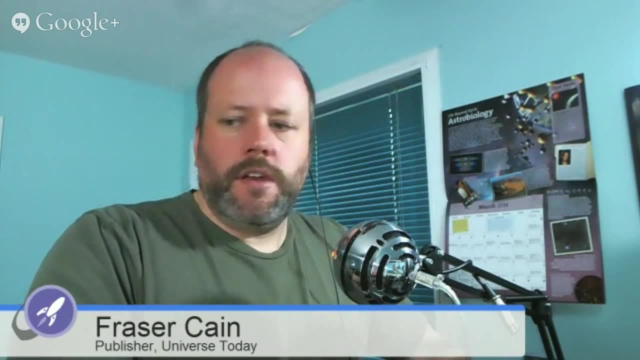 beautiful views of the moon last night in the virtual star party. I've always had an interest in photometry. What equipment and software is needed for a backyard amateur astronomer to do photometry? I guess we should have mentioned this- that amateurs do. 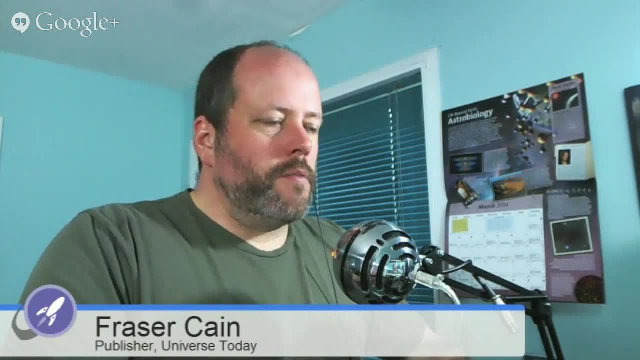 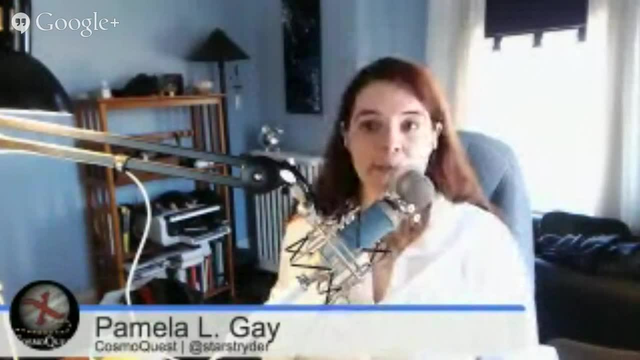 great work in photometry and the variable star observers depend on them. American Association of Variable Star Observers. you need a CCD, a telescope, a mount filters- Johnson or Cousins filters are kind of standard We're also now starting to use. 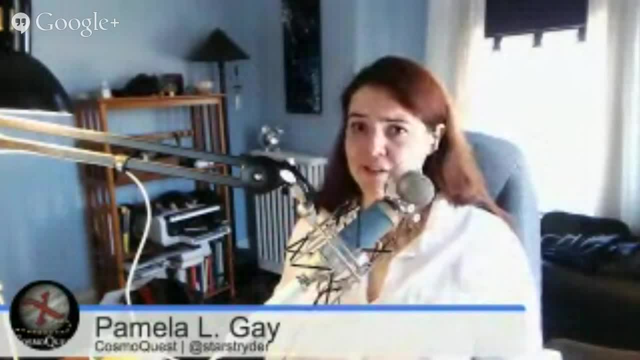 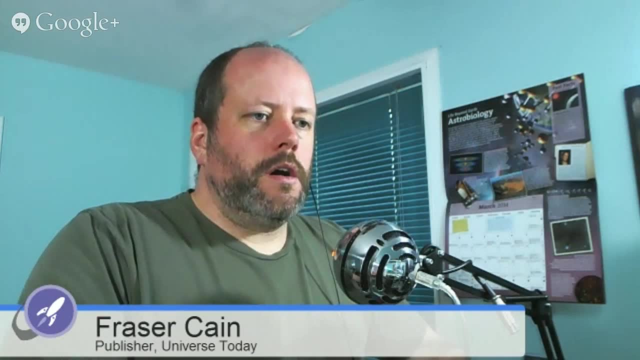 the Sloan filters And then just Maxim DL will get you there, or Apes for Win or, if you really hate yourself, IRAF, CCD soft. Those are software packages. Reiko Prozo asks: is it possible to take x-ray images? 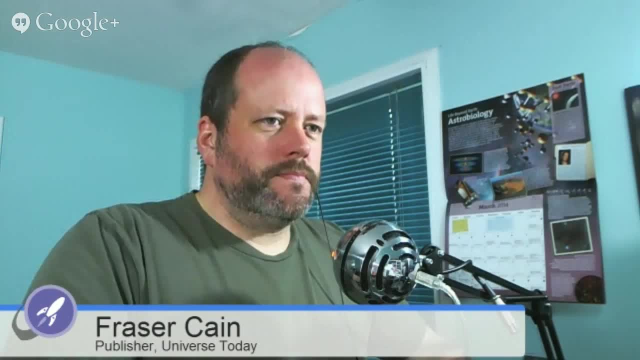 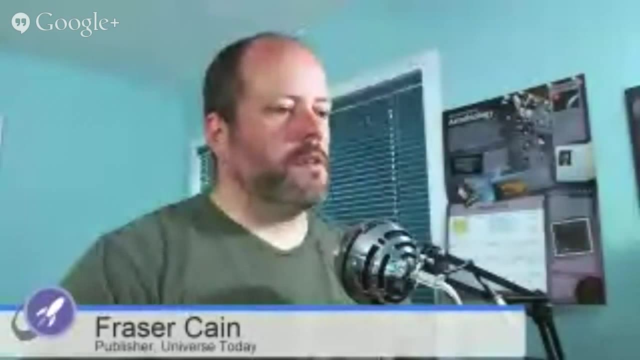 using amateur astronomy equipment. No Atmosphere- Yeah. so it's not even possible for super professionals to take x-ray images, because the atmosphere You need to use a sounding rocket, Yeah. so what about when we launch our amateur telescopes, our amateur space? 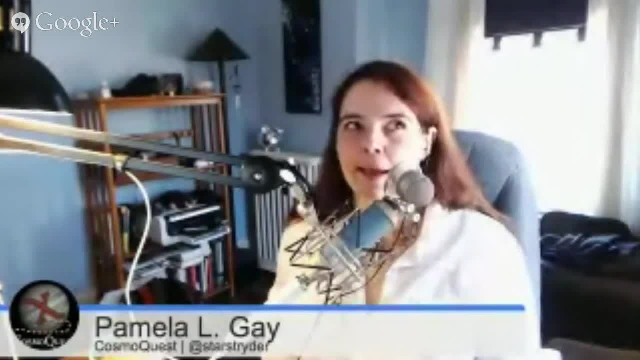 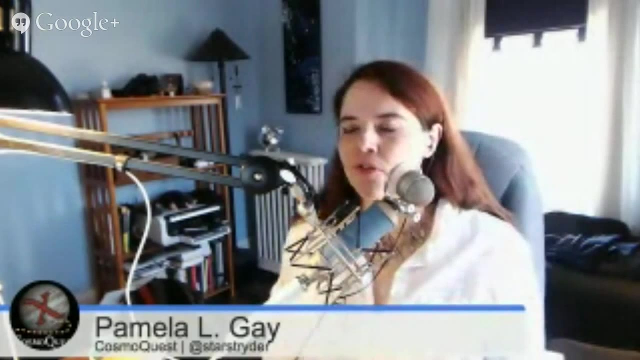 telescopes, Then we could. Yeah, it's. unfortunately I don't think you can fit one in a can set, just because the detectors- x-ray light does not want to be gathered and focused, and so you have to use a very careful scattering. 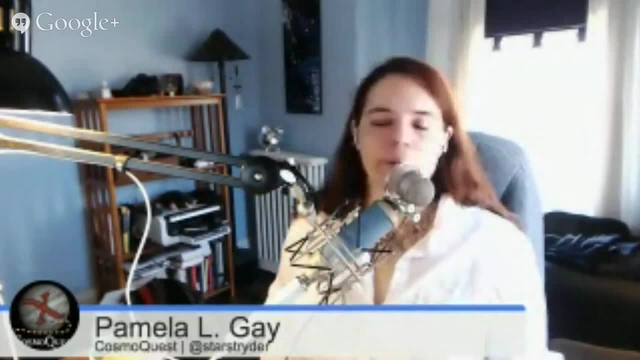 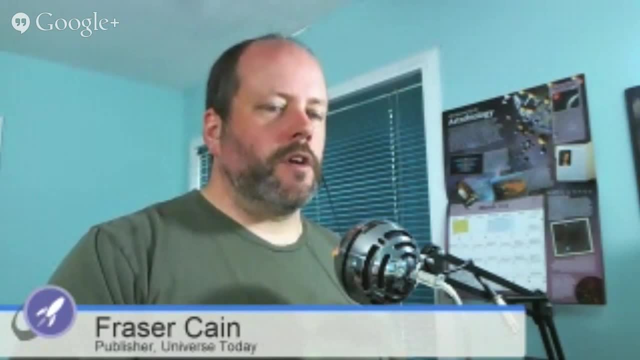 set up and then you have to have a shadow set up. Read about it. it's beyond the scope of a quick discussion. Nancy Graziano says you can see Cosmos on Hulu free or Fox or YouTube. Okay, haven't got there yet. 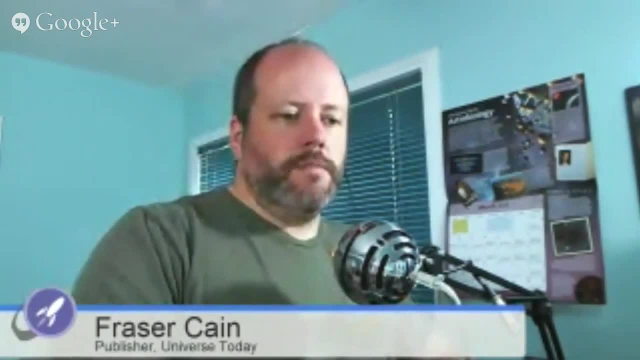 All right, neither have I. I will watch Cosmos shortly And you're in Canada, so you can't use Hulu. No, No, No, No. Nancy also notes: I don't believe you're not athletic, You're an equestrian, which is true. 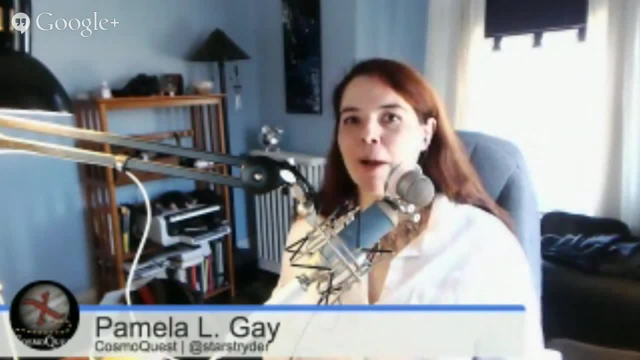 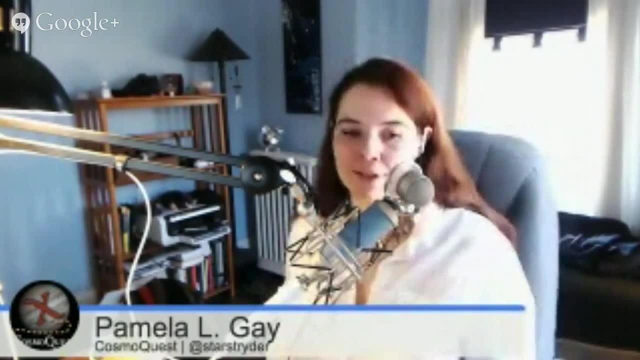 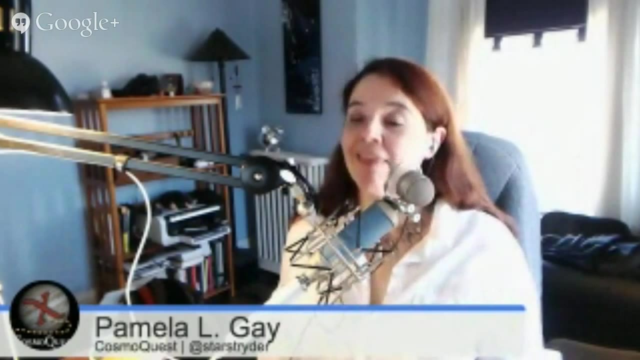 I, okay. so there's the difference between, by sheer force of will, tenacity and practice, being able to jump my horse over something that is all of 12 inches tall and not challenging to a dog, And actually having athletic skill. I, I, I lack the skill and have much practice. 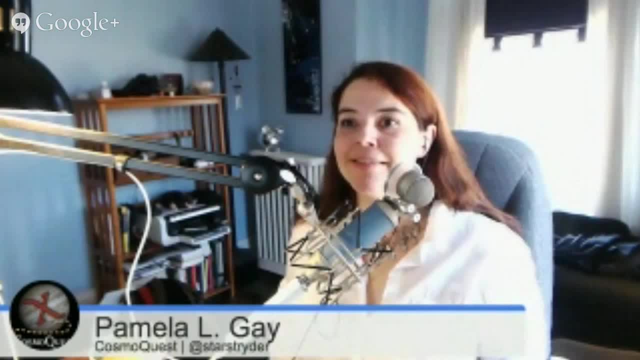 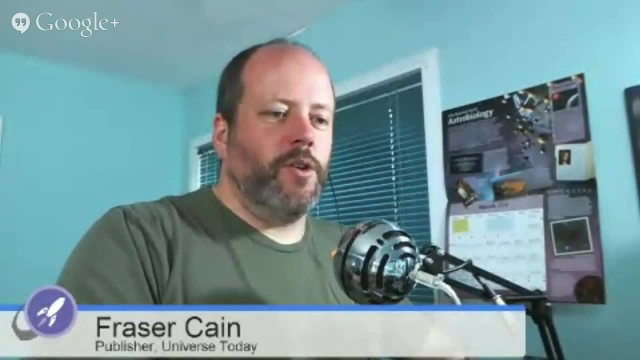 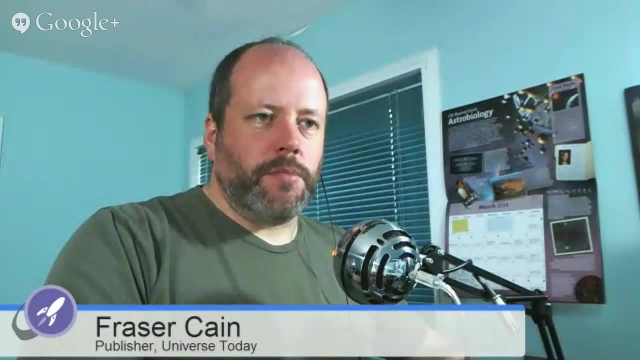 The horse is doing the jumping, I'm staying on. that's surprisingly difficult, I know, I know. I know riding a horse is just the worst. It's so hard. It like ruins my body when I ride a horse. Okay, I think this will be the last question, but I love it. 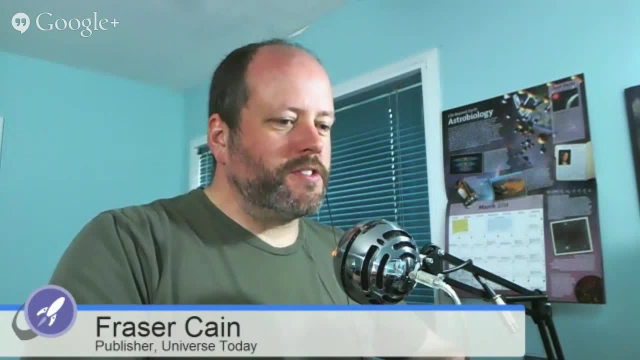 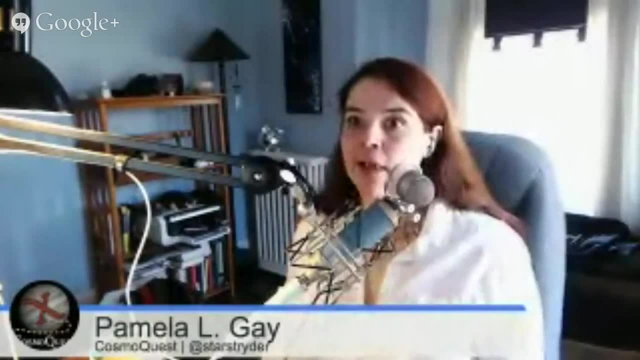 Pamela, can you give a quick explanation of your current research, Of my current research? Right now? I'm doing two different things. I'm working on statistical analysis to understand how well citizen science is and. I'm doing two different things. I'm working on statistical analysis to understand how well citizen science is, and. 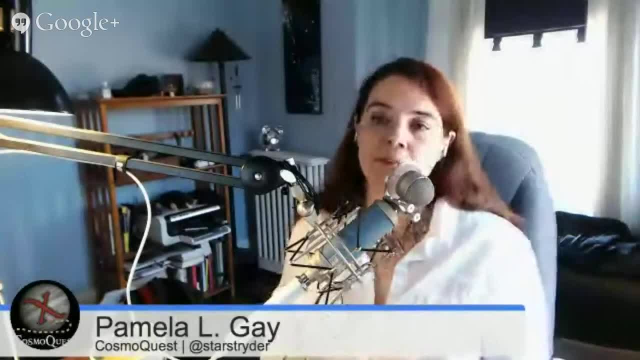 I'm doing two different things. I'm working on statistical analysis to understand how well citizen science is, and part of that is approximately 10 points of scientific results in different countries. Part of that is approximately 10 points of scientific results in different countries. 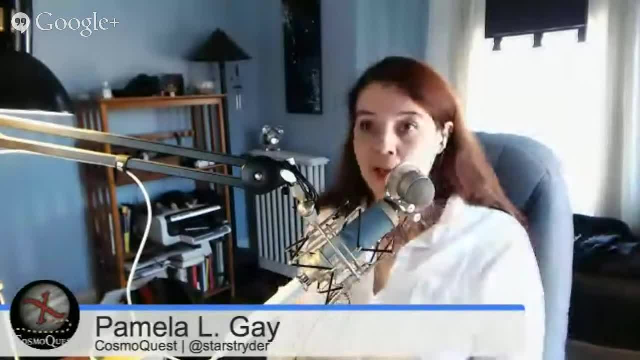 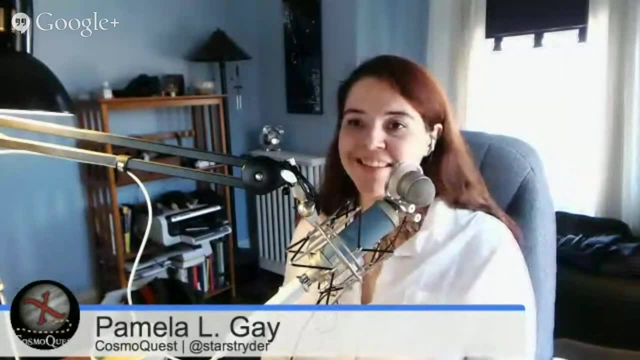 So how often can I get to do things that are really good and remarkable And then the other way to do this is adding a fashion- retroactive research to stimulated incremental health change? hi In the In the. In the picture there is a picture of Helen. 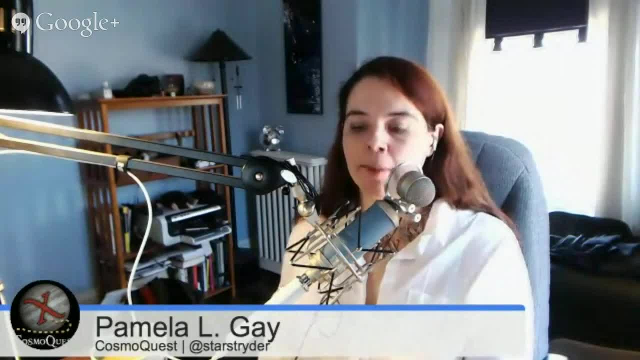 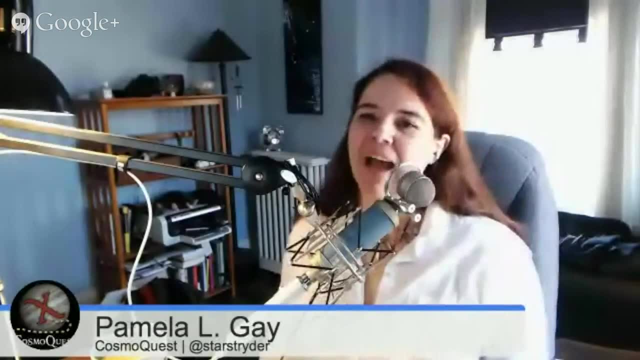 speaking, and I think that the there's a lot of us who are being interested in looking for a doctor. To make it obvious for a film, we need to make sure that authors provide results: deep, depth and deep get information working. I started college as a sociology major. I just switched a few times, But seriously. 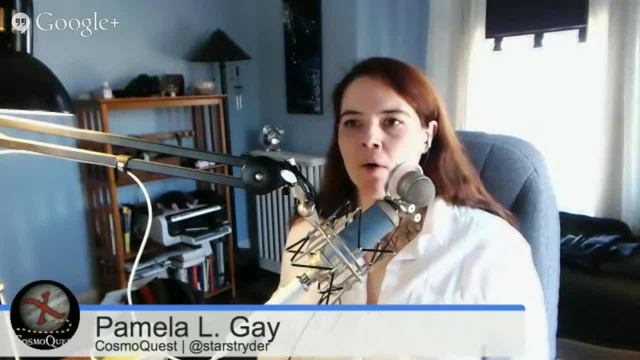 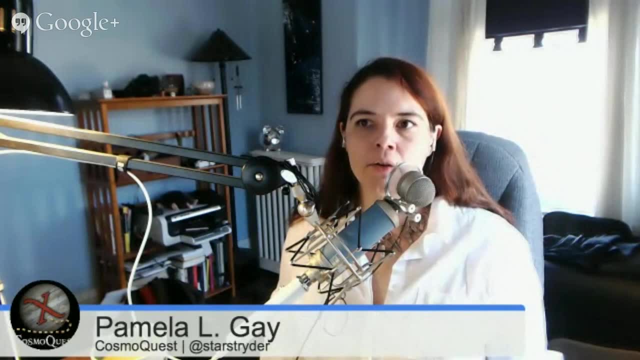 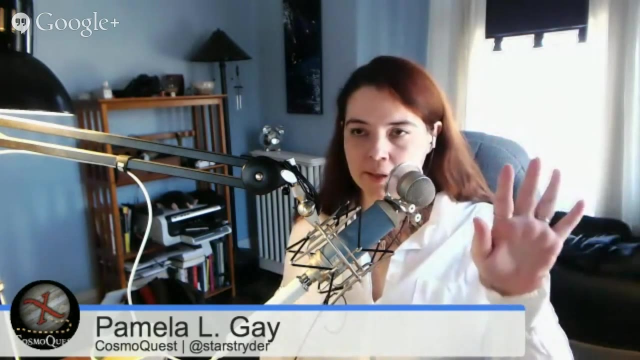 so part of my statistical brainpower and computational ability to do stuff is going into doing large scale surveys of trying to understand what factors cause people to want to participate in citizen science. So there's all of the comparing. I've started to become a computational. 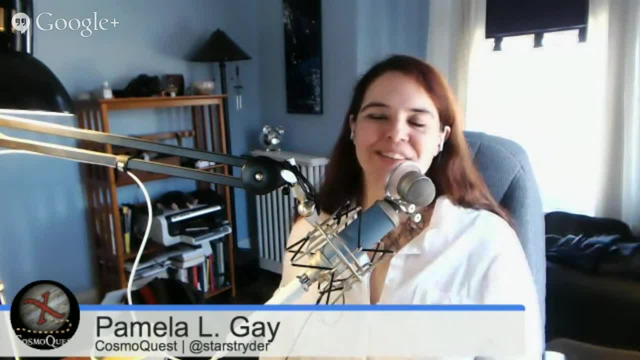 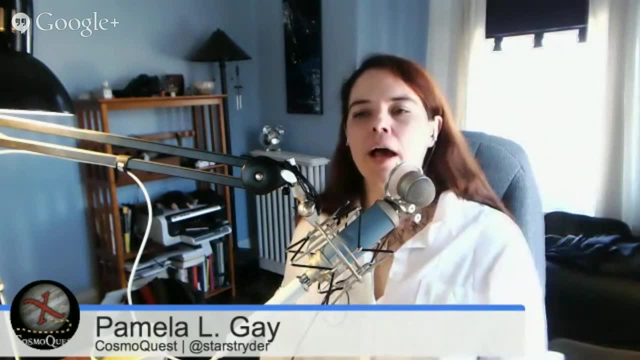 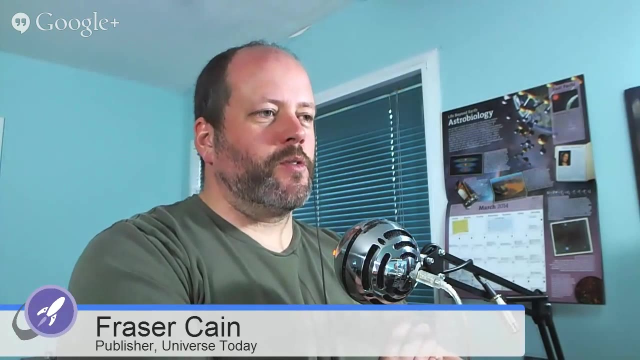 person against my will. So there's all the computational work to try and make sure that moon mappers, all of our different projects at CosmoQuest, are producing legitimate science. And then there's understanding why people do this. I think it's hilarious how I'm the one with the computer science degree. you're the one. 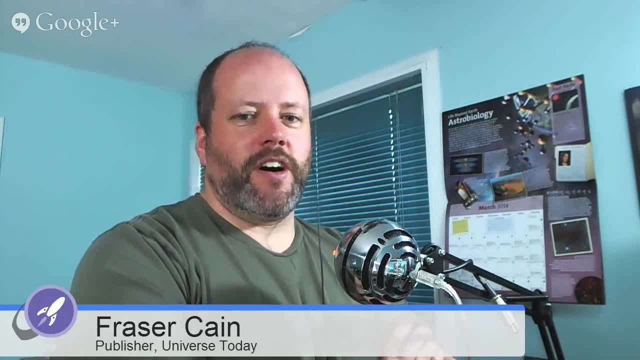 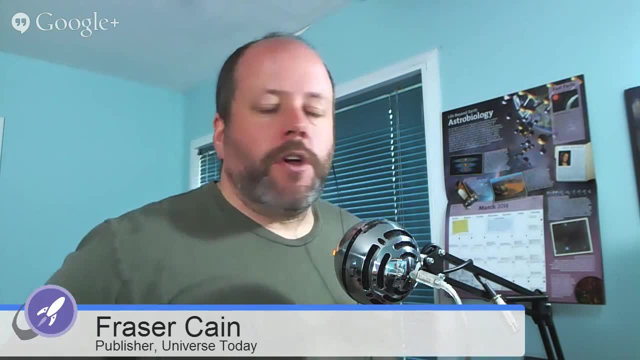 with the astronomy degree, and you're often doing this Doing more computer science than I do, So you know what? before we go, I think we should wrap this up, But before we go we should make a push on Cosmo Academy, because I know we've got a bunch of courses coming. 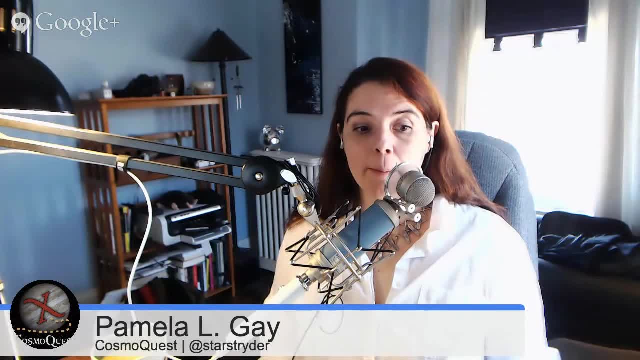 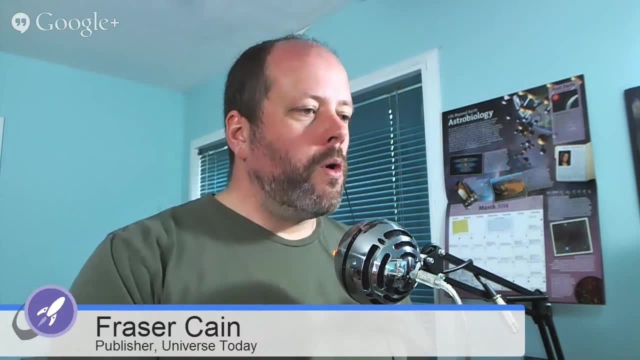 up shortly, right? Yes, Yes, there's a whole bunch of classes coming up. I have not made it that far through recovery. I have no memory of the month of February. Nicole is doing a show on astrobiology. Dr Matthew Francis is doing a show on- I forget. 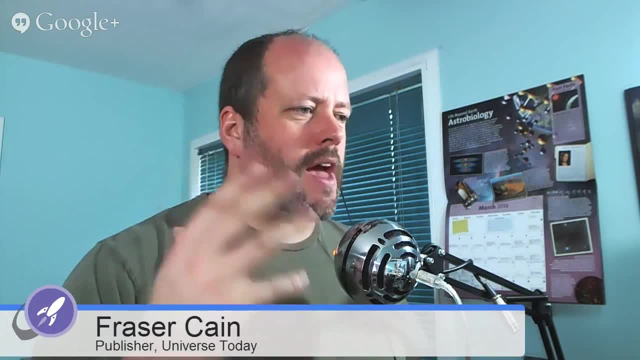 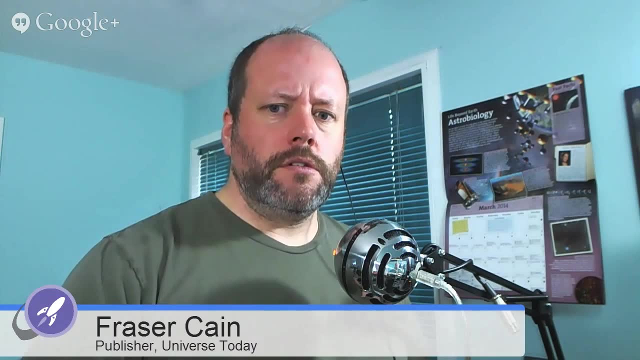 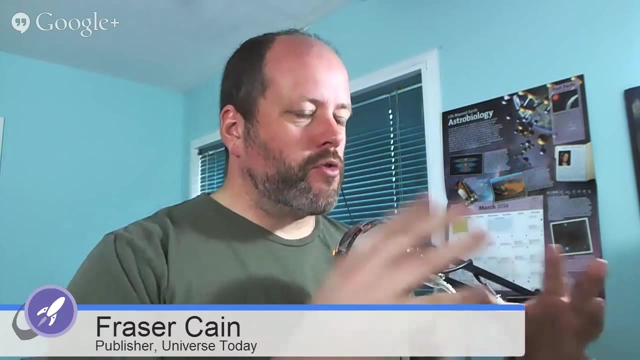 but it was really cool. Cosmology, black holes, dark and mirror, Yeah, the big cosmology type stuff. And then there's another one on, I think, planetary geology. Anyway, here's the deal: We are building a crew of working PhD astronomers who really 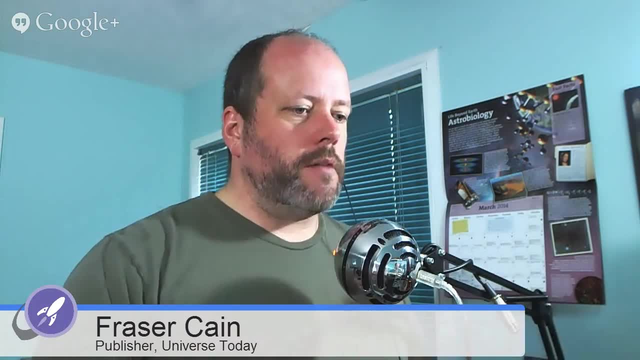 know this stuff and you can sit and there's like eight people in a class. You get really personal treatment and they will teach you over the course of multiple weeks, seven days, and then you can sit and watch this show. And then you can sit and watch this show And 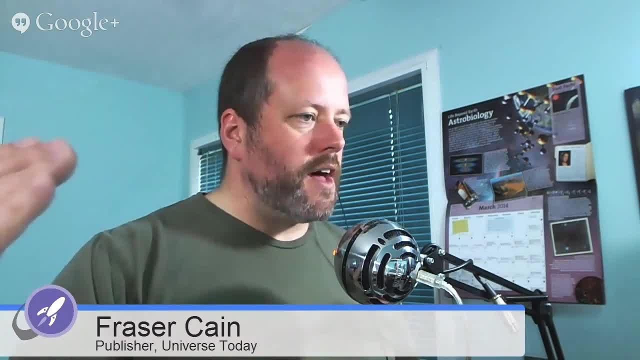 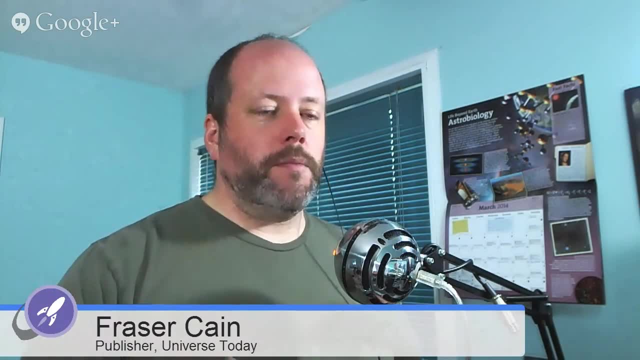 you can sit and watch this show, And then you can sit and watch this show, And then you can multiple weeks a subject matter that is at the next level. This is an enormous opportunity. It's not free- No, it's not free, But if you've got some money and you want to take your knowledge, 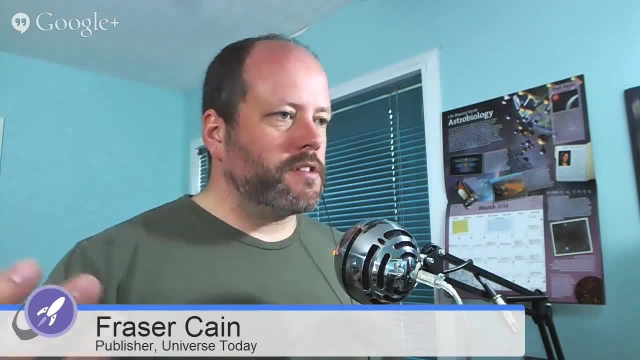 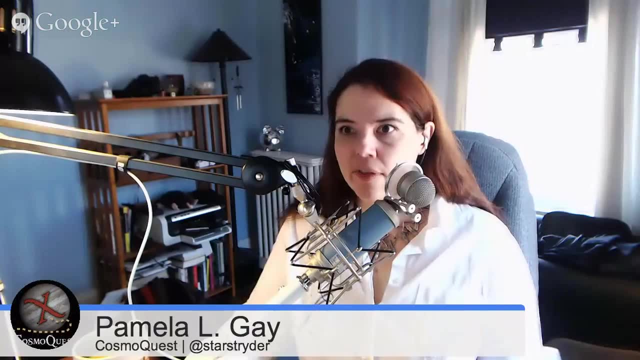 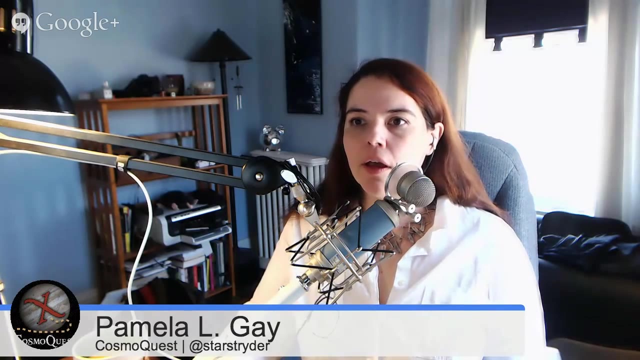 to the next level. Pamela sometimes does some of these courses. This is something that people have been asking us for. Yeah, People have been asking us: how can we learn more from you people? This is how. This is how We priced it, based on how much I pay for equestrian riding lessons. I was trying to 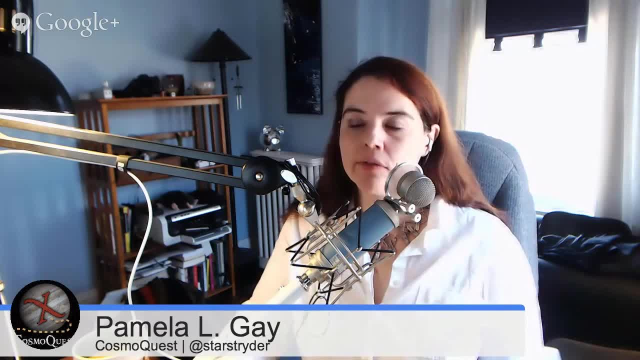 figure out. what does a hobbyist training thing cost? Almost all the money goes to the instructors who are taking the time to prepare the lectures, to show up, to prepare assignments. We're working to build this up. I'm sorry that I don't know more. I literally have almost no.